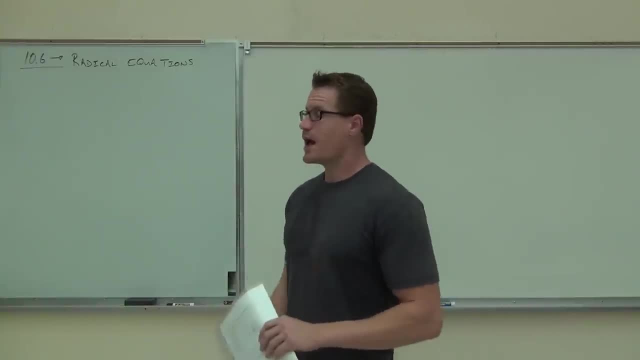 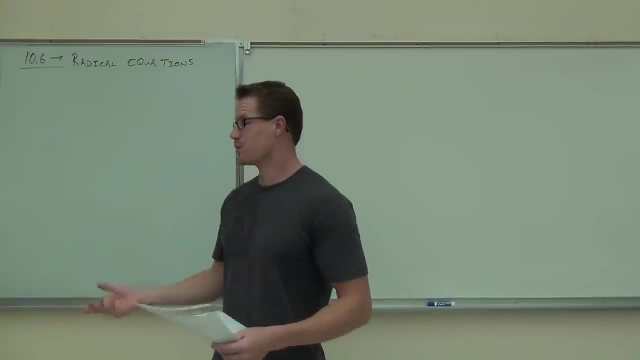 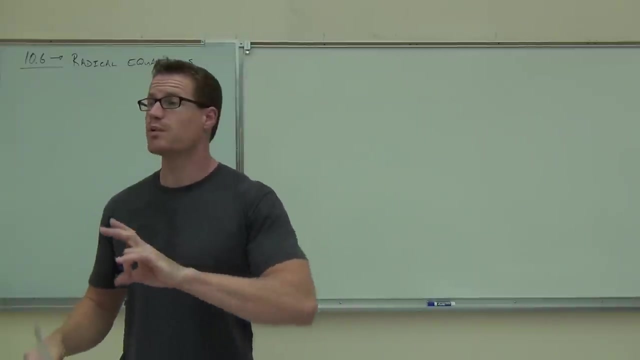 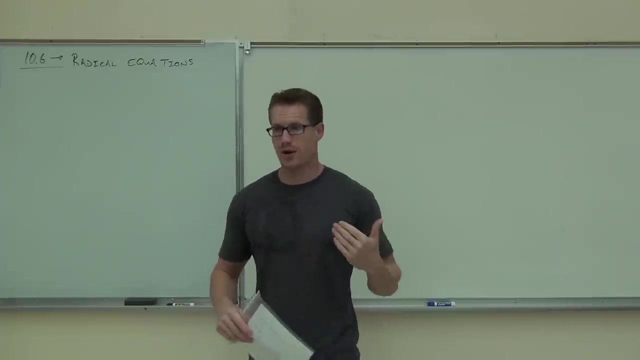 So we're talking about section 10.6 and we're going to talk about radical equations. You see, we really haven't talked about equations thus far. We've only talked about how to simplify and manipulate our roots. Right now we're going to talk about equations and those have the equal sign in them. Now there's one cool thing that's very similar to fractions: what we can do with these radical equations. If you remember about fractions, we could not actually get rid of fractions unless we had an equation. That's because we had fractions on both sides. we could multiply both sides. 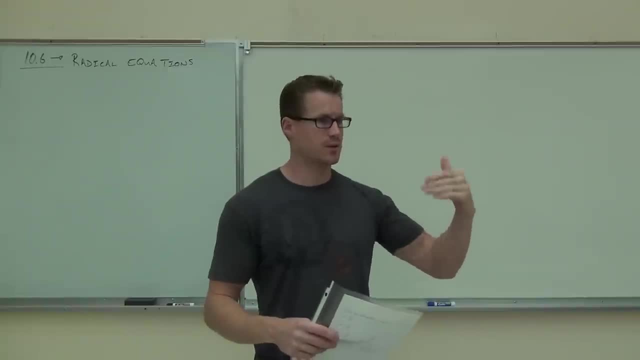 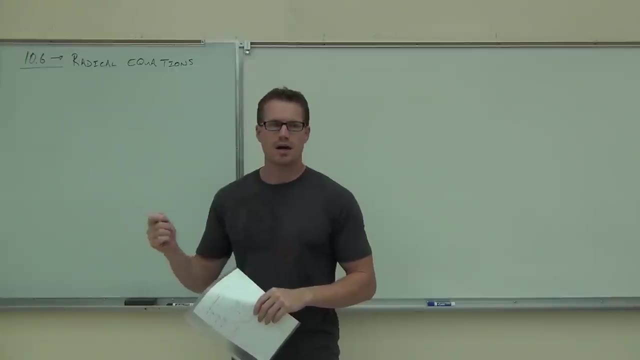 We could multiply both sides by the same value and then that made it equal. That was able to get rid of our denominators. We have something very similar, something very similar with these radicals: If we have an equation, we can raise both sides of an equation to the same power and still equal, And that's the kind of statement we're going to live off in this whole section right here. It's just one statement. It's the only thing that we're really learning today. So, if you guys aren't even with me right now, It's the only statement we can live off today that we're going to learn is that we can raise both sides of an equation. 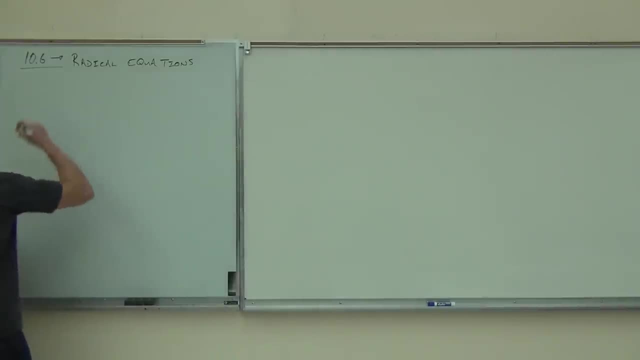 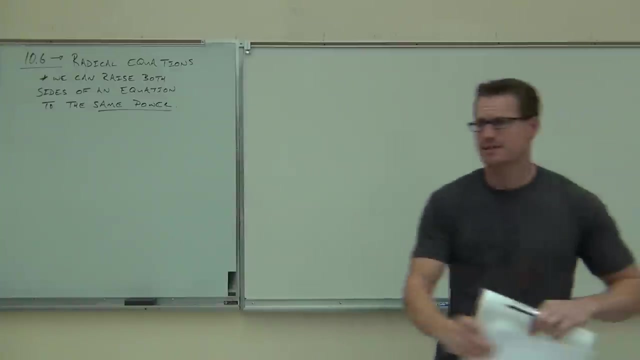 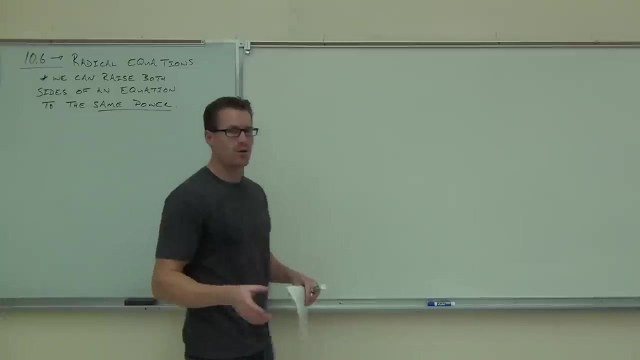 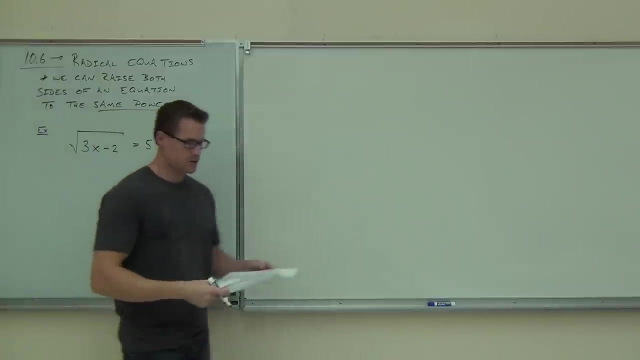 to the same power. That's it. So not only can we add something to both sides, subtract something to both sides, multiply, divide on both sides of an equation. we can now take both sides of an equation to the same power. I think I previewed this for you last time, but let's look at an example like this one: If we have the square root of 3x minus 2 equals 5, we can raise both sides of an equation to the same power. That's it. 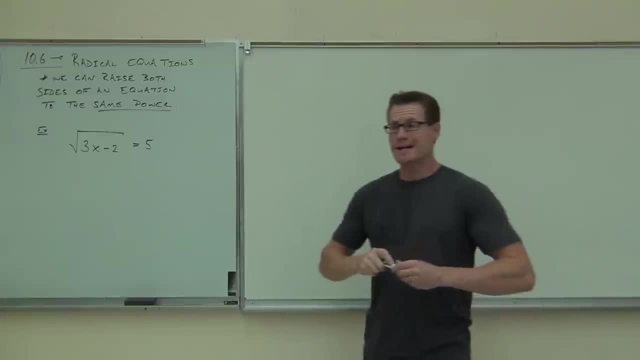 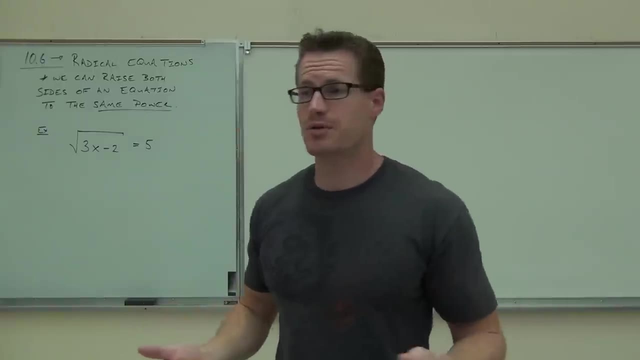 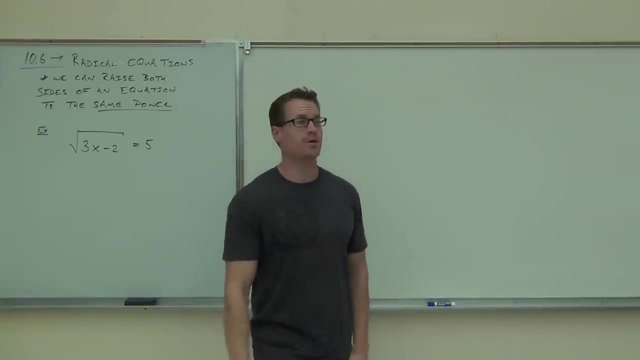 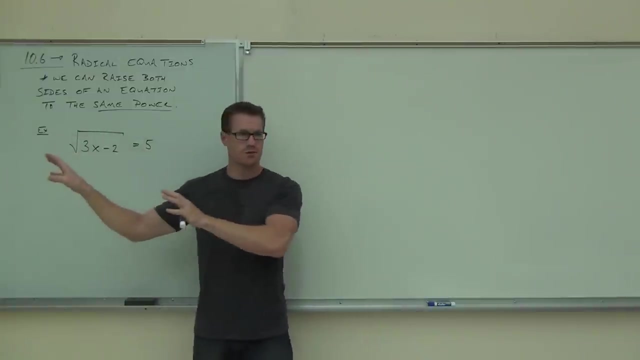 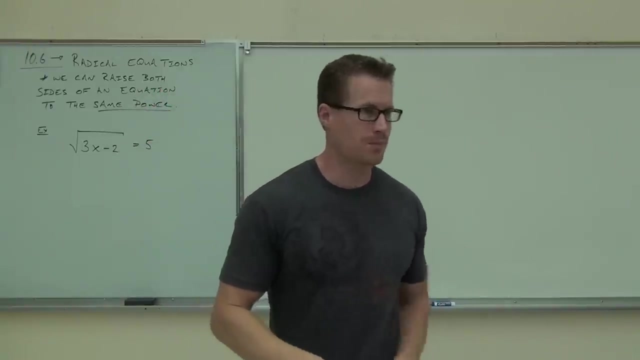 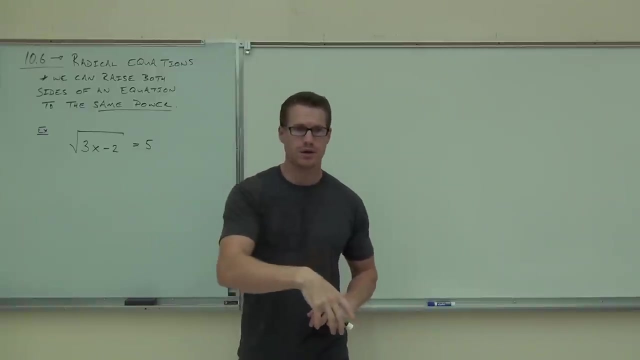 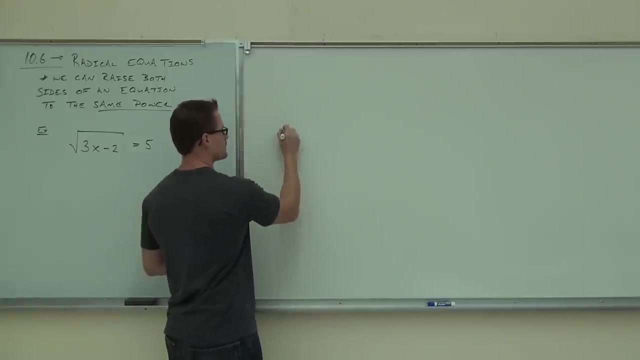 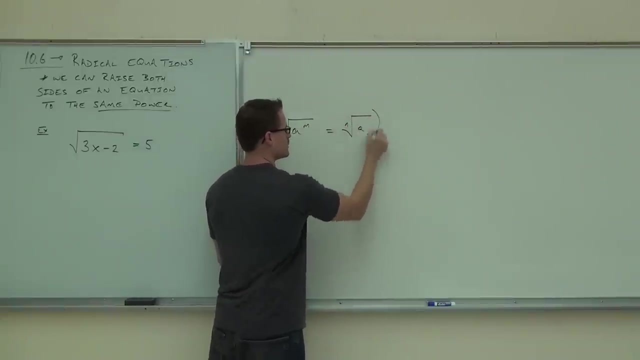 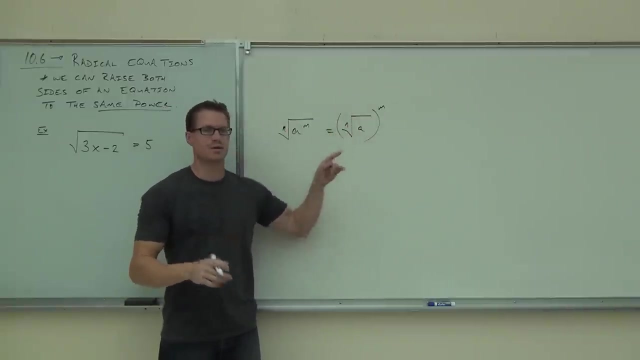 So let's look at an example like this one. If we have the square root of 3x minus 2 equals 5, we can raise both sides of an equation to the same power. That's it. So let's look at an example like this one: If we have the square root of 3x minus 2 equals 5, we can raise both sides of an equation to the same power. That's it. 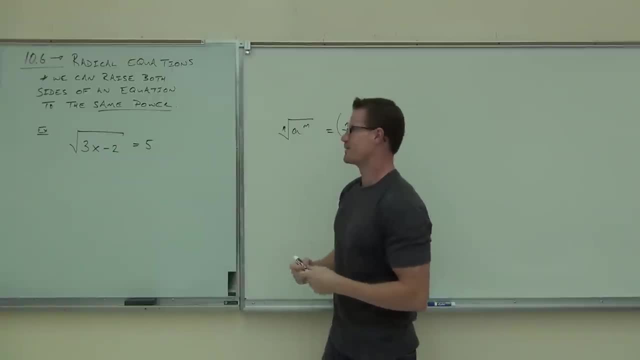 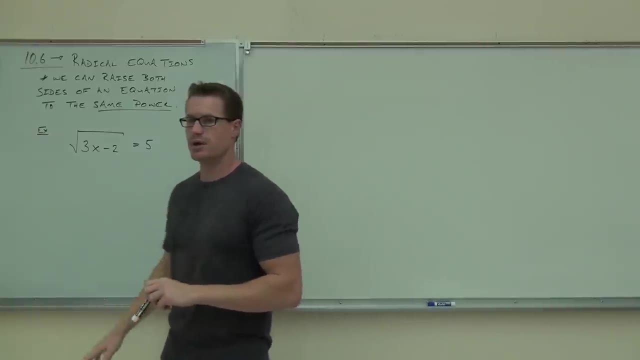 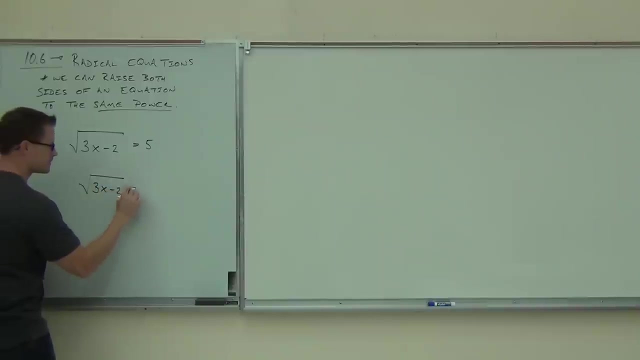 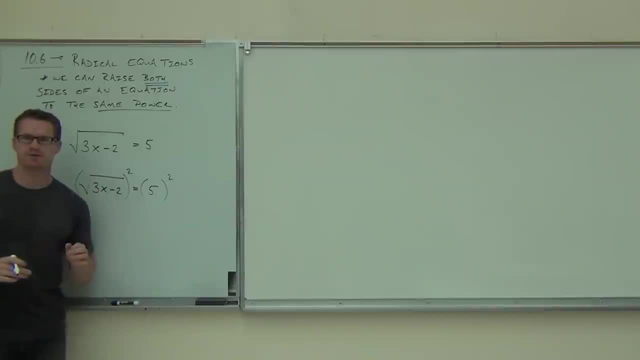 So tell me what's going to happen on the left-hand side of my equation, The square root of 3x minus 2 squared. What happens to the square root and the square? Well, that's great. What do we have left then? 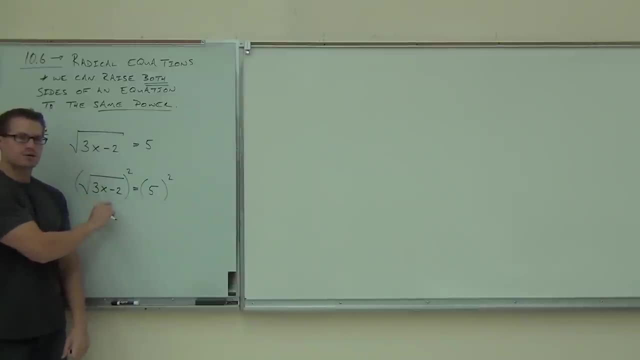 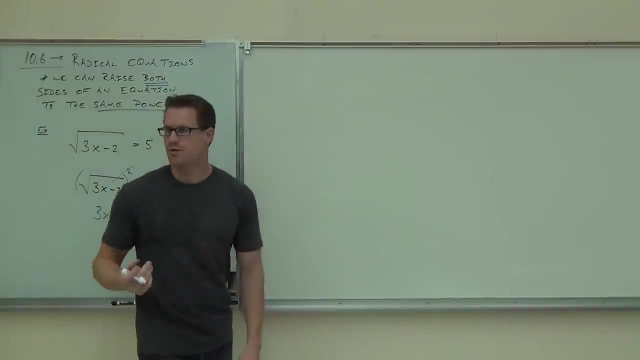 Okay, Do I have to square this inside part? No, Do I have to do anything with that? No, So as soon as I do that, that's all that operation is doing. That's kind of nice, I mean really. we're just left with 3x minus 2 equals. Well, we can square 5.. That's pretty easy. We're going to get 25 on that side. 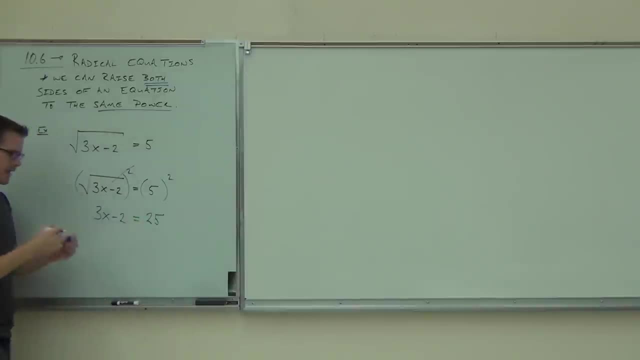 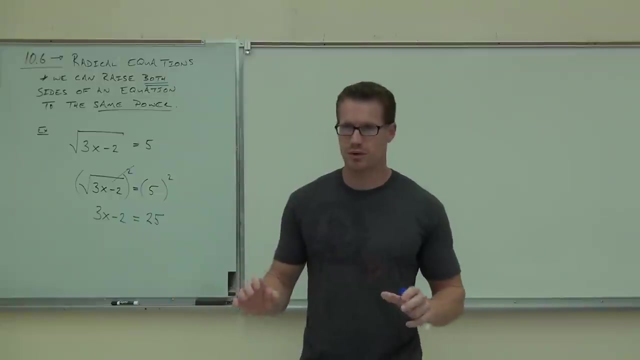 Okay, After that we have something that is very, very simple to solve, something we've seen in this class time and time again, and that's how this process is going to work: We square or cube or fourth- both sides of an equation, depending on what type of root we have. After that, we'll have something simpler to solve with no roots. 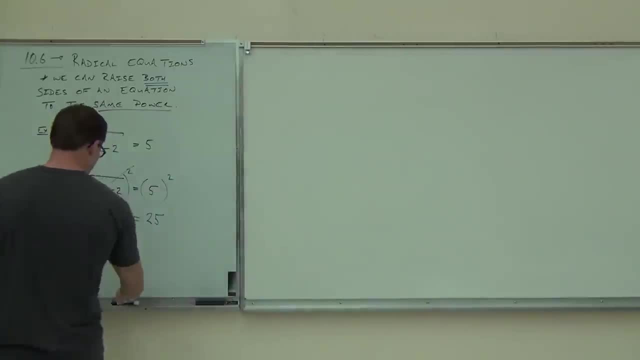 Are you with me? We can solve this one. I'm not going to patronize you by asking you about it. We're going to add 2 here. We'll get 3x equals 26.. Okay, We've got 27.. Of course, our last step is divide by 3.. We've done this a lot. That's why we're in this class, because we do things like this. 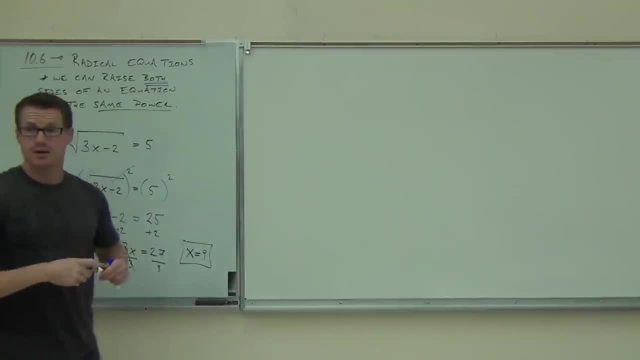 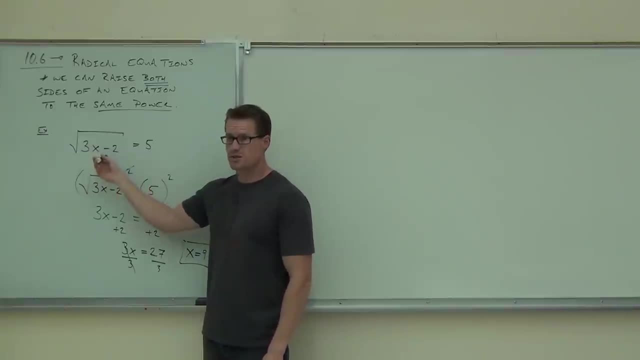 And we've got x equals 9.. By the way, could you check your work? Sure, If you want to plug it into your original one, 3 times 9 is minus 2 square root. We got it. That's the right answer. Raise your hand if you're okay with it so far. 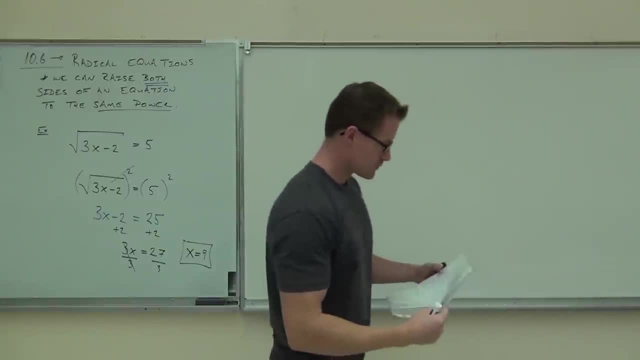 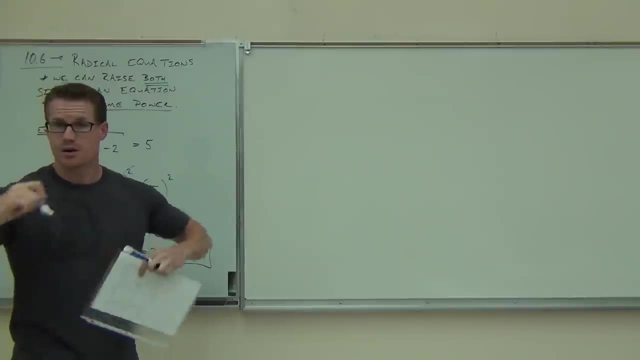 All right, Good, Let's try one on your own real quick, just to make sure you get the hang of this. Go through the process once. It'll be very similar, not a real hard thing. You just have to kind of remember what to do, right? That's the whole idea in this chapter. 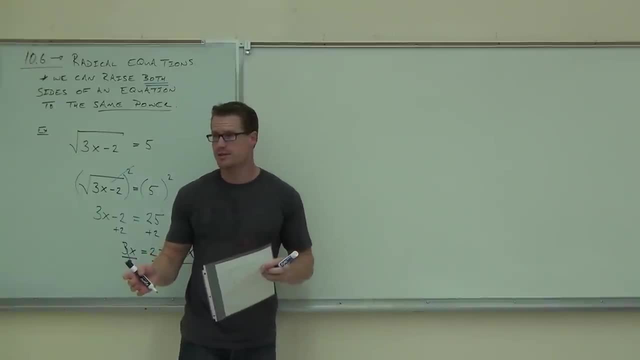 The math isn't too hard. It's not like chapter 7, where you were doing all sorts of crazy stuff, right? This is not that many steps. to be honest with you, It's not that hard. You just have to remember what you can do, what you can't do. That's the whole idea. 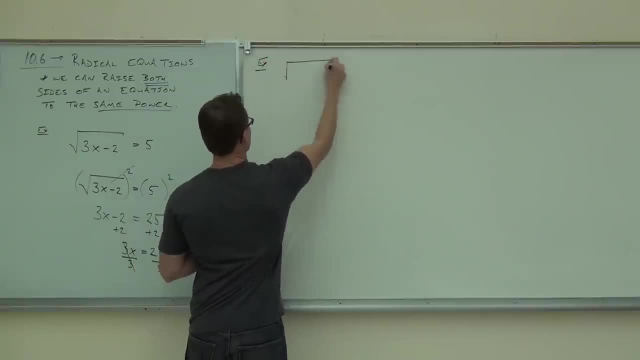 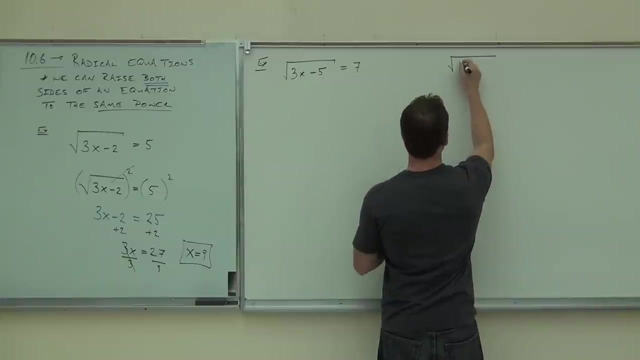 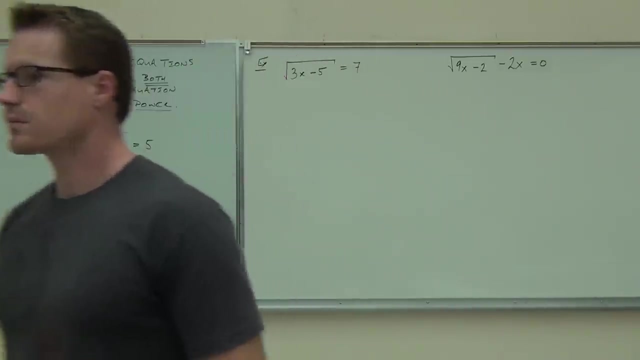 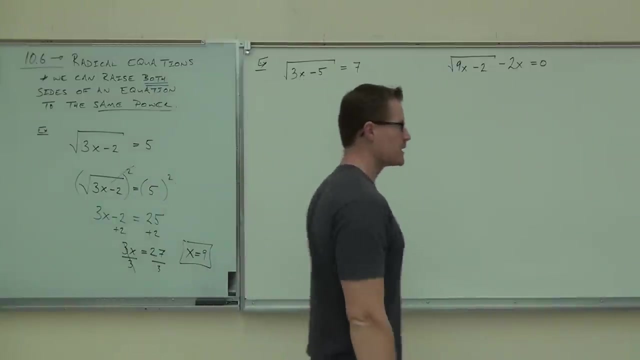 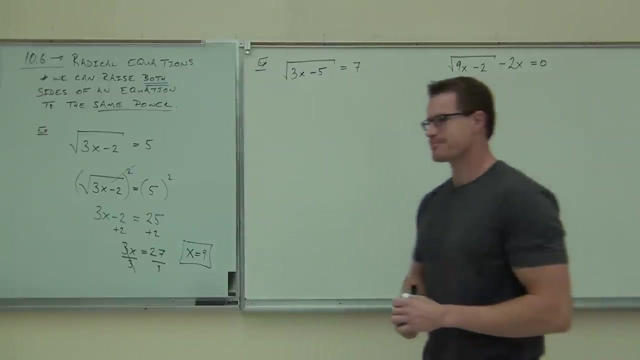 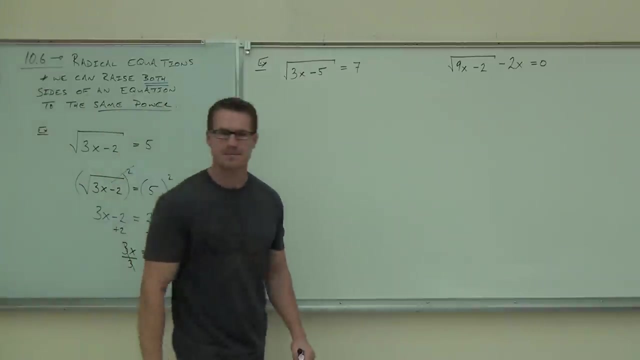 There you go, There you go. So the way we get rid of a radical is to look at the type of radical we have, Look at that type of root, And we can raise both sides of the equation to that same power. Hey, what power is going to get rid of that root? 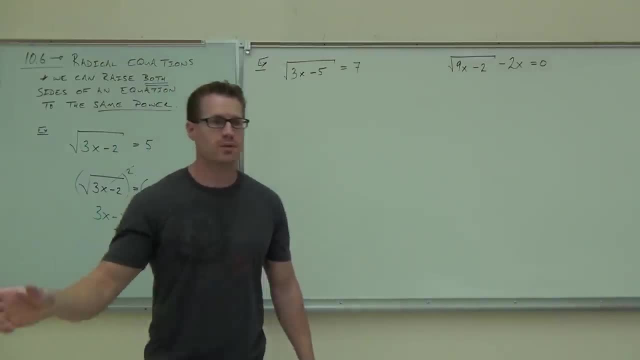 Two. So we're going to look at the type of root we have. the square root, A square power, is going to get rid of that. One thing you've got to be careful of: make sure we're not just doing this to one side. 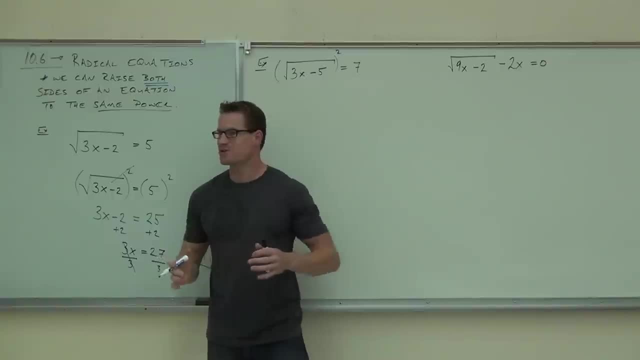 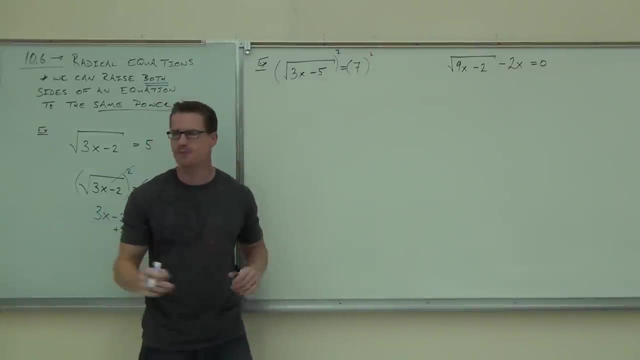 If you do it to just one side, you're going to be way, way, way off right, Because you'd have 7 instead of what we should have, which is 49.. So we're going to square both sides. That's legal, Taking both sides of the same power. that's fine. 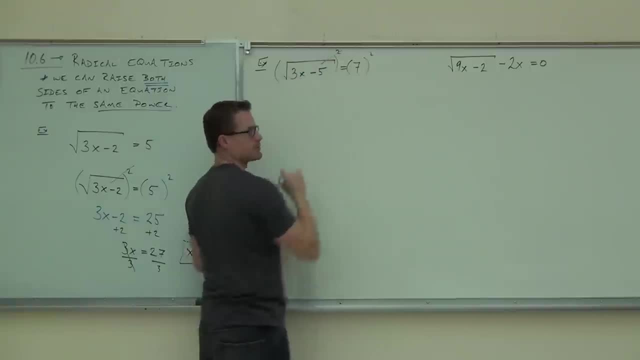 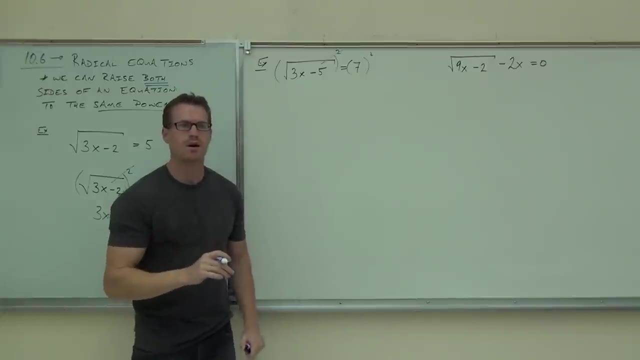 What happens over here is that the square is going to undo the inverse operations, undo that square root. By the way, do you want to see why this works? If you really want to know, Here's why this works. I'm going to do a very simple example to show you why. 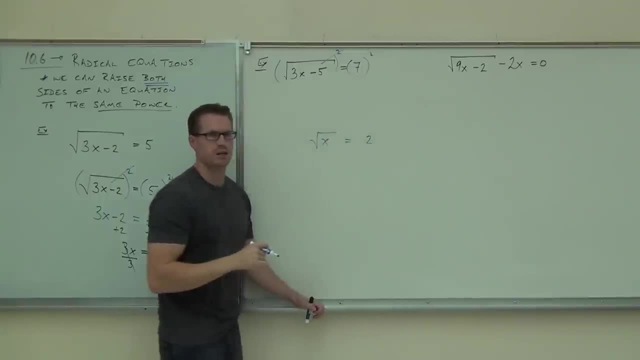 Let's say you had the square root of x equals 2.. A very simple example. Watch on the board here real quick. You don't have to write this down. just watch The square root of x. I would square both sides of that, right. That's what I'm telling you. 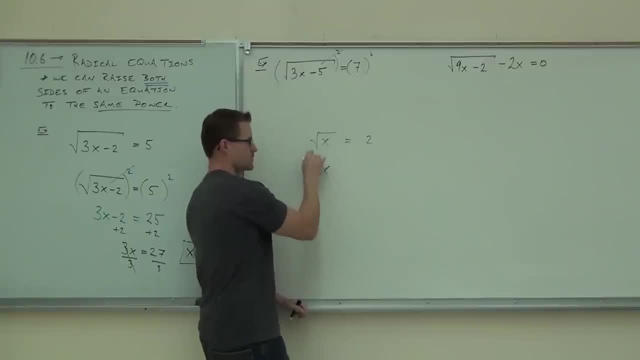 Why that works is because x- sorry, the square root of x- could actually be written as x to the 1 half power. Is that true If you square both sides here? what do you do when you take an exponent raised to an exponent? 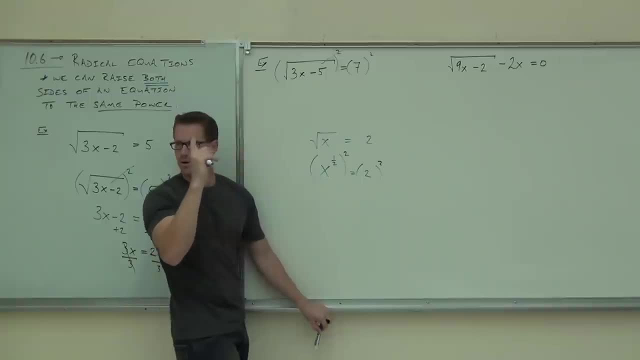 What's 1 half times 2? 1. You get 1. You get x to the 1st. So this would actually give you x. That's why that works. That's why we can square a square root and it actually works out for us. 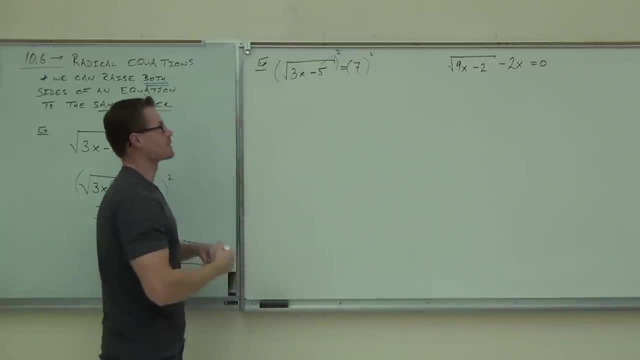 Okay, anyway, a little above and beyond for you. Hopefully you caught on to that. So here we know, a square root and a square. they're going to simplify, We're going to get 3x minus 5.. You don't change that at all. 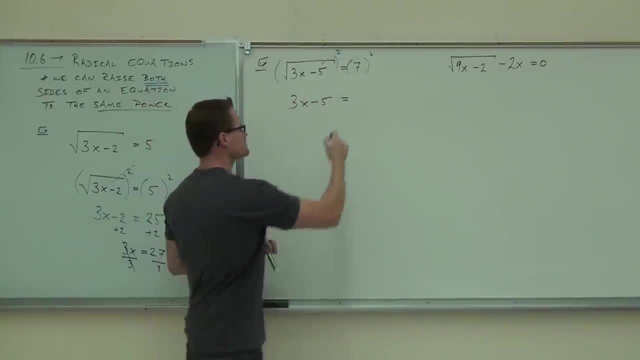 You just have to remember to square the right side as well. We're going to get 49.. After that, we'll solve it. We all know how to solve these things. We're going to add 5 to both sides. We'll get 3x. 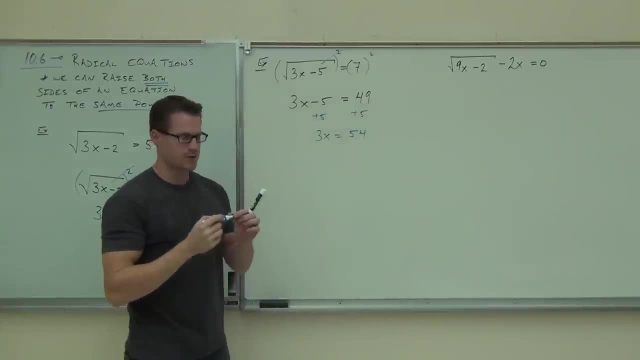 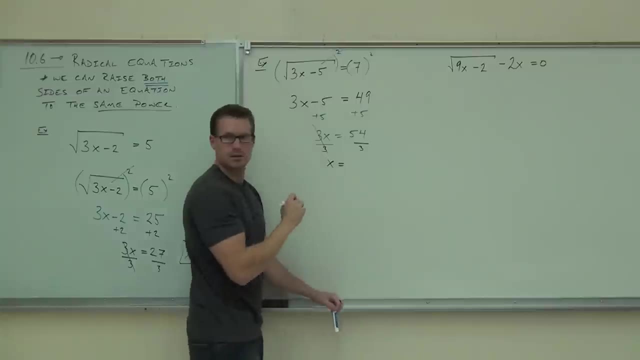 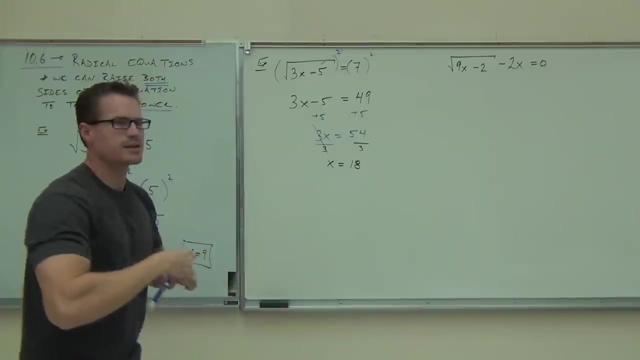 What is that? 54?? And if we divide by 3,, how much is it 18.. Would you raise your hand if you got 18?? Cool, All right, Let's try the next one. Let's try the next one. 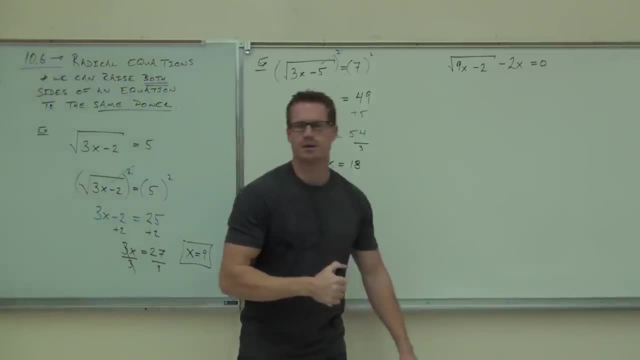 What type of root do we have? Square root, Okay, cool, Definitely a square root. So we'd square both sides here, right? Wait a second, Wait, wait, What do you mean? not yet, Oh, Does it look like these ones? 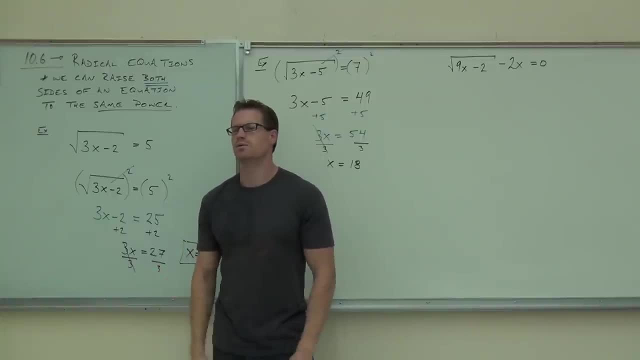 No, These ones were different than that one. These ones, it was: square root equals something right. Square root equals something That was great. Do you remember the absolute values that we did in Chapter 9?? And how, when you did your absolute value, you actually had to get it by itself first? 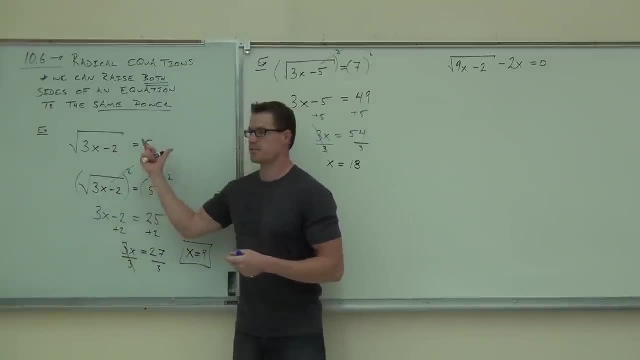 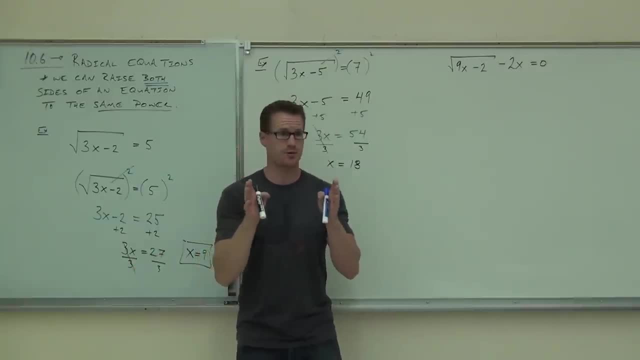 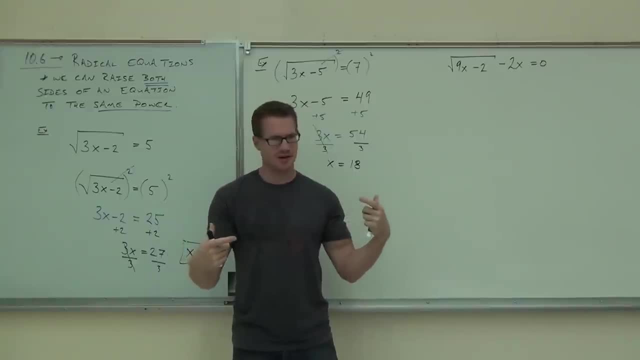 Yeah, So we'd isolate that and then we'd make our two equations. Some people in one of the tests forgot those two equations, but you know, whatever, Whatever, We would normally isolate those things before you do any work with it. 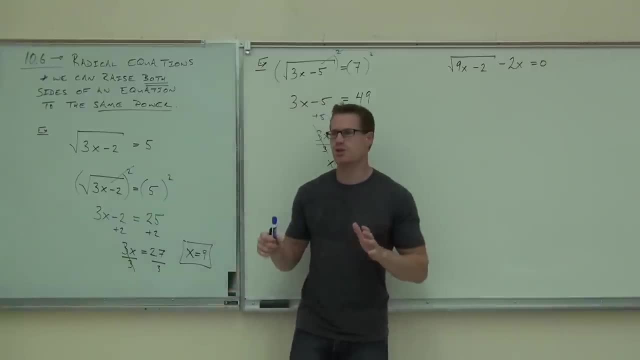 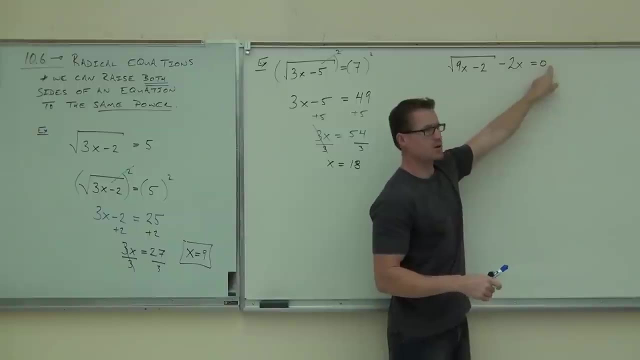 That's the same idea here. If you try to square both sides- I want you to notice this- You could do it, It's legal, You could do it. But if you squared both sides here, sure, the square of zero is still zero. 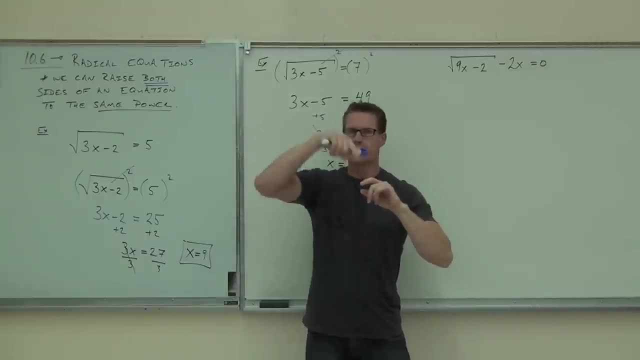 But over here, notice, you have a FOIL problem. You have to write that out. You would have four terms. Two of them have a square root. That would be ridiculous. You really don't want to deal with that, do you? 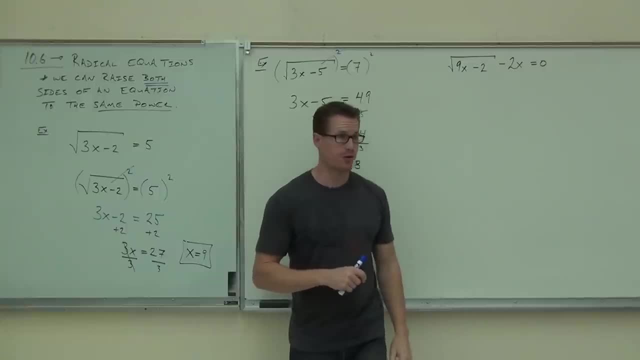 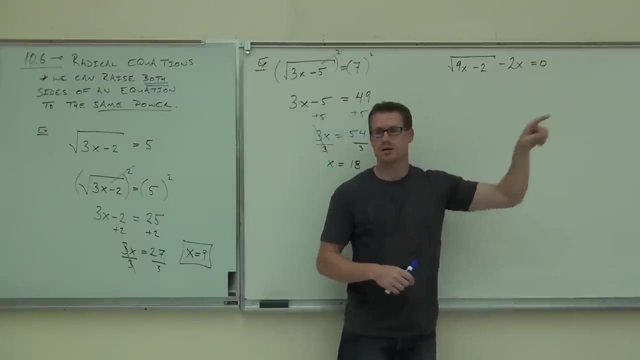 No, No, We're going to isolate the square root first. That way, when we square this side, we get something reasonable. When we square the other side, we don't get the square root anymore. That's what we want to do. 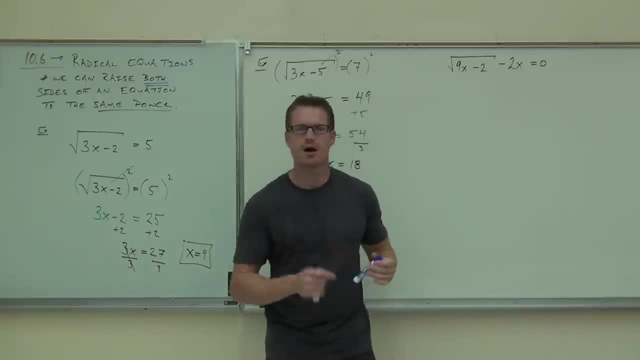 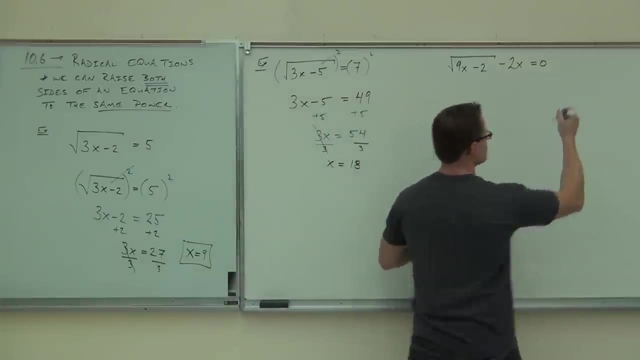 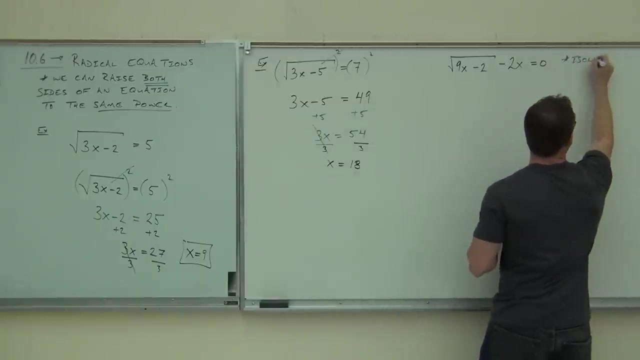 So, before you square both sides, please listen to this, Please write this on your paper: Isolate your square root first. Absolute necessity, Absolutely Unless you want to spend a whole long time on these problems which you don't Isolate the root first. 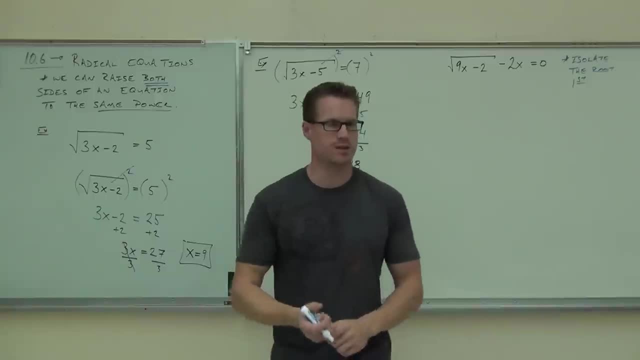 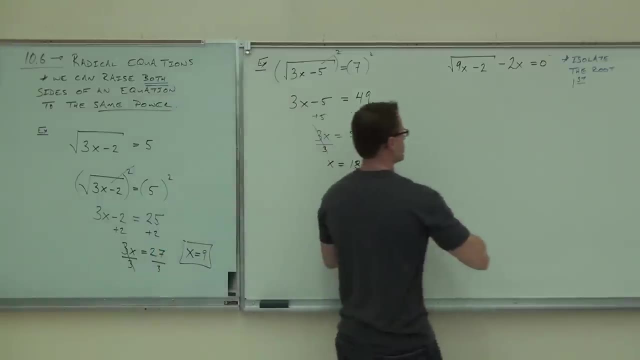 Whatever root you have, Not just a square root. Whatever root you have, you're going to isolate that. So tell me, how am I going to isolate this root? What would I do? Okay, Perfect. Now, of course, you would mean to both sides. 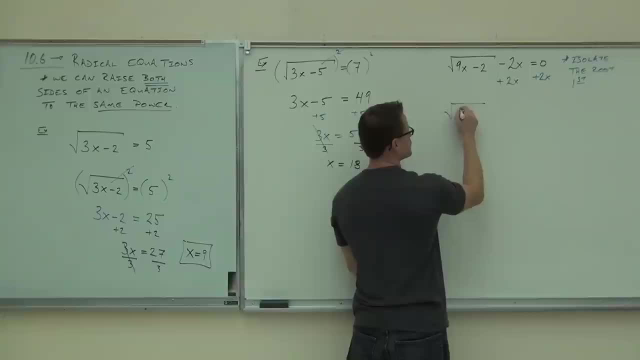 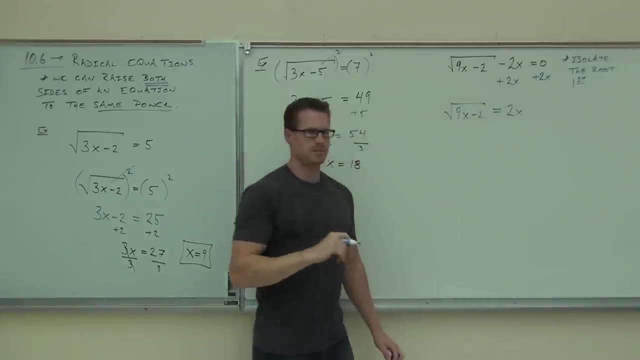 On the left-hand side, I'm left with a square root of 9x minus 2.. On the right-hand side, I'm left with 2x. Keep a little head nod if you're with me. so far, Okay, Is my square root isolated? 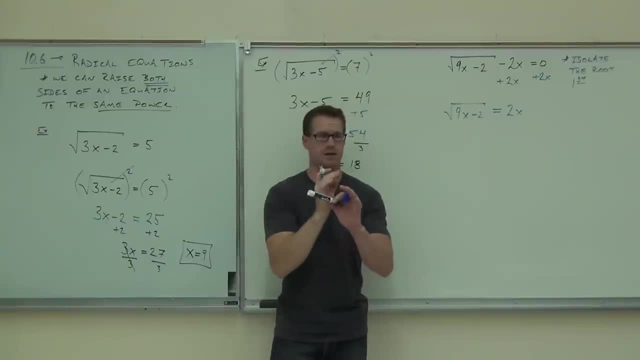 Yes, No. It's all by itself, then, an equal sign. We got that. Yes. What power is going to get rid of our square root, Square root? Okay, Now watch what we're going to do here, Okay. 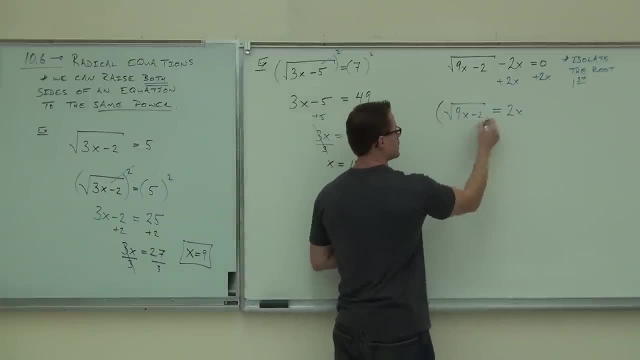 You've got to watch carefully. Sure, we are going to square. We are going to square left-hand side, No problem For sure, If we square the right-hand side. is that okay? No, What that means? right, there is 2x squared right. 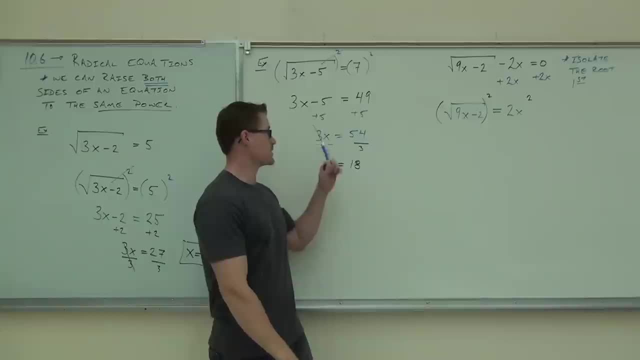 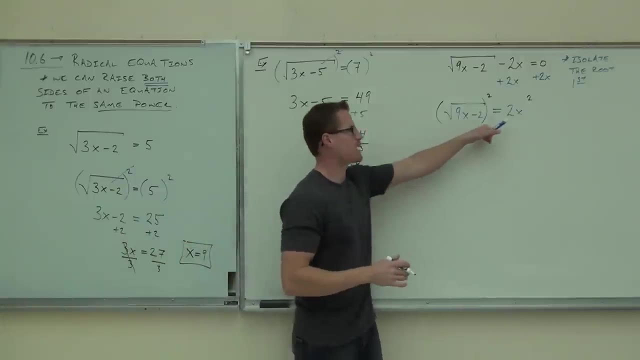 No, The reason why I had you do parentheses here, and the reason why I had you do parentheses here- even though it seemed like we probably didn't need it- is that if you're going to square this right-hand side, you are not going to get 2x squared of that. 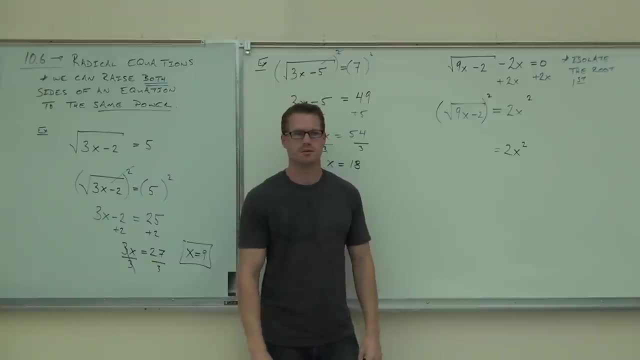 Why not? Because you're doing both the 2 and the x at the same time. I don't want to leave that 2 alone and just square the x. I want to square both those things. I want to square the entire side, right? 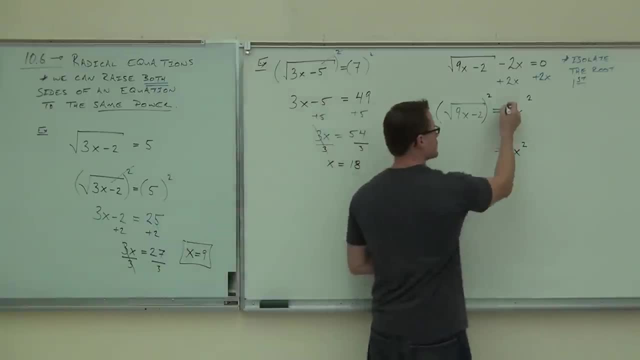 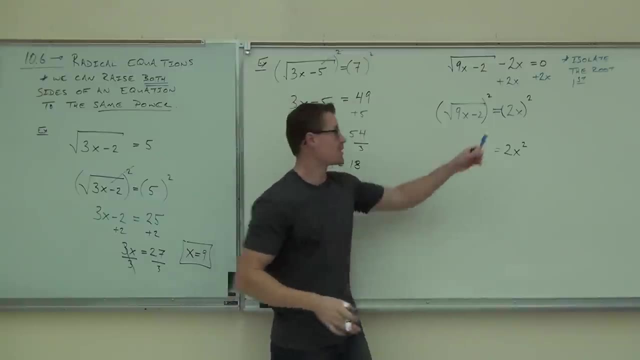 That's why we've been practicing the parentheses here. If I put the parentheses around it, well, that changes the problem. That says: not only am I squaring the x, I'm squaring everything in that. It's a product. One of those rules that we had for our exponents was that if you have a product inside the 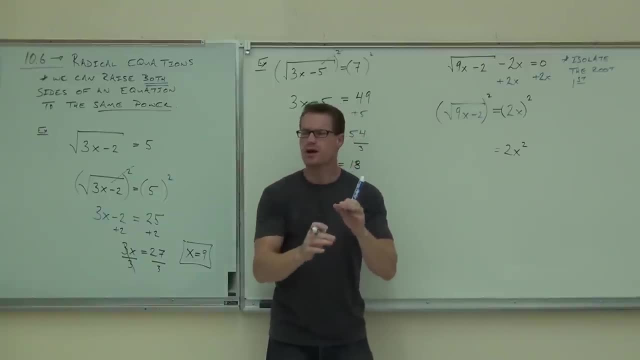 parentheses. you square not only the x, you also square the 2.. Think it's going to work. Think it's going to affect your problem if you forget to square that 2?? Yeah, probably You're going to get 2x squared instead of what we should get 4x squared. 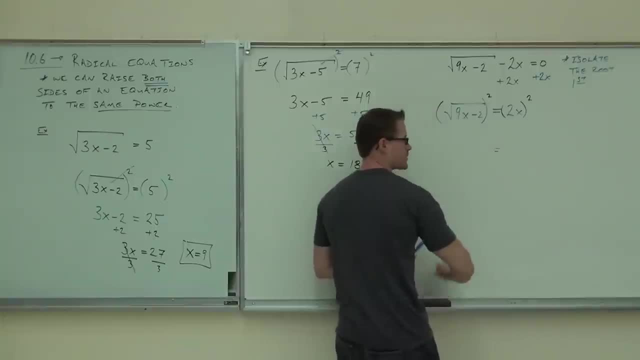 Here now. we're not going to get 2x squared. When we square the 2, we get 4.. Then, of course, we are going to get x squared. Don't forget that we have an x squared. You know what a lot of people do. 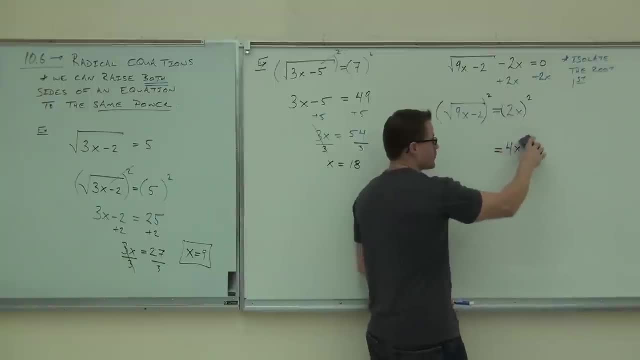 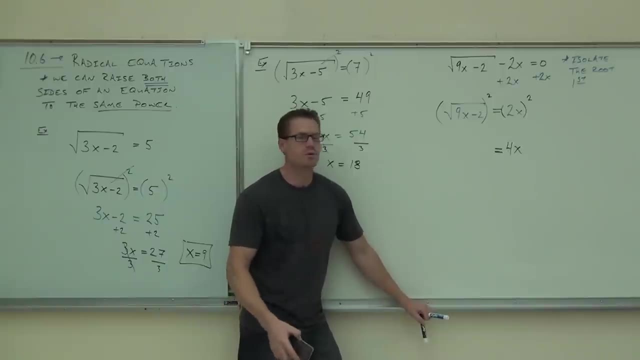 They're going quickly. They give me this. Maybe they do the 4. They give me that. Is that going to change your problem? Yeah, Yeah, that's a drastic change in our problem. right there, Be careful, Don't go too fast. 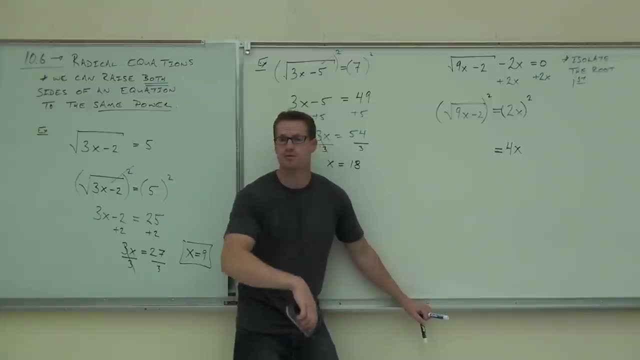 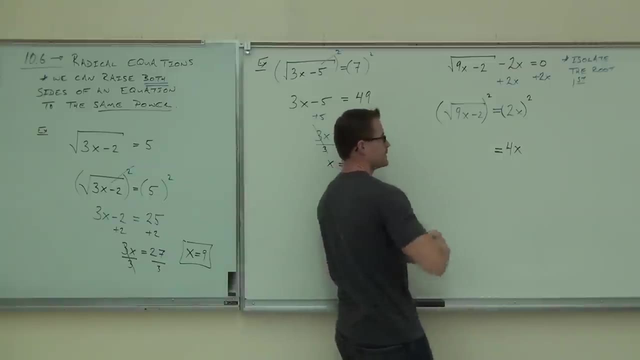 Again, the math here isn't going to be that hard. It's all stuff we've done before. It's just kind of noticing the small things, knowing what you can do for any given problem. So here for sure we're going to get 4.. 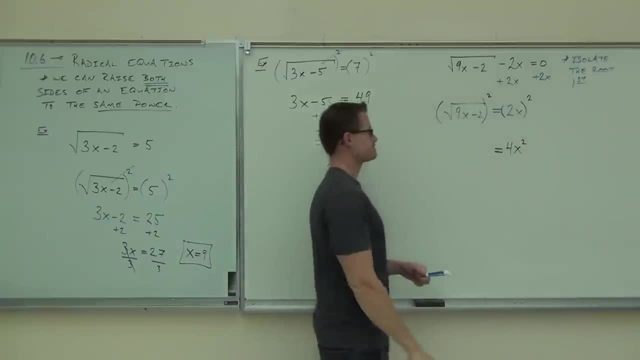 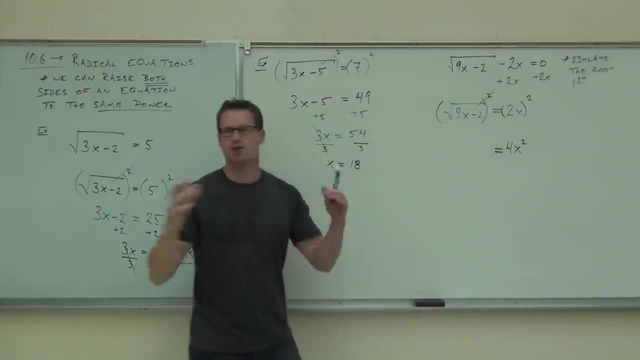 We're also going to get x squared, Now the left-hand side. well, we've done this a couple times now. The square and the square root, those things are gone. They're inverse operations. They're going to cancel, if you want to say, cancel each other out. 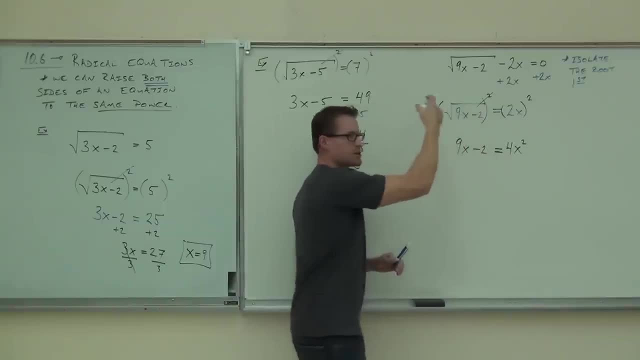 We get 9x minus 2.. No change, except that we don't have a square root anymore. Raise your hand if you feel OK with this. so far, especially the x squared, Yes, Oh my gosh. What do we do now? 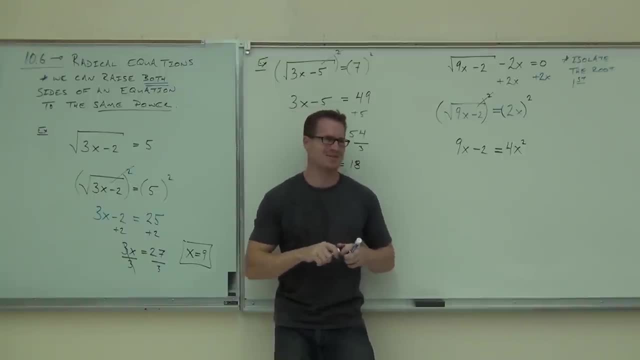 This should be exciting. Oh, this is exciting. This is a good day for you guys to be in class. I mean, you don't want to miss Thursdays anyway, because it's the best day of the week- But this day, oh, putting stuff together now. 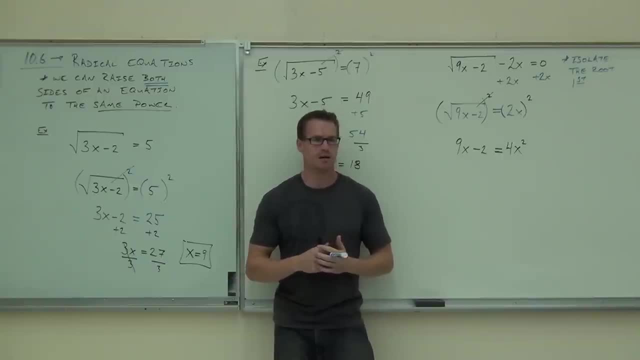 Do you see it? It's a diamond problem. Why, Why, Why, Why is it a diamond? Someone explain that. Someone else explain that You have to set it to 0.. Why do we have to set it equal to 0?? 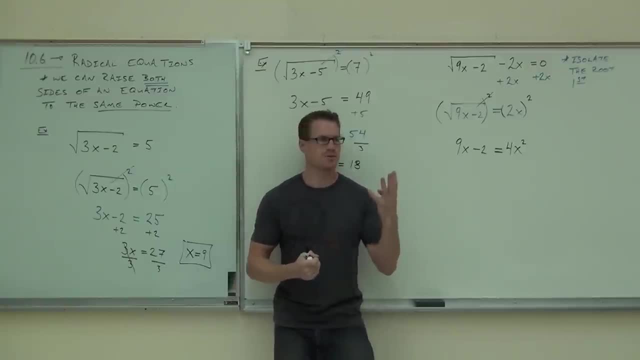 It's squared Squared. OK, that was four people who knew that. That's fantastic. Did you all see that as well? We've got an x squared. You can't solve that by any normal means. It's not like this problem right, where we just add a number and divide. 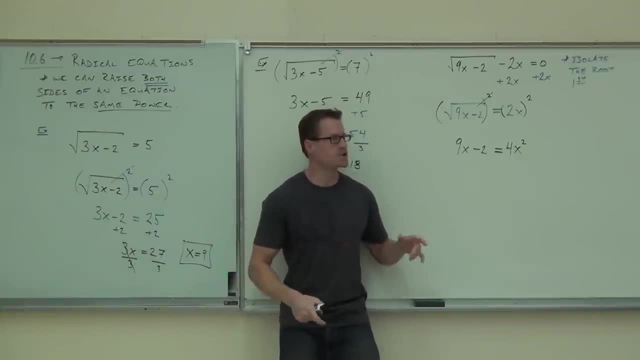 It's not like that, because we have an x squared up there. Notice how, if you would have forgotten the x squared, it wouldn't be a diamond problem. You'd be subtracting the smaller variable. You'd be something completely different. We're actually going to get two answers on this thing. 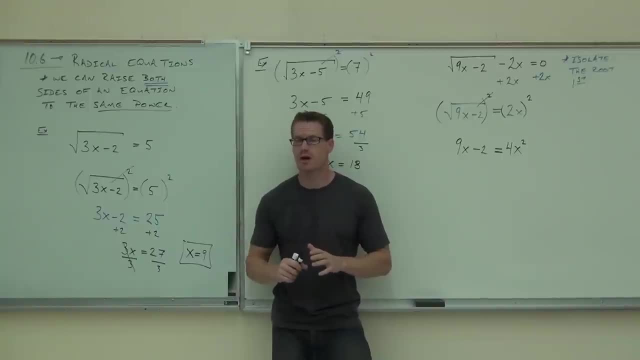 Or we should. We have the potential for getting two answers on this thing. Whenever you saw the x squared, this was way back even before this class. This was reviewed for you, like section C, the appendix C that we did. This means that you're going to get everything to one side. 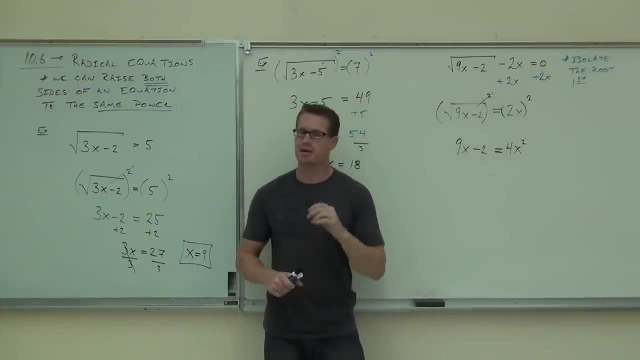 You're going to get 0 on the other side and you're going to factor this. That's what the x squared says to do. Now should we be moving the 4x squared to the left or the 9x and the 2 to the right? 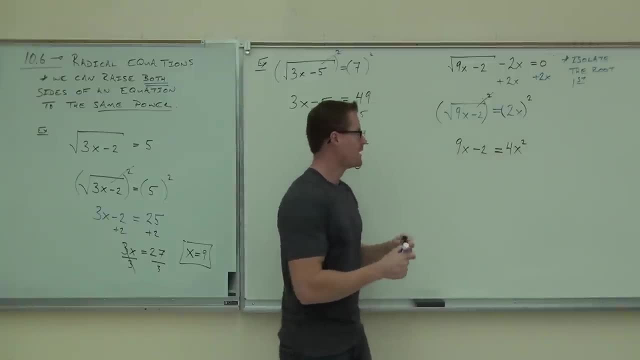 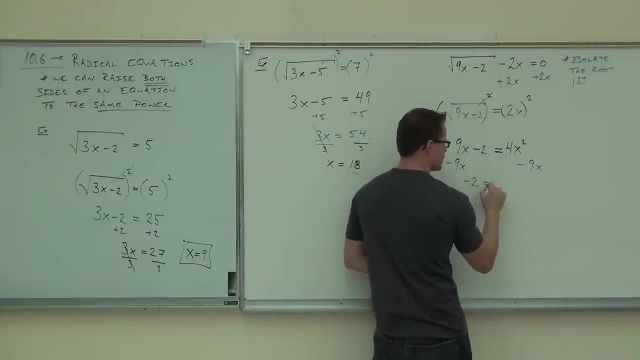 To the right. Yeah, we want to keep that positive. That way we can factor it. So that means we'll have to subtract 9x, We'll get negative. 2 equals 4x squared minus 9x. Notice, they're not like terms. 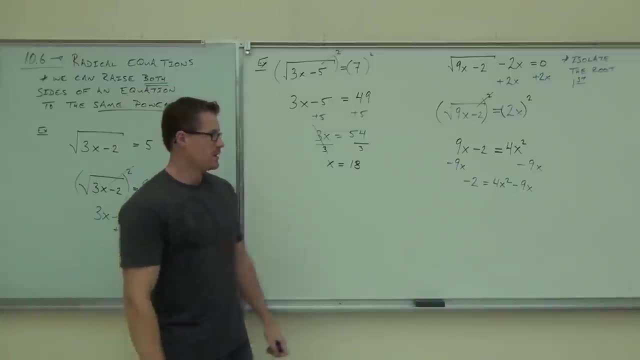 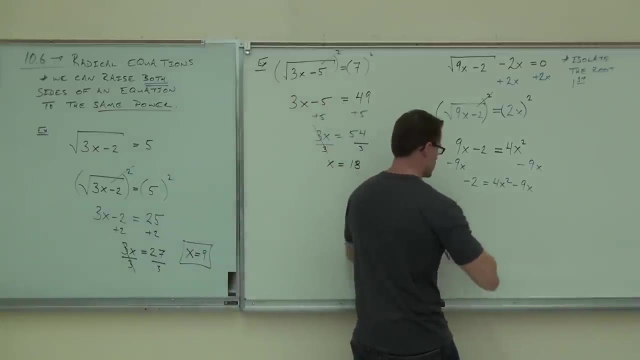 I just have to line them up horizontally. Is that good enough? No, the last thing I've got to do is: Yeah, I've got to do that as well. So 0 equals 4x squared minus 9x plus 2.. 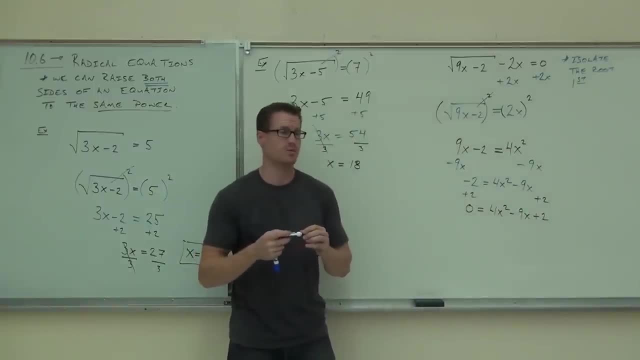 Now that should look familiar. We've done that a whole lot in this class. This is kind of where we really started the actual math process for it. We factored it. That's what we factored. How are you going to factor that thing? 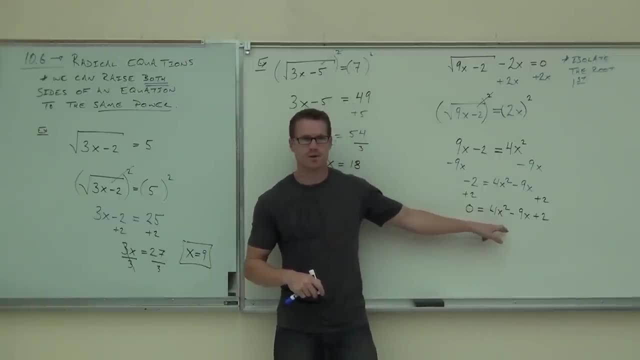 I'm going to split it into two and write it down. Sure, What did we call that Diamond? We're going to do diamond, Three terms, diamond problem. I want you to set the diamond problem. See if you can still do it. 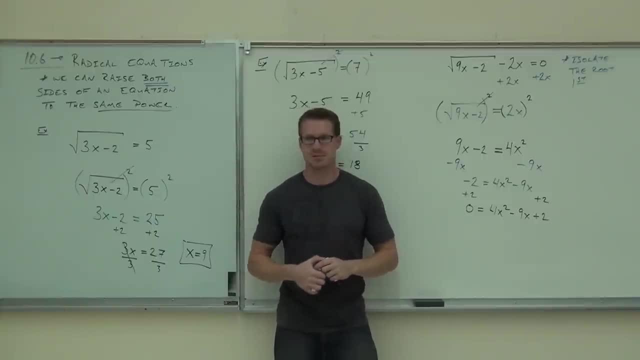 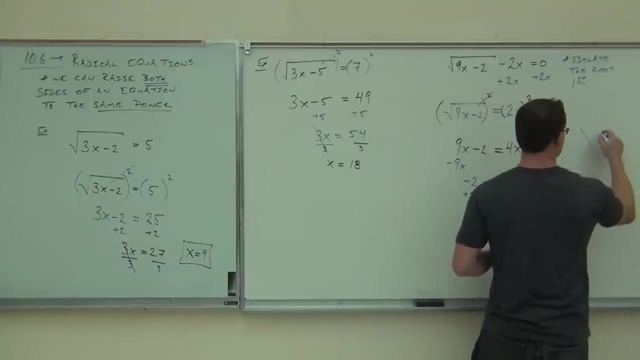 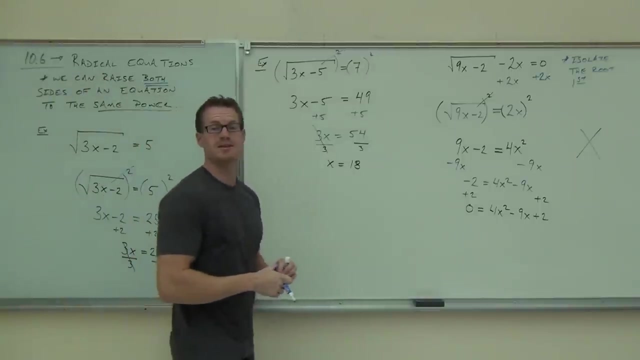 Remember what I said about spiraling information. If you lose this stuff, you're not going to be successful. You can't lose the stuff. Math is kind of a growing thing, right, It's like a tree. I'm inventing this analogy as I go. 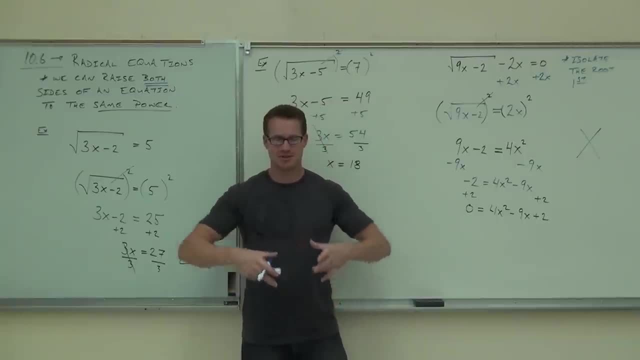 Let's see So: factoring is your roots. The stuff we learn is the trunk, And when you're successful, you get little leaves. You can't get leaves if you lose your roots. You can't get leaves if you lose your roots. 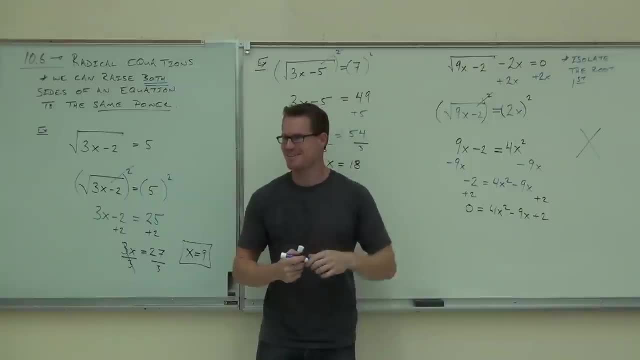 That was actually pretty good Top of my head right there. You like that? The leaves of knowledge. Oh, I could go all day with this stuff. I hope you didn't forget how to factor. My goodness, that was a key concept. 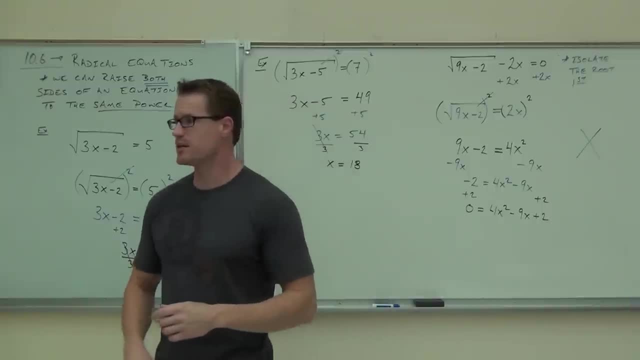 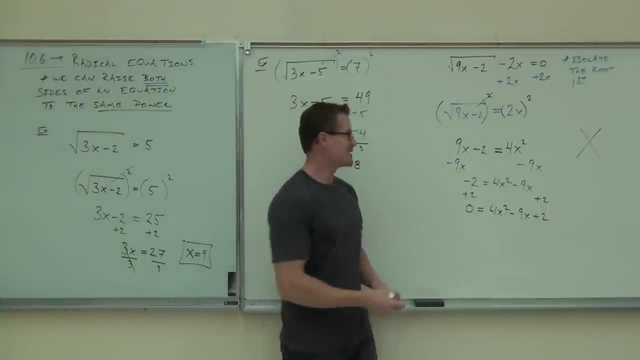 I said: if you can't factor in this class, you will not pass this class. I wasn't lying. If you can't factor, you will not pass Here. if we do this problem, we're going to get negative 9 and you're going to get 8.. 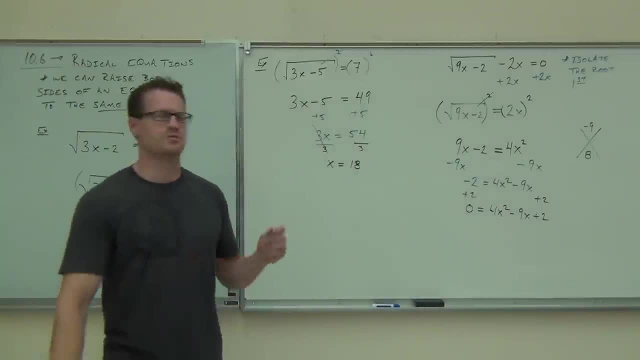 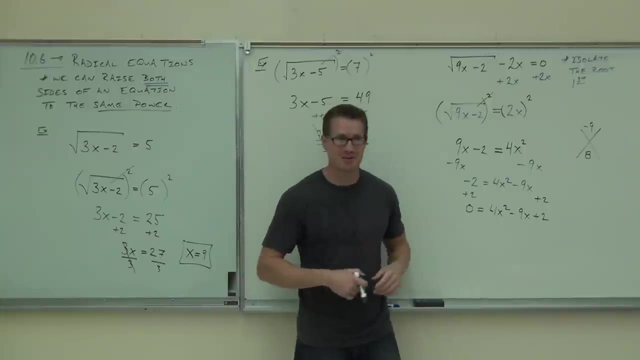 Where am I getting 8 from Four times 2.. Four times 2.. Very good, And we're going to find out what two numbers add to this one and multiply to this one. I'm going to go kind of quickly through these things because you're supposed to know how to do it already. 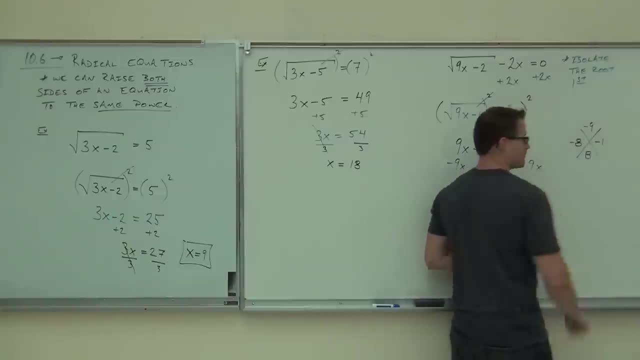 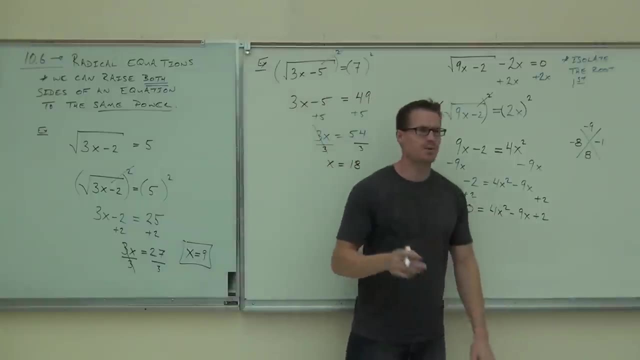 We're going to get negative 8 and we're going to get negative 1.. Those two things add to negative 9.. They multiply to positive 8.. This says- because I have a number up front, it's not a simple x minus 8,, x minus 1.. 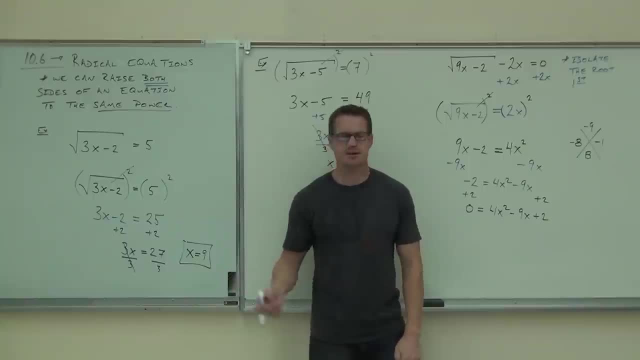 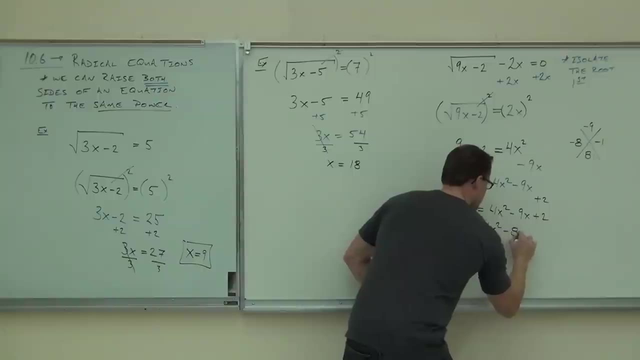 It's the extra step problem. It's a little more advanced than that. This says I can break this thing up and get 4x squared minus 8x Minus 1x. I'm going to put the 1 there, just so you see where that number is coming from. 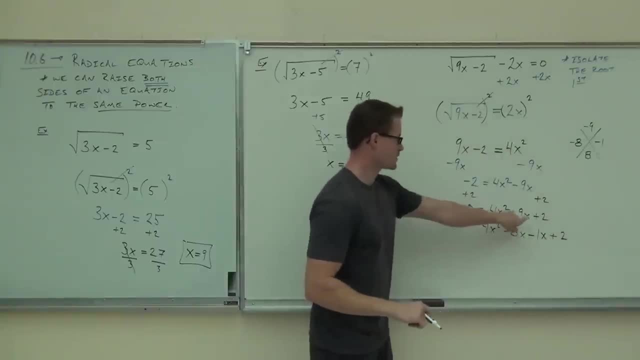 And then plus 2.. 4x squared, we split the middle term, we have the plus 2 at the very end, And then we factor by grouping. When you factor by grouping, of course, we're going to get 4x x minus 2.. 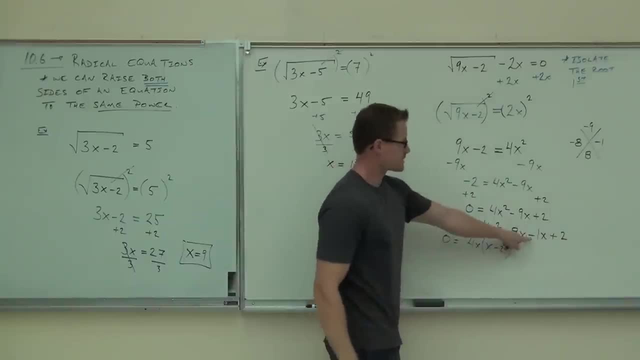 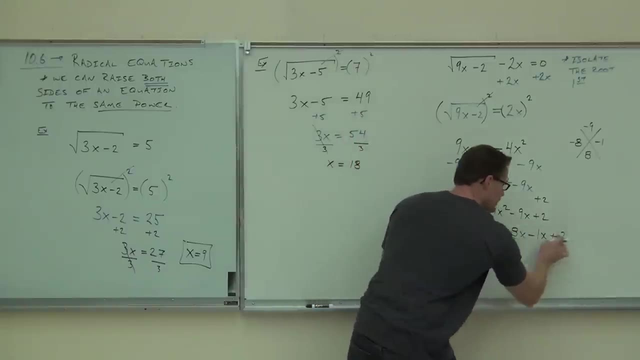 That's factored from here. This says there's really nothing much you can factor out besides a negative 1.. Why a negative 1? It's a minus. That says you have to factor out a negative. The only thing they have in common is 1.. 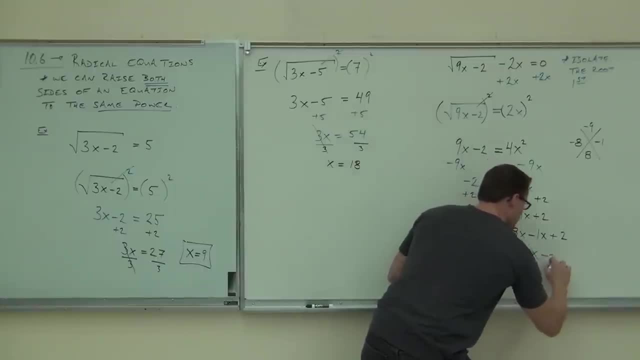 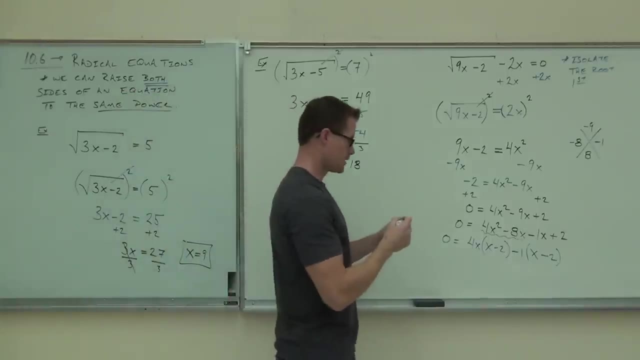 So I write my minus 1.. I get x, not plus 2, but minus 2.. Do you see where the minus 2 is coming from, ladies and gentlemen? I hope you do. I'm factoring out a negative. 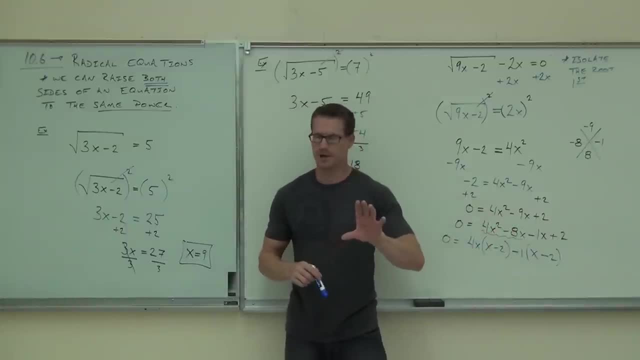 If this is confusing to you. you really- I'm not even kidding here. you need to go back today and review chapter C, the appendix there. You have to. You've got to refactor If you're losing it right here and you're like: what's he doing? 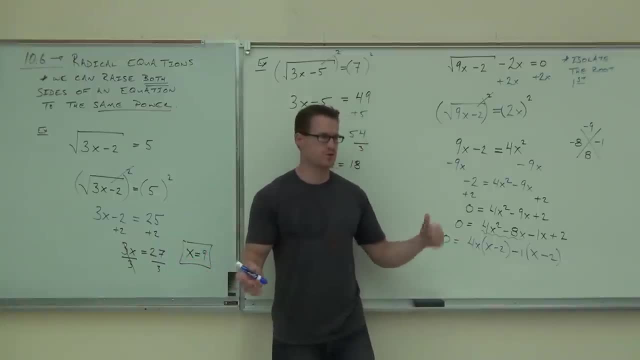 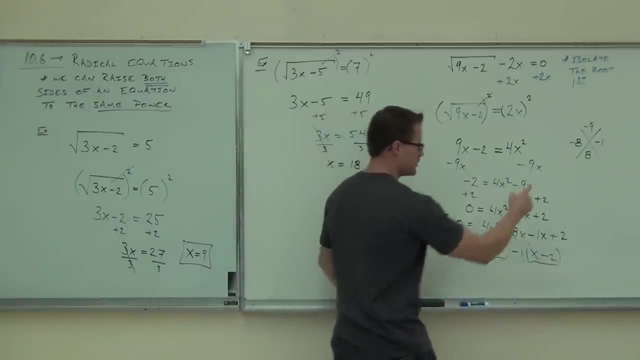 I have no idea what this is. No, you should, because that was the first week of school that we did that. Okay, factoring by grouping says when you have the same exact thing twice, you can factor it out. I'm going to move up here for you so you can actually- you know what- one more time. 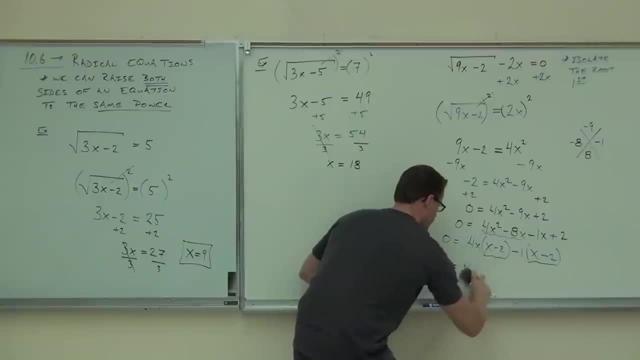 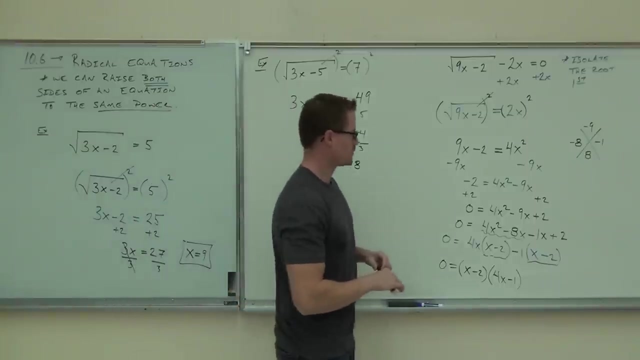 We could write x minus 2.. That's our common factor. We write the remaining stuff, 4x minus 1, and that's factored. Okay, Now, after you have it factored, are you done? No, you have to set each one equal to zero and then solve it. 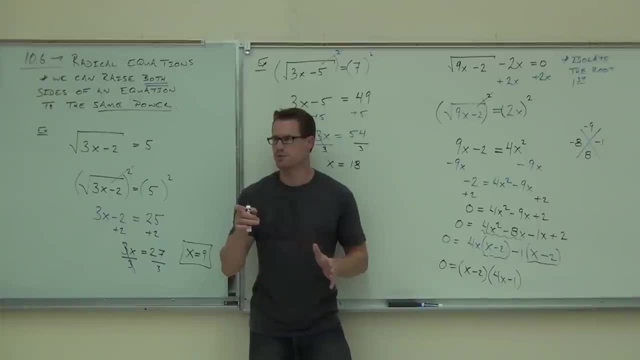 What's that called on the right-hand side of the room when we set each one equal to zero? Why do we get to do that We do. That's why we do it. What lets us do it? The zero rule. Okay, yeah, it's called the sum zero rule. 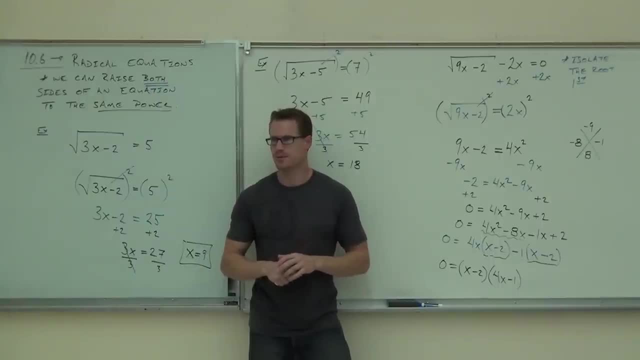 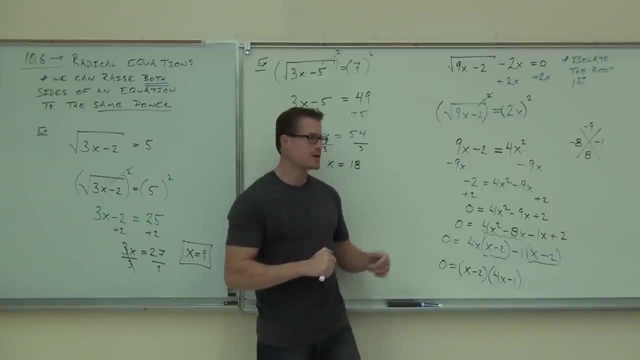 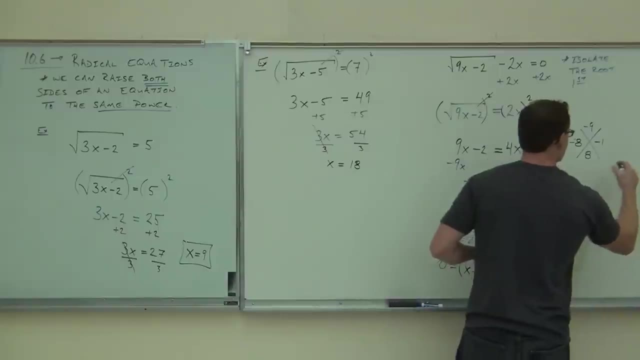 You can do it. You can do it. You can do it. Zero product property. It says that if you have two things that are multiplied together that equal zero, you set each one of them equal to zero. I'm going to make a little section over here. 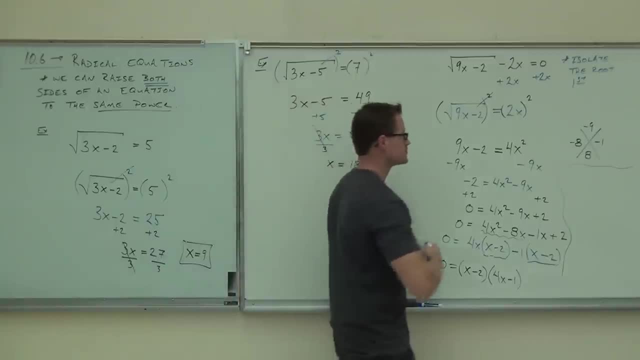 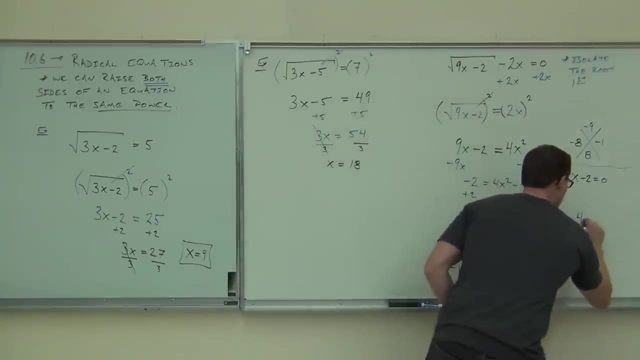 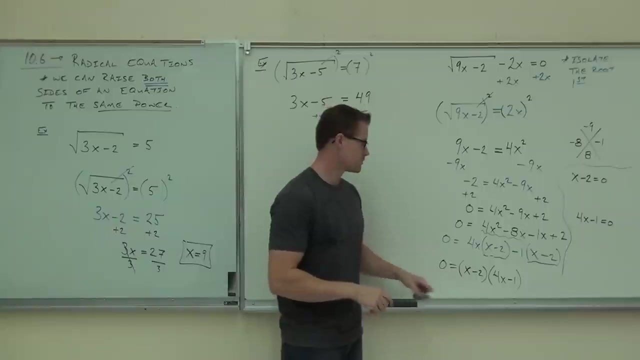 We get to set x minus 2 equal to zero. That's the first one. We also get to set 4x minus 1 equal to zero. By what? By the way, we absolutely have to have a zero for that to work. 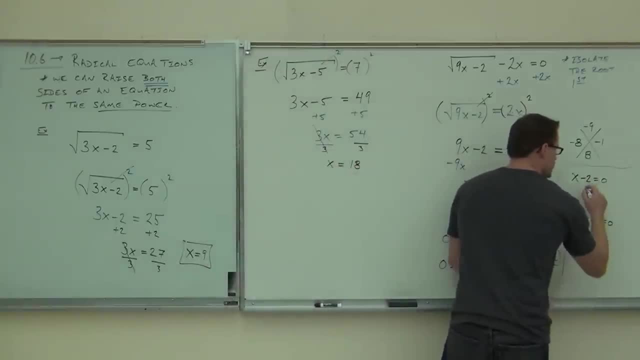 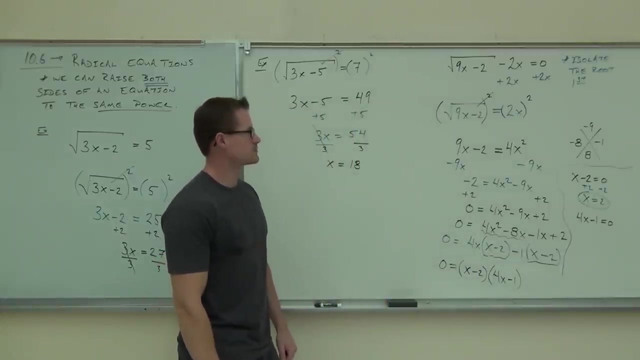 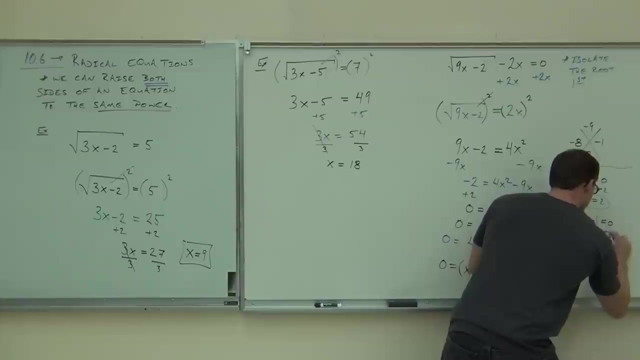 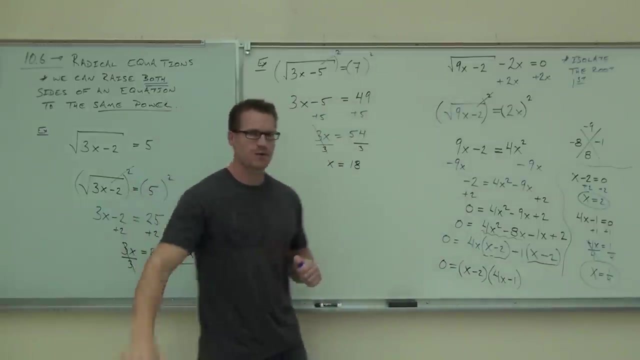 Any other number isn't going to happen. If we add 2 here, we're going to get x equals 2.. So far, so good. Yeah, If we add 1 and divide by 4, would you really feel okay with that? 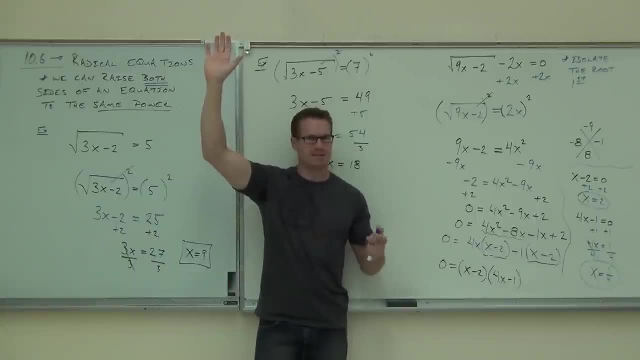 How about okay with the factory? Now, honestly with me, how many people kind of were iffy on the factory? Okay, that's all right, That's all right, but you need to go back and look at it. If you knew you were iffy on the factory, go back tonight and look at the factory. 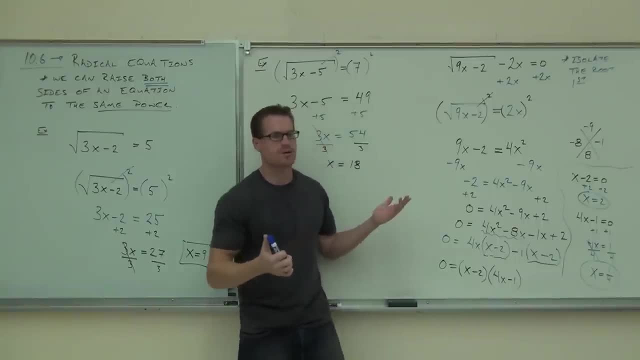 Are you with me on that? Because otherwise, I mean honestly, this is easy. Adding 2x and squaring both sides, that's easy, It's really really easy. But then doing this part, that's the tough part and that's old stuff for us. 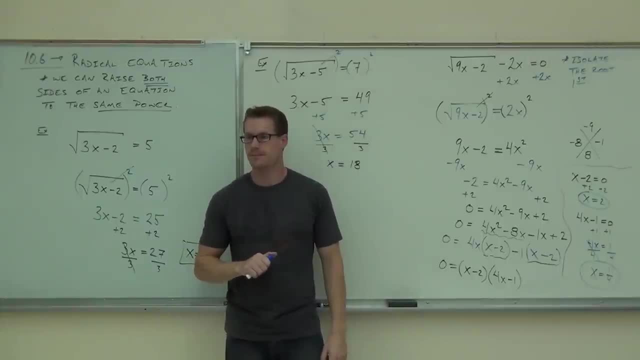 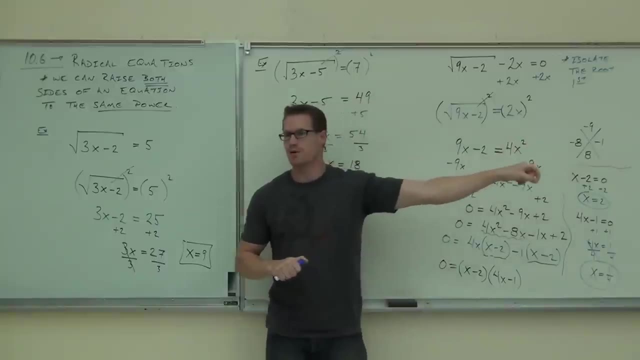 Brenda, When you do diamonds, does the middle term always go on top, or can it be like such: Yep, this one goes on top and these two go on the bottom. You add to the top, you multiply to the bottom. 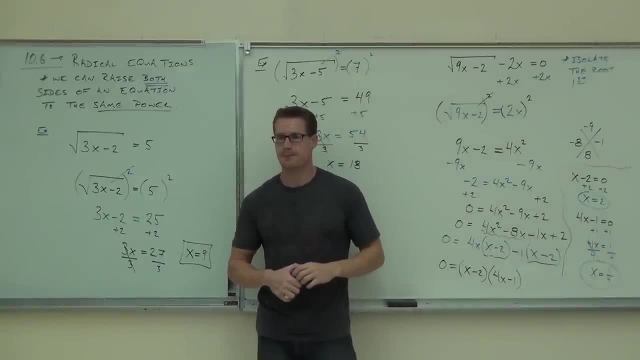 Go review that tonight on that video. okay, Was the diamond? was that in Chapter 9? Chapter 7. Chapter 7. Actually, no, Chapter 7. Before Chapter 7. So it's still in the appendix. It's in the appendix. 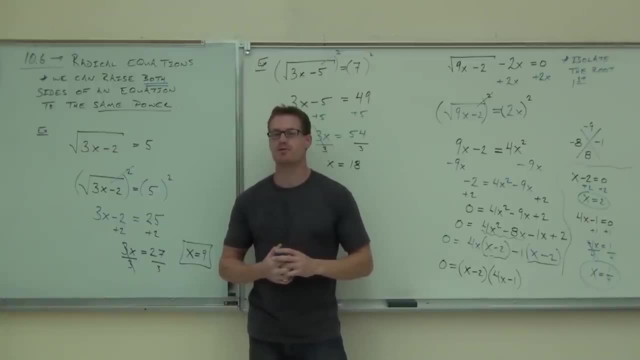 C.4.. If you are having trouble on factory, C.4 is for you And C.1, where you did the equations. The equations are C.1.. C.4 was just factory and stuff. It's a good lesson, guys. 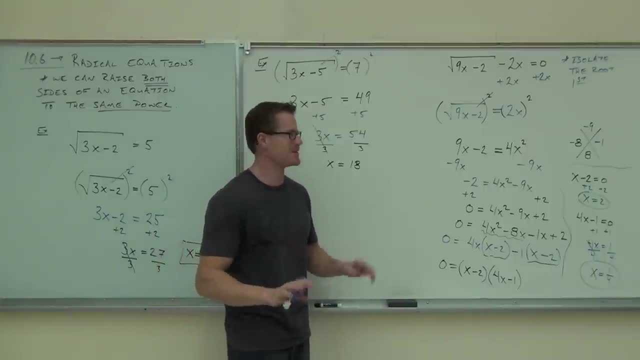 I mean, I watch them all the time just to kind of feel good about my thing. No, I'm just kidding. Are we going to have that, those examples with different votes on one one? Mm-hmm, Any of those different votes? 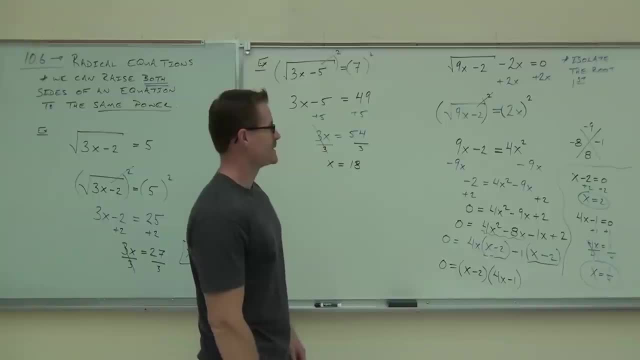 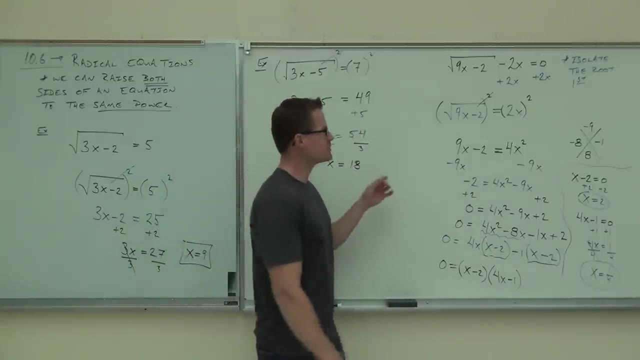 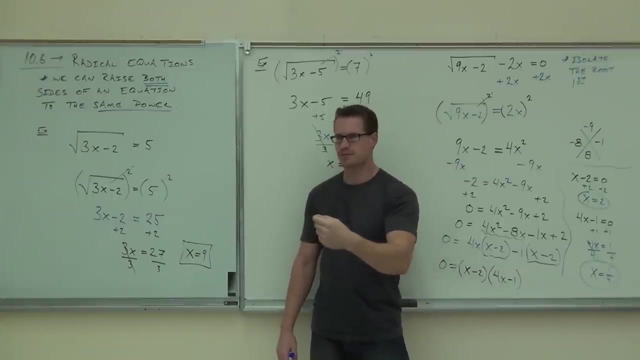 Mm-hmm. Now, one thing you do have to do: you've got to check your answers, Because occasionally, when you do this process, you eliminate something that is kind of weird on these things. You make negatives positives. You see that. 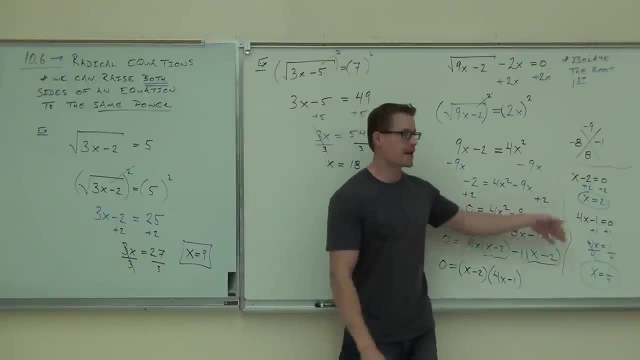 When you square something, you make negatives positives, So occasionally you're going to get an answer that really doesn't work. Now I'm not sure that that's going to happen on this example. It doesn't, But occasionally you'll plug one in. 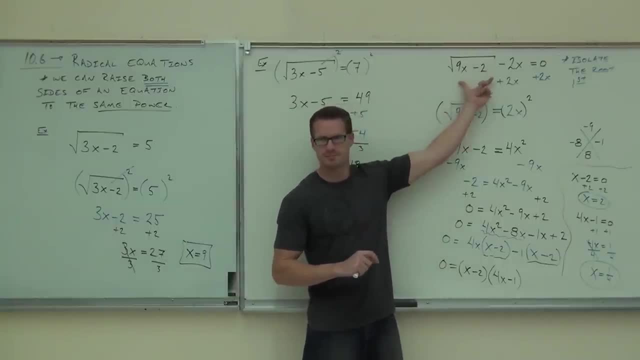 and you'll get a negative inside of a square root. Is that OK to get? No, OK, So you've got to check both answers Here. you check two, You're going to get 18 minus 2. That's 16.. 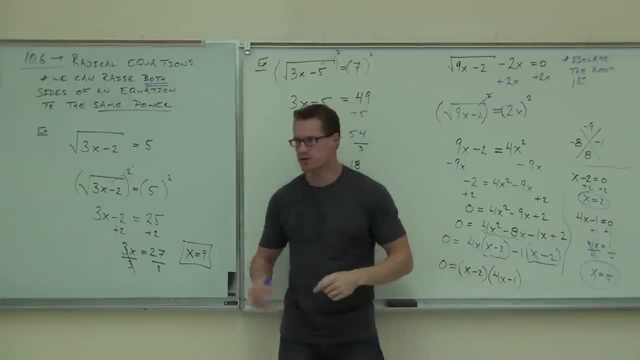 That's 4 minus 2 times 2 is 4.. That's 0.. That's OK, That works The one quarter you get. oh my gosh, it's hard to check, But you can do it. 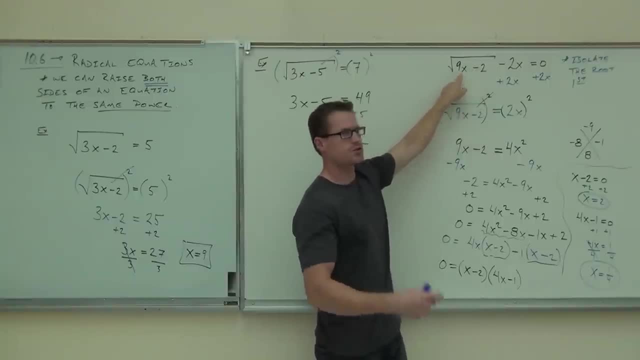 You get one fourth, I'm sorry, nine fourths. That's greater than 2.. So when you subtract 2,, you get one fourth. Square root of that is one half Minus 2 times one fourth. That's also one half. 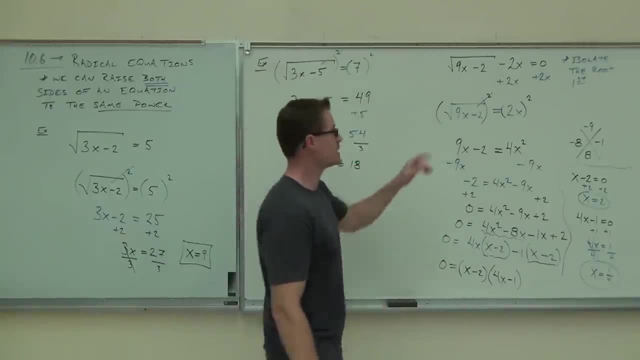 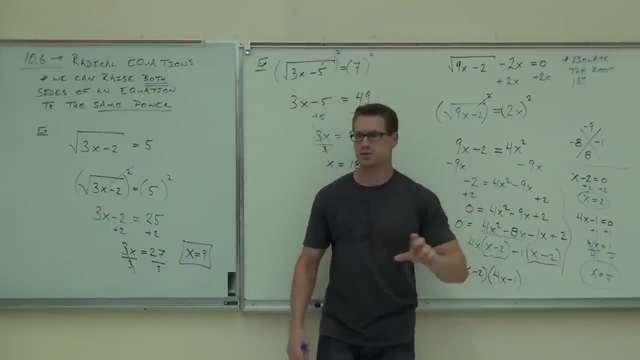 You would still get 0.. But you need to check it. You do, Because if you get a negative inside of a square root, that's a bad thing. That would be a complex number. You can't deal with that. This occasionally will make up some solutions. 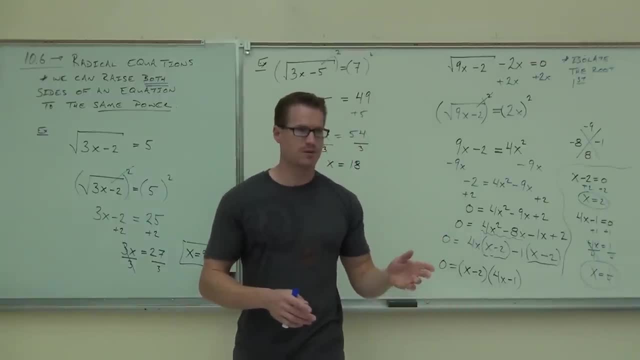 that are not actually true. You follow. You've got to check your work. You've got to check your solutions. I'm going to have you do one of your own, very similar to this, and see if we can work our way through it. 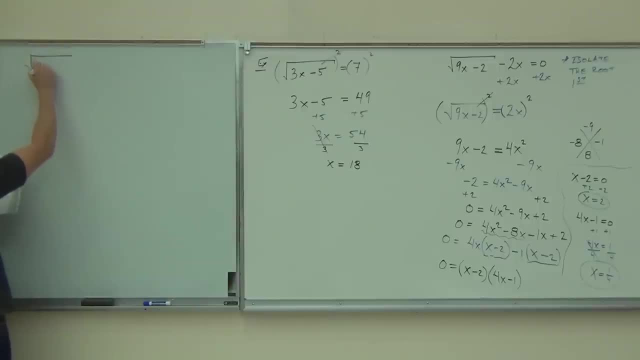 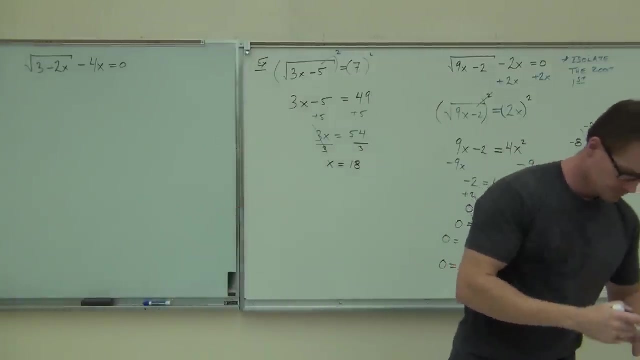 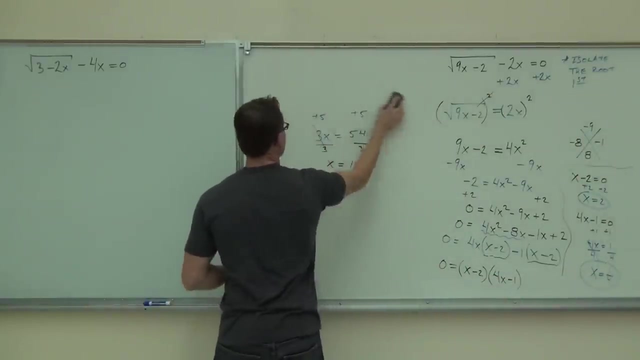 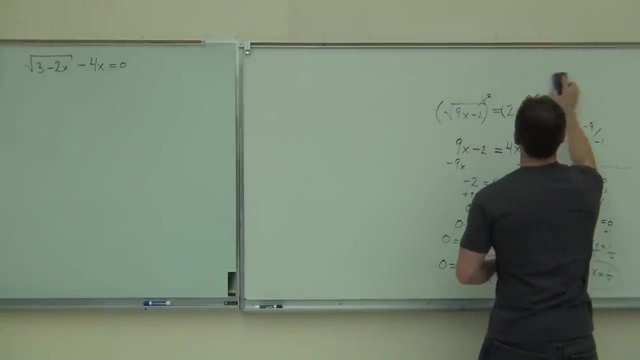 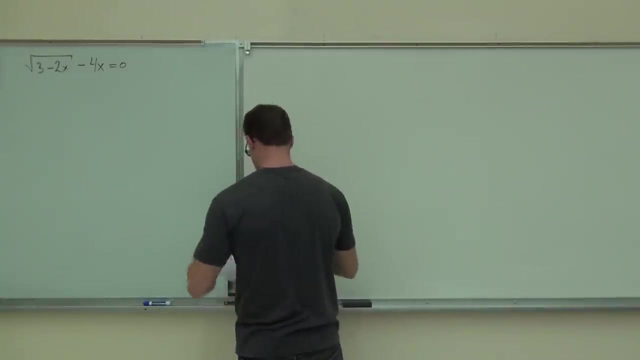 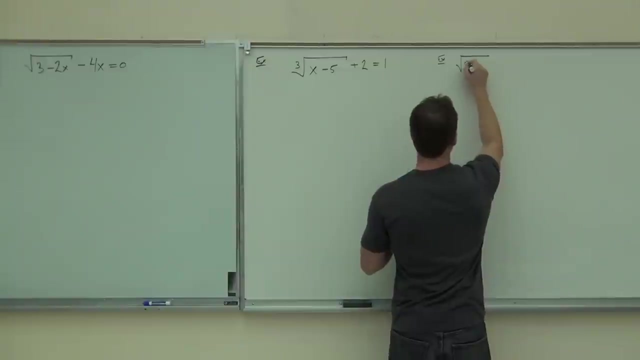 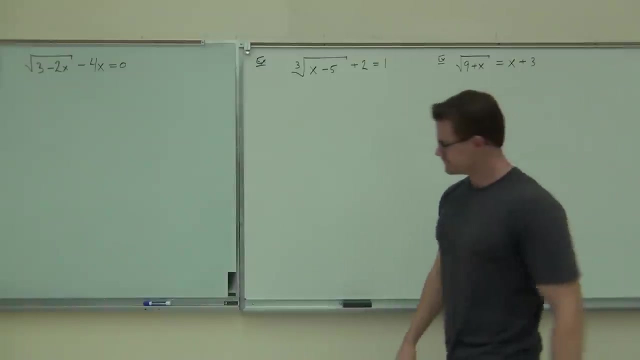 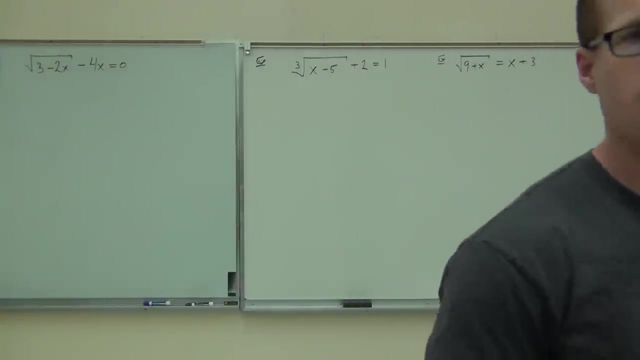 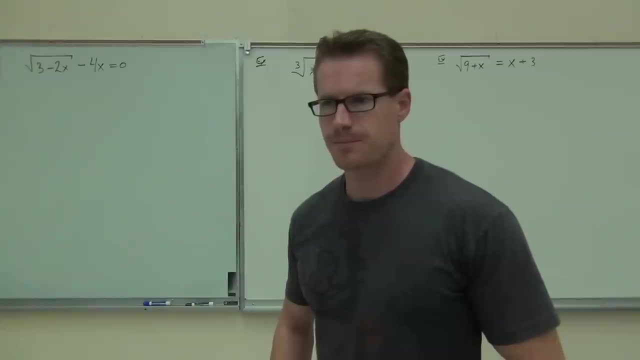 Don't worry, Thank you. So first thing you must do, of course, isolate your roots. So do that. first Get that root all the way by itself. After that, use the appropriate power to get rid of the root and then solve it. 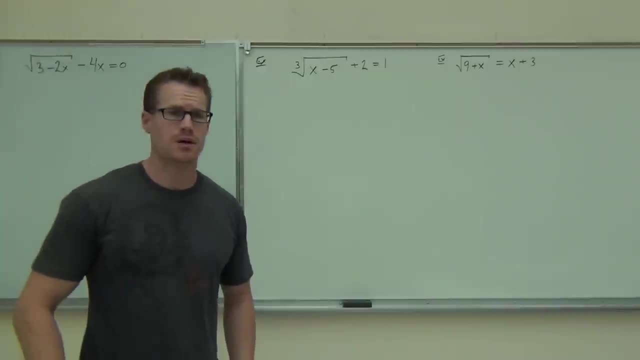 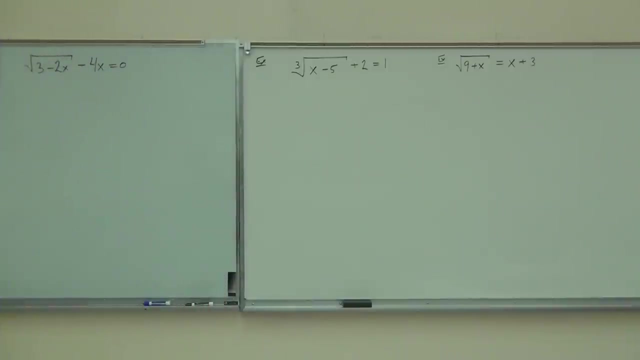 If you get an x squared, you know you're going to factor. If you don't get an x squared, well, no problem, You can solve that one pretty easily. In this one did you get an x squared? Yes, Okay. 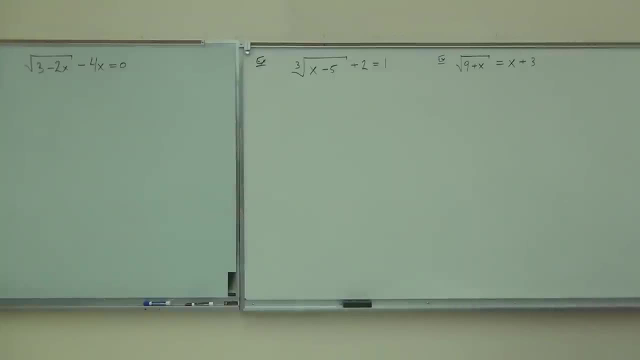 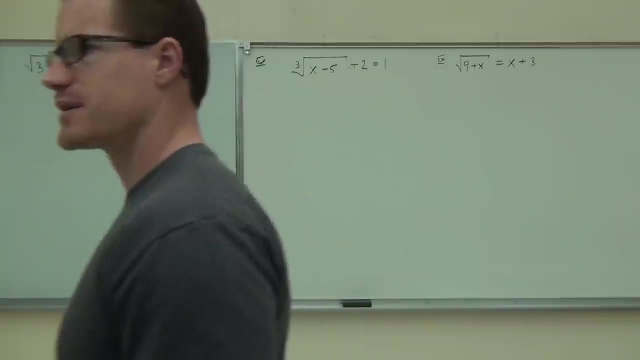 Okay, Thank you, Thank you, Okay. I see a lot of good work on people getting all the way down to the factoring. You know what that tells me? It tells me that you understand the concept. It's the factoring. that's the thing that might hold you back here, right? 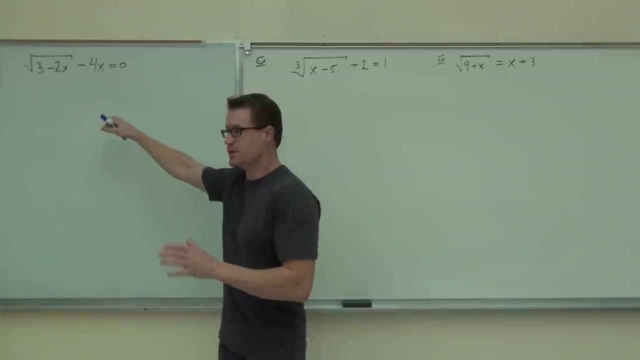 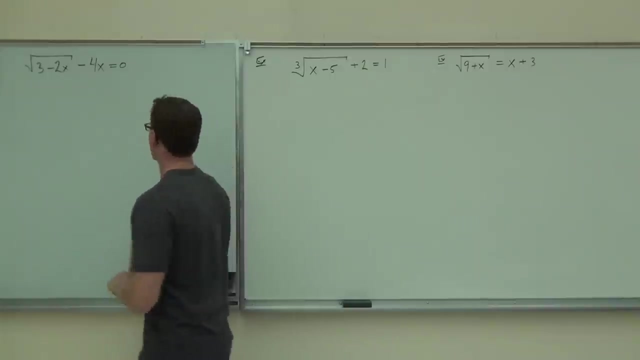 It's not the problem. I mean, the problem is okay. You all got down to where you're supposed to factor. Let's just make sure that we drive this home, make sure we know how to factor, That way that part doesn't hold us back. 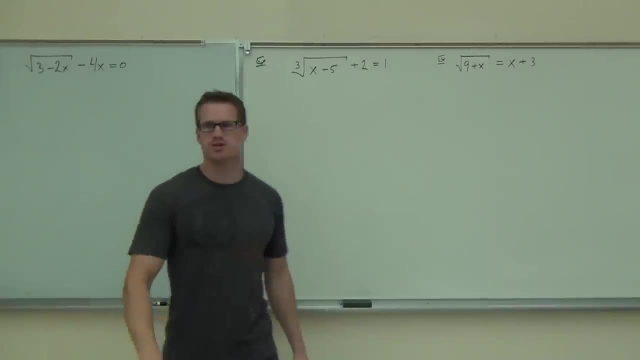 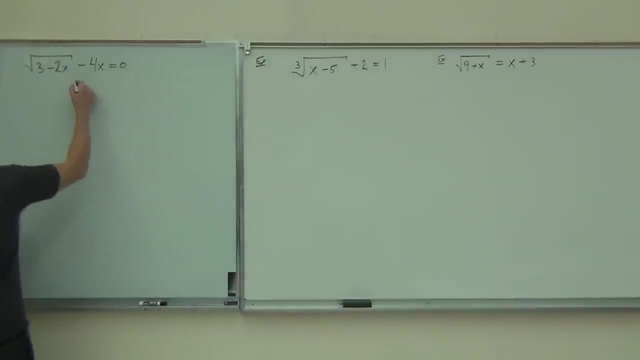 So, on our problem here, the first step is to square both sides, True or false. True, First step is to square both sides, True or false. False, Definitely false. We're going to add 4x to both sides. The reason why is because 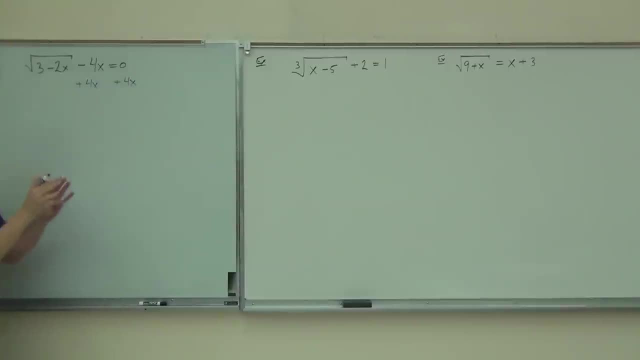 True. well, we really can't do much unless our square root, or whatever root we have, is isolated. 3x minusI'm sorry, 3 minus 2x equals 4x. Did you make it that far? Yes, 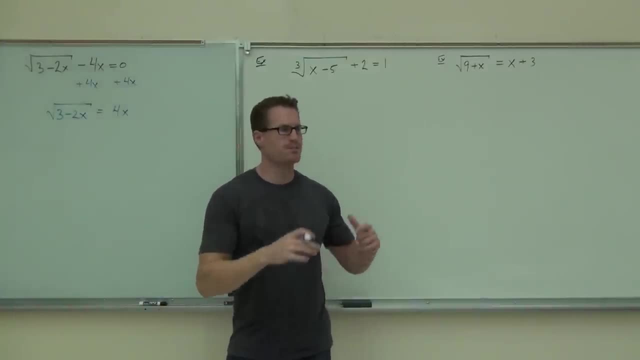 Good deal. Next thing is understanding that we're going to have to square both sides on this problem. We use a square because we have a square root. If we had a different type of root, we would use a different power. So in our case, right now, we've got a square root. 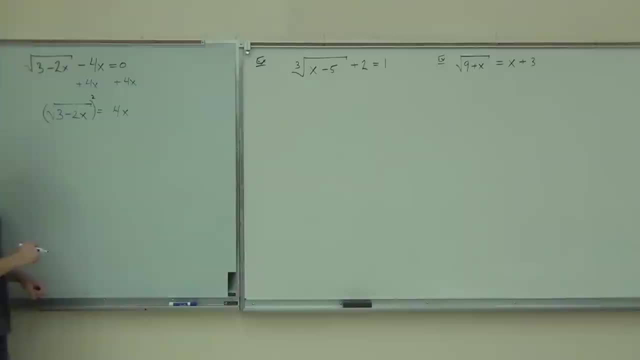 We're going to square this side And we're going to square the 4, the x or both, wouldn't we Both? Yeah, because really we're squaring this whole side. So you needed to get 3 minus 2x equals not 4x squared, but 16x squared. 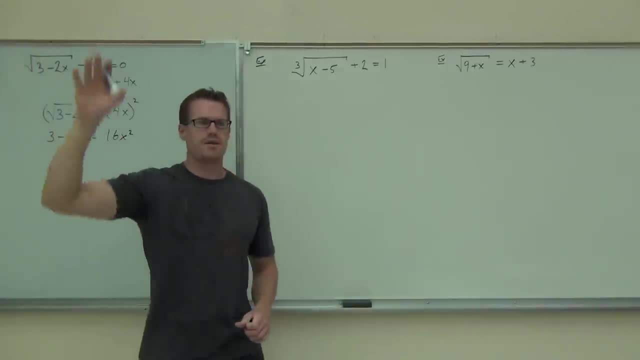 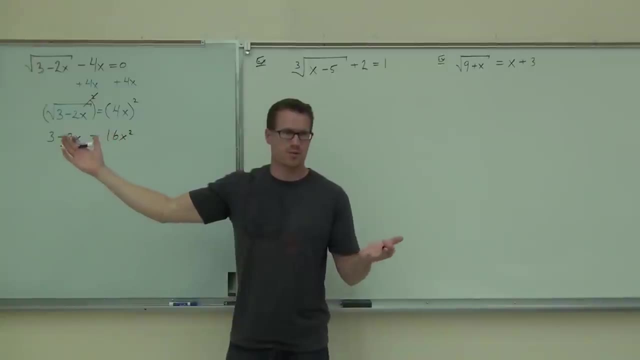 Rachel, have you gotten that far? That's good. That really right. there is the end of the concept for this section. That's it. This is really it. Isolate a root, take the power to both sides. That's all I taught you. 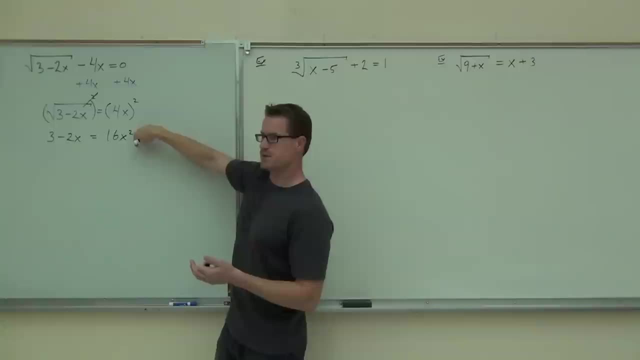 This: if you ignore this top part, that's no problem. We've been doing that since the appendix, the review for this class. So now is where you tie in all that old crap that you learned. You're like: oh, I can forget about that now. 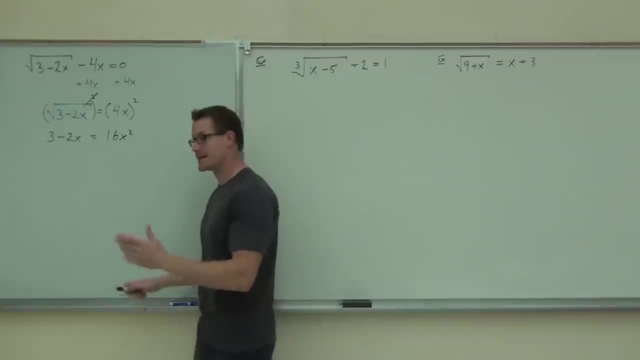 I've had the first test. Ha ha ha. Oh, you can't forget about it now. We've got to keep going with this stuff. So of course, we have a square x squared. We're going to get everything to one side and 0 to the other side. 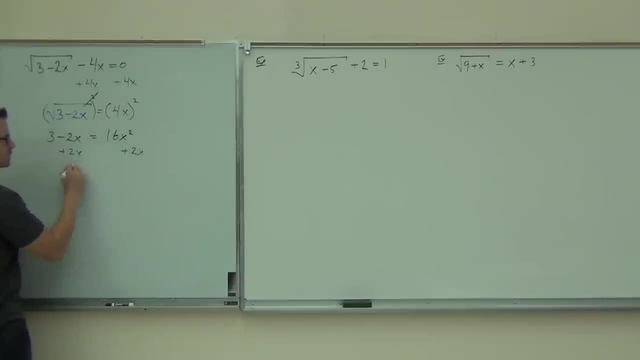 In this case, we're going to add 2x. We'll get 3 equals 16x squared plus 2x, And we're going to have to subtract 3 as well. We get 0 equals 16x squared plus 2x minus 3.. 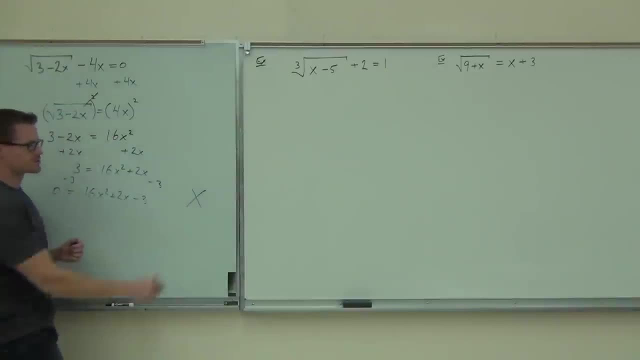 This says that we're going to need a dyno problem. Are you going to get the extra step or not? Yes, We've got a 2 up there. We've got- oh, it looks like a, what is it- 48?. 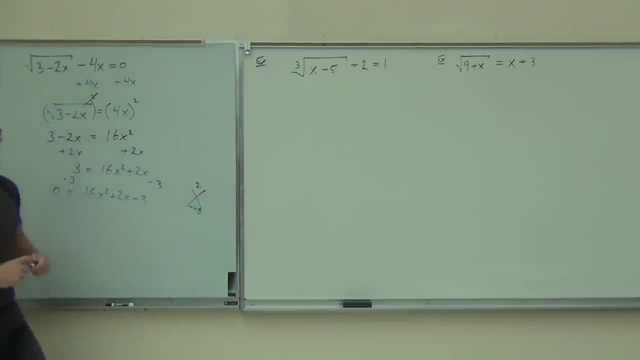 Negative 48.. The only two numbers I'm seeing are a 6 and an 8. somehow Probably a positive 8 because it's adding to a positive 2. And a negative 6 because I need to get a negative 4.. 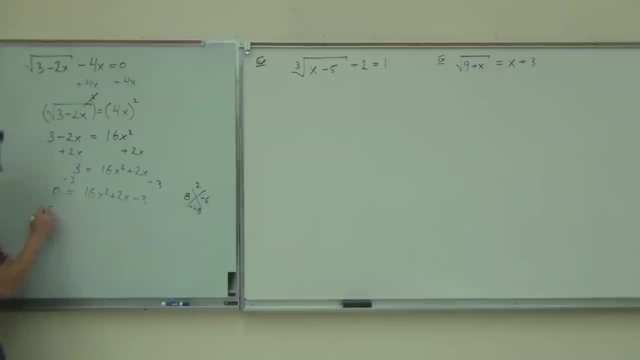 So 8 and negative 6. And I'm going to split up the middle term. That's what this allows me to do: 16x squared plus 8x minus 6x minus 3.. We factor by grouping and we get factoring out a 4,, I'm sorry, an 8x here. 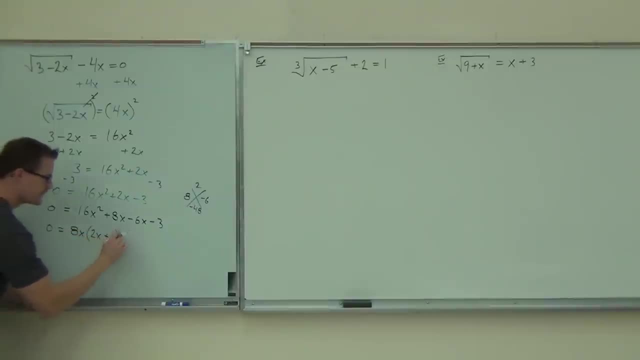 Factoring out 8x, we're going to get 2x plus 1.. This says you're going to factor out a negative. That sign says a negative 3. And you're going to get 2x plus 1.. 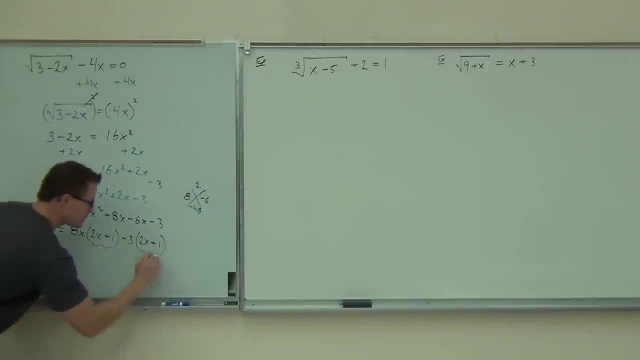 That's because you factored the negative out. Now that we have the same thing in both spots, of course we factor by grouping And we get 0 equals 2x plus 1.. That's what you're factoring, And what's remaining is 8x minus 3 in another set of parentheses: 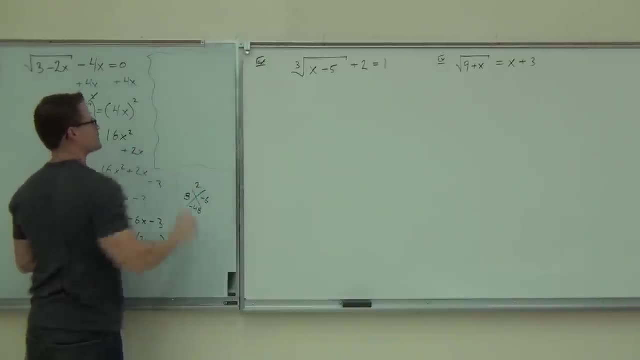 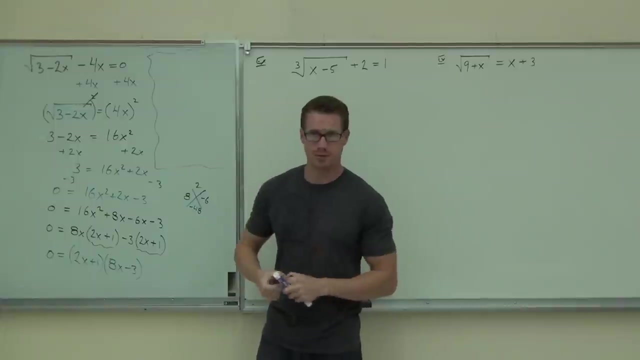 I'll make some room over here for our solutions. Zero product property says you've got two things that are multiplied together that equal 0. Each one of them equal to 0. That means you're going to get the 2x plus 1 equals 0.. 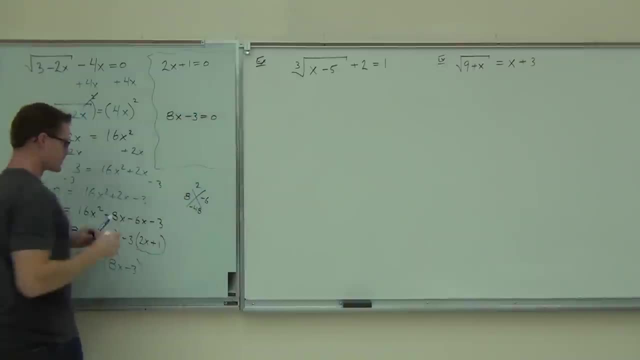 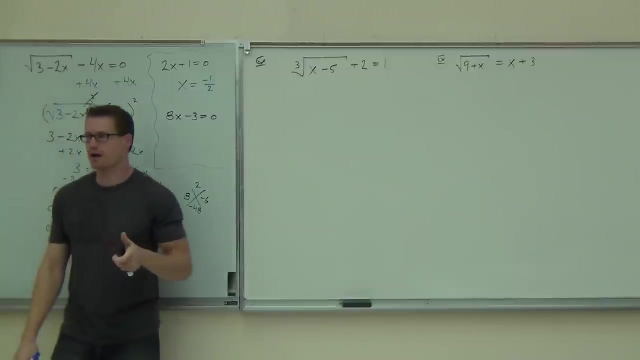 You're going to get the 8x minus 3 equals 0.. If you subtract 1 and then 2,, x equals negative 1 half. Did you get negative 1 half? Yes, Okay. If you subtract 3 and divide by 8,, you're going to get x equals positive 3 eighths. 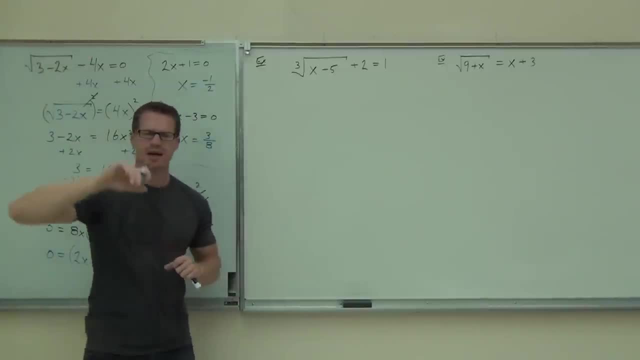 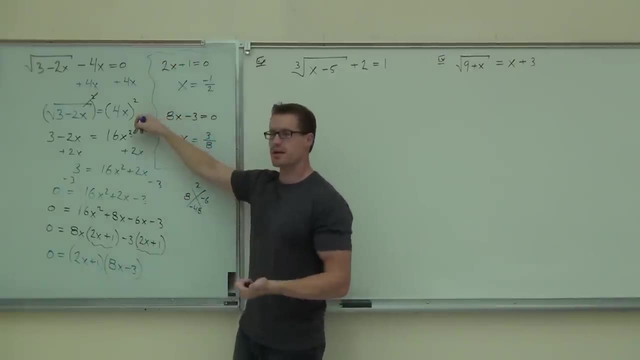 How many of you got positive? 3 eighths, Okay. How many of you will be able to make it all the way down? That's good. If you didn't, if you made it to here, that's great. That means you understand the concept for this section. 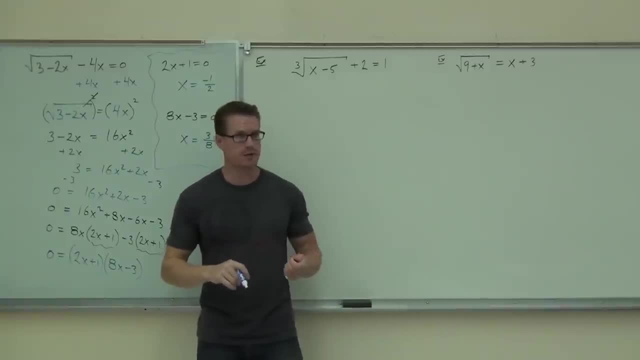 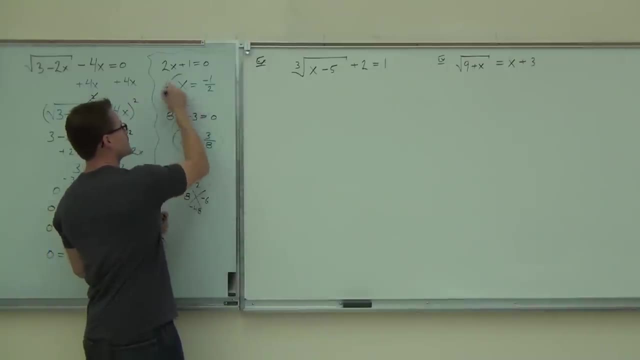 But if you didn't make it down to here, that means you need to review your factoring. At least you know what you need to review, right Right there. So we get our two solutions. Well, we do got to check them, though. 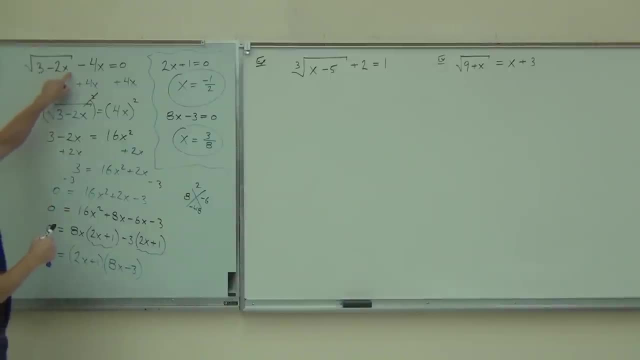 If we check these, we're going to have 3 minus 2 times negative, 1 half. That's going to make it positive. I know for sure I don't have a negative inside that square root. That's great. That's what we're looking for. 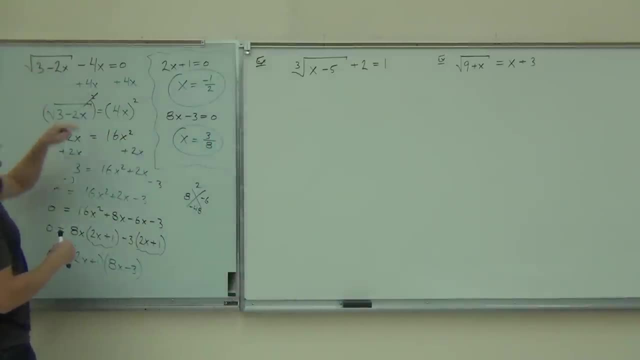 Here. you've got 3 eighths. You're going to get 3 minus 3 fourths. That's still not going to be a negative inside the square root. That one's also going to work out for us. So we've got our two solutions there. 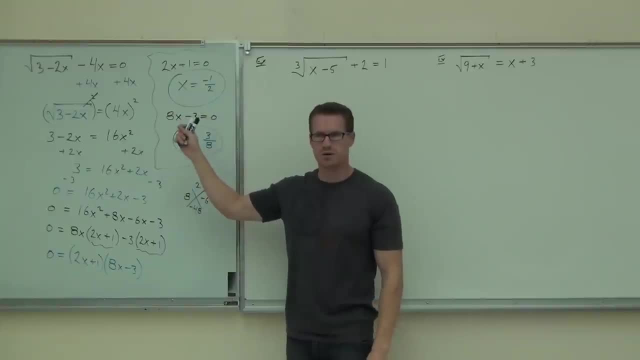 Did anyone double check those all the way through to make sure that they actually work? Do they work? No, 1 half doesn't. 1 half doesn't. OK, let's see why. So if we plug in negative 1 half, we're going to get what is that? 3 plus 1.. 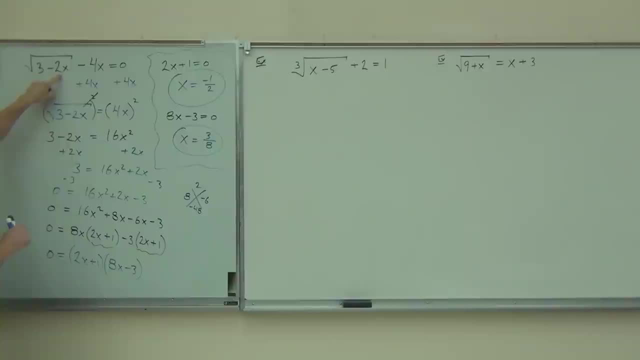 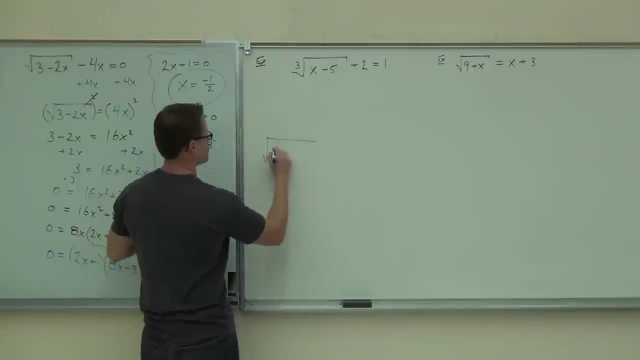 That's 4.. Square root of 4 is 2.. Yeah, that doesn't work. All right, here's why, If you plug this in, you're going to get the square root of 3 minus 2 times negative 1 half. 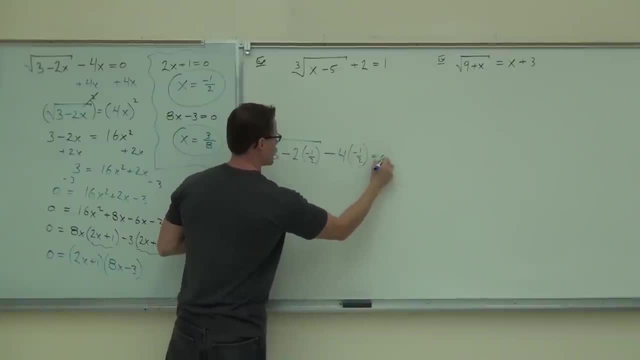 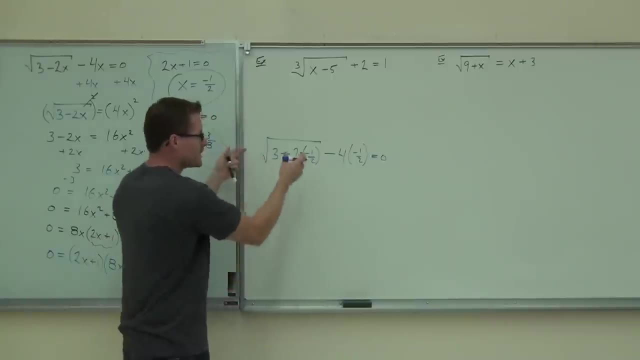 Minus 4 times negative 1 half. See what happens. I was telling you this earlier. sometimes it switches the signs on you and tells you that a negative's going to work in these cases, But here we're going to have 3 plus 1.. 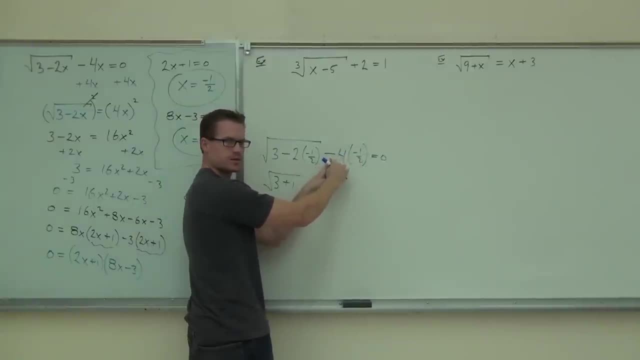 See how the negative and the minus are going to make a plus. This is plus 2.. This is 2 plus 2, not 2 minus 2.. That's going to give you 4.. Is 4 equal to 0?? 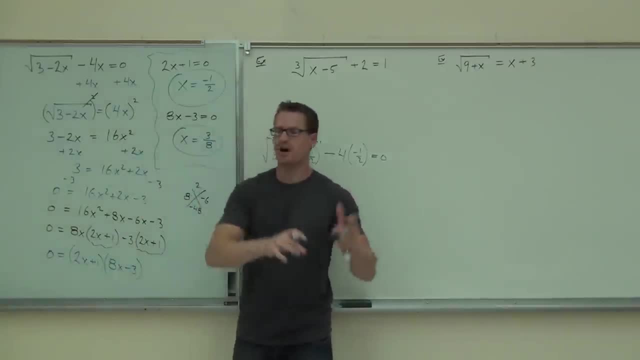 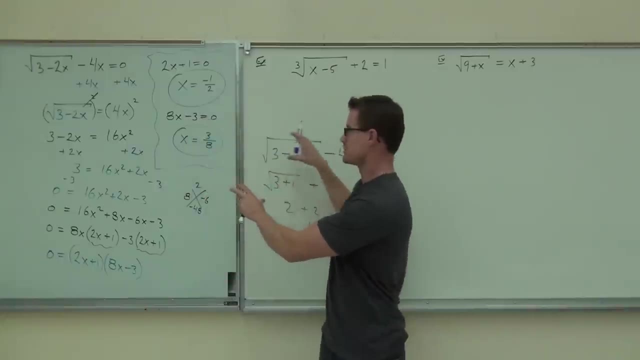 That's bad, That's wrong, That square changes some negatives to positives for you. That's the problem. It's going to make it seem like some answers are solutions, when they're not, And the two situations you get is this one which we see here. 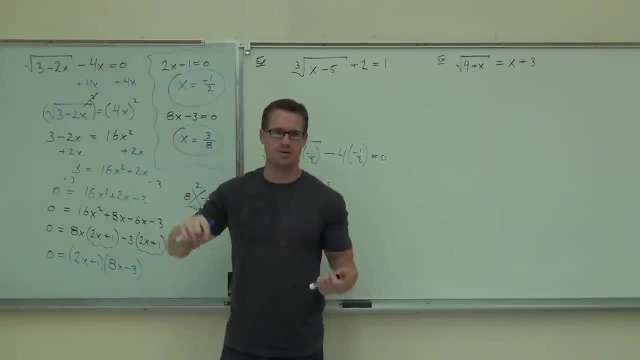 Or sometimes you'll get something that's a negative inside your root and you can't have that either. So there's two cases you've got to watch out for How many of you understood that idea. OK good, I'm glad you checked that. 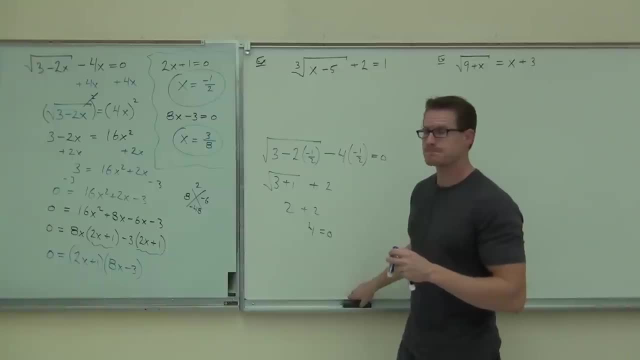 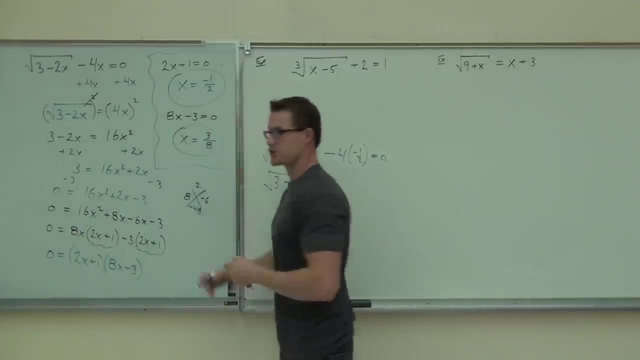 So when we get that, do we line through that? Yeah. So we'd say, OK, how many solutions do we actually have here? That one doesn't work, So you'd show both, because the potential is both are going to work. 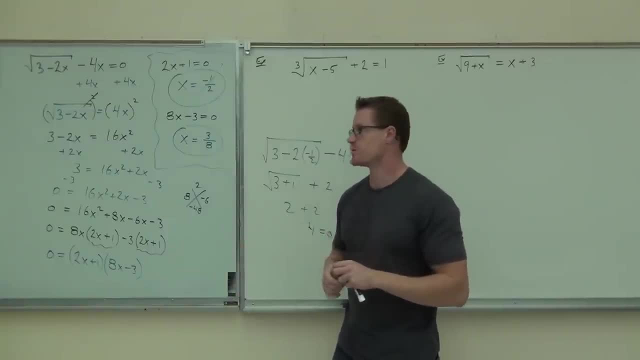 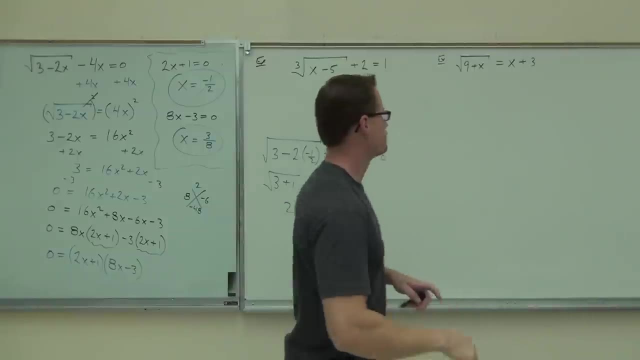 But you have to cross the one out that if it doesn't work, you cross that one out, It's not just because it's negative. You actually have to plug that in and check it to make sure it works. OK, Are you ready to move on? 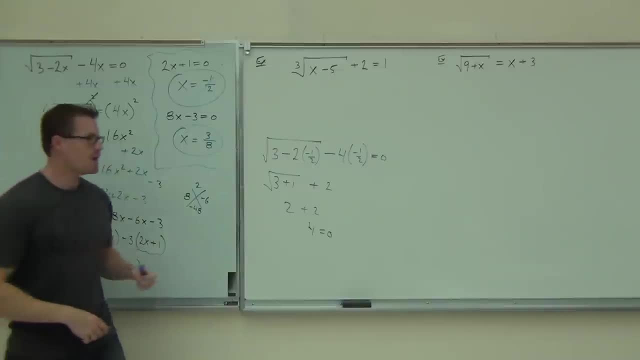 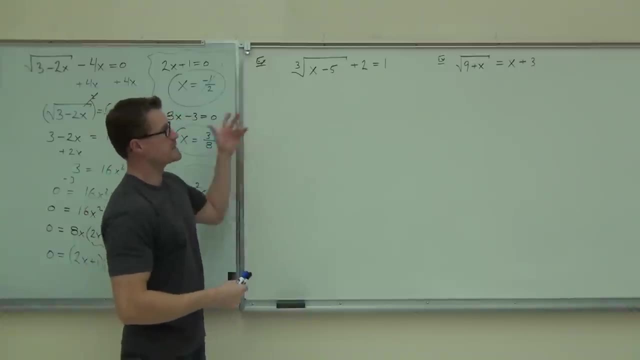 Are there any other questions on this thing? Let's work through these two. We kind of have the idea down. This was the only idea I was going to teach you today. That's it. So, using those ideas, what's the first thing I need to do on that problem? 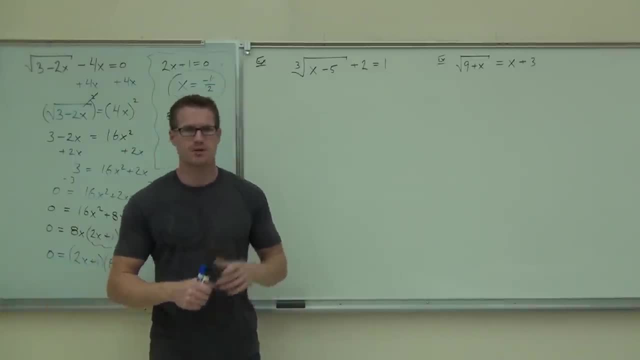 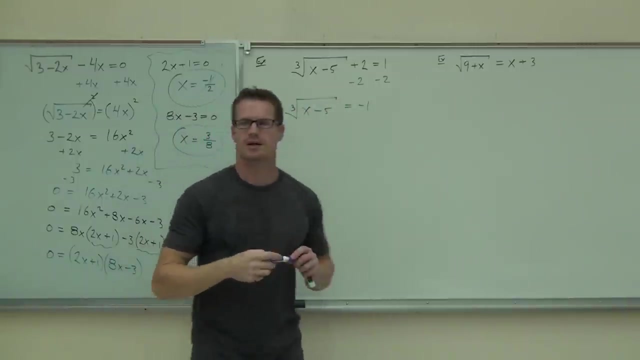 In other words, isolate the root, right, Whatever we got. So here we're going to subtract the 2 for sure. Cube root of x minus 5 equals negative 1.. I'll give you a little hint. Is it OK to have a square root equal to a negative? 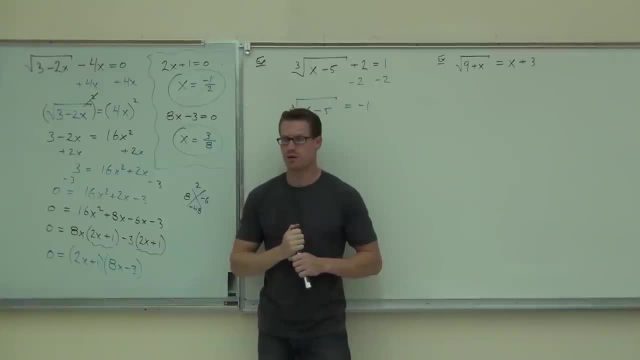 A square root? No. Square root, no. How about a cube root? Yes, That would be OK. A square root is never going to give you a negative. You can't get a negative out of that. That's what we do with complex numbers. 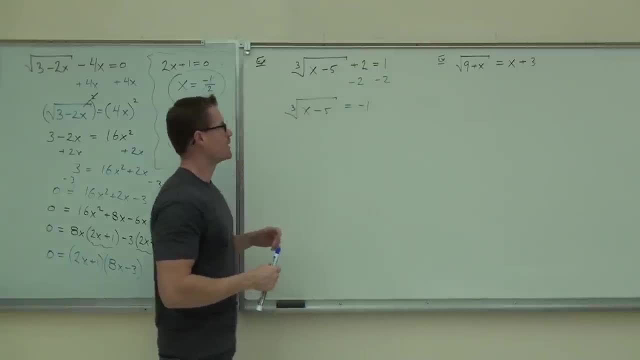 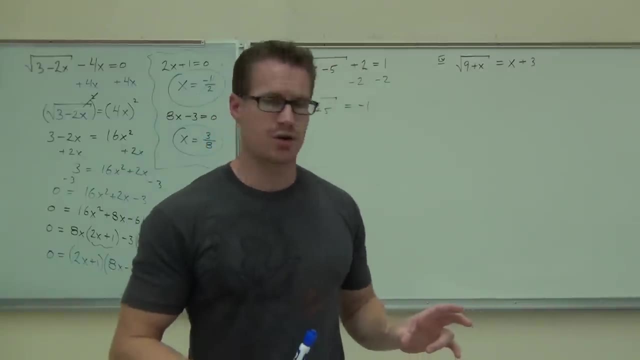 We're not there yet, But a cube root, that's not a problem. So now that we have our root isolated, you've got to look real careful at this thing. What type of root do we have? Cube root? By the way, in your homework I noticed some of you are losing the cube root when you're. 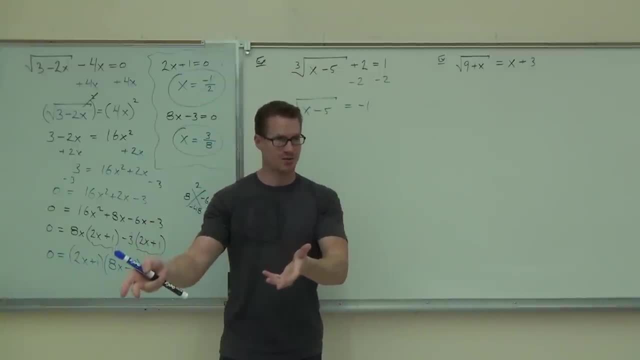 going through your problems, It's magically disappearing and you end with square roots. Be careful on that. I'm going to take points away from that on those problems. So we have a cube root here. Does a square root undo a cube? I'm sorry, does a square root undo a cube root? 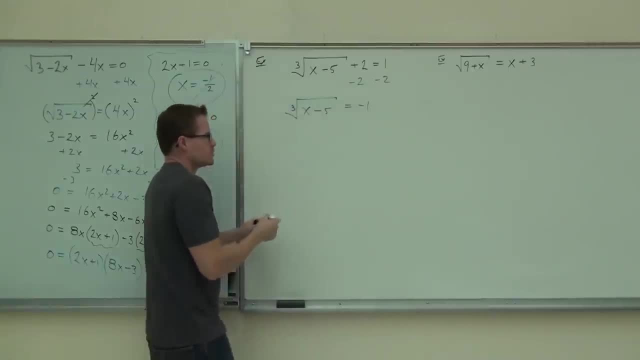 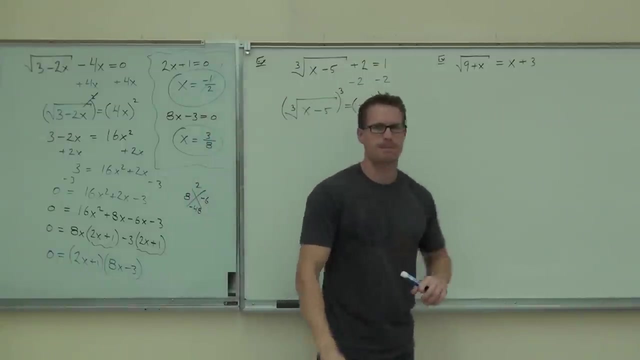 No, No, No. A square root wouldn't undo a cube. So what would undo a cube root here? A cube root, So whatever root you have, that's what power you're going to use, Not just to one side, but to both sides, just like we've been practicing. 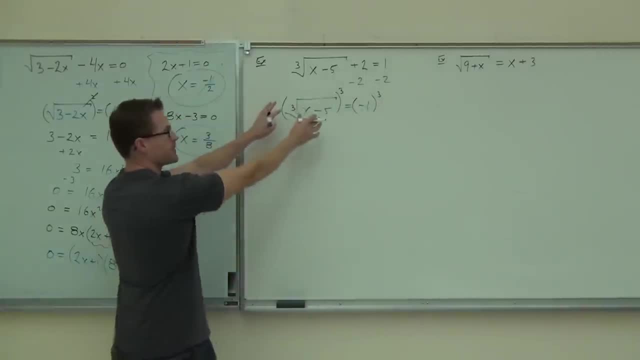 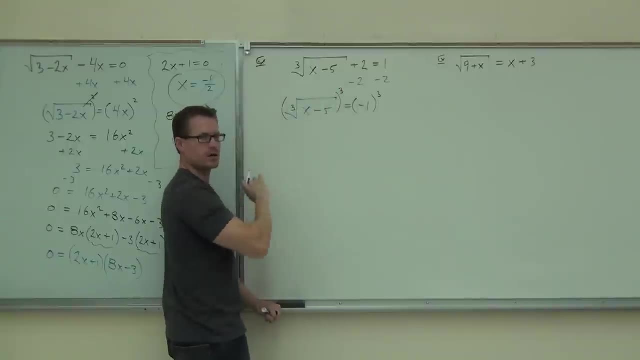 Can you please tell me what happens on the left-hand side of my equation? Okay, Does the cube and the cube root go away? They're actually inverses. You get just x minus 5.. That's kind of nice, right. It just gets rid of that. 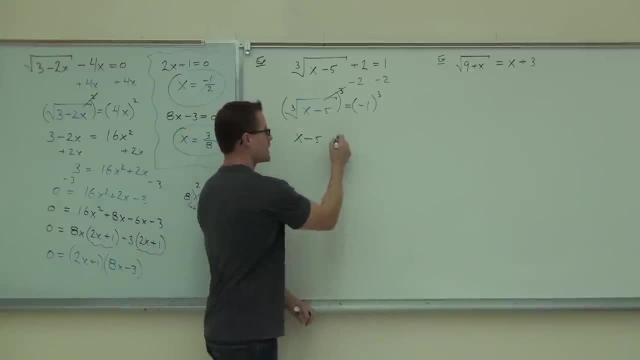 It's beautiful On the right-hand side. how much is negative? 1 to the third power, Negative 1.. Good, You're squaring it, but then you have another negative 1.. So you're going to get negative 1 times negative, 1 times negative 1.. 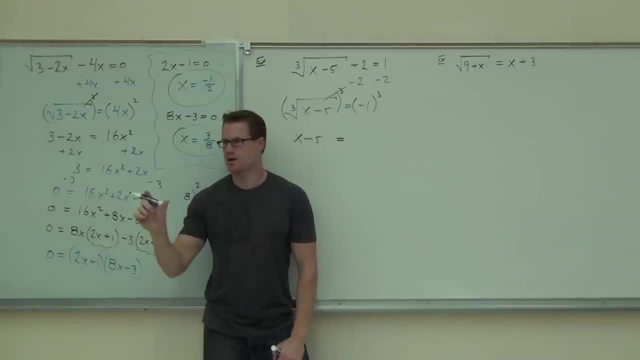 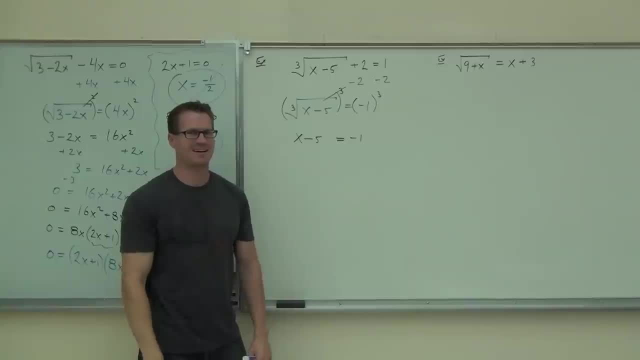 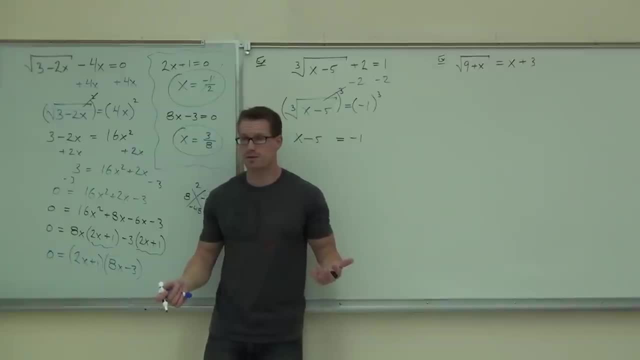 how to deal with cubes. You can't factor those cubes in this class. You don't know how to do that, So pretty much you're going to be wanting things like to the third powers, right, because those are easier, Yeah. 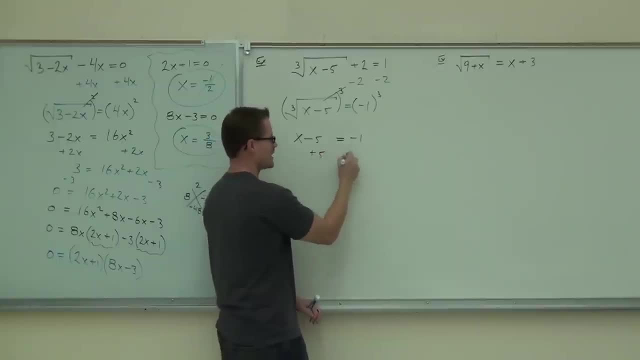 Like: oh yeah, Give me those all day. I'm just going to add 5 here. I'm going to get x equals 4.. I'm done, That's it. That's kind of cool, Thank you, Thank you. 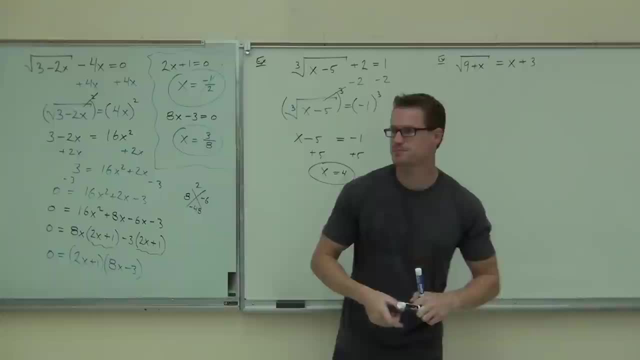 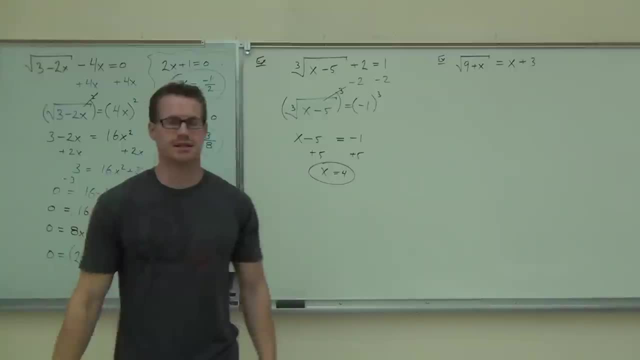 Now let's do this last one. First thing we check for is: is the root isolated? Is the root isolated here? Yes, It's all by itself, then, an equal sign. Sure, How am I going to get rid of this particular root? 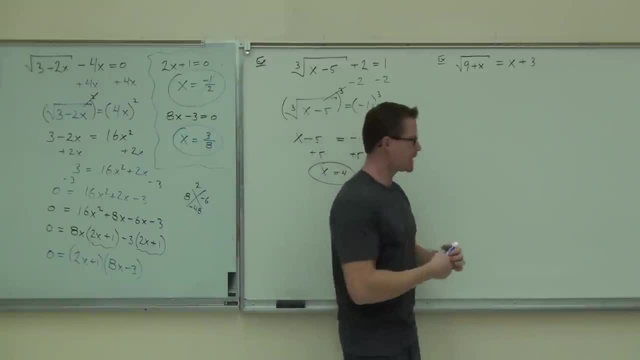 Square cube. fourth: what is it? Square Square. OK, Now again. why we've been practicing this is, of course, I'm going to square the left hand side. Do I also have to square the right hand side? 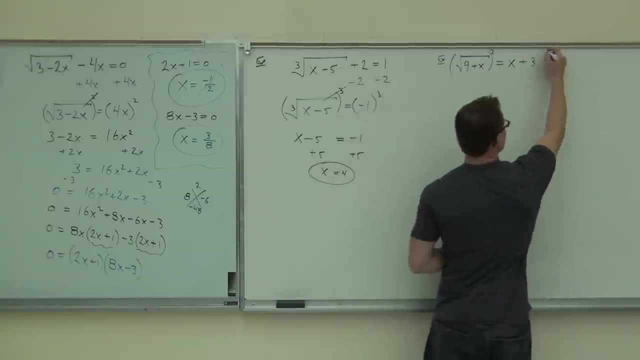 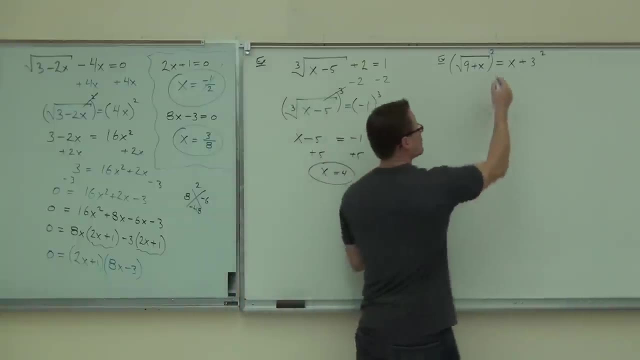 Yes, Absolutely. And you know what I can't just do that That squares the three, But that doesn't square the whole side. What do I need? Oh, OK, OK, Is that OK with you? Yeah, Sure. 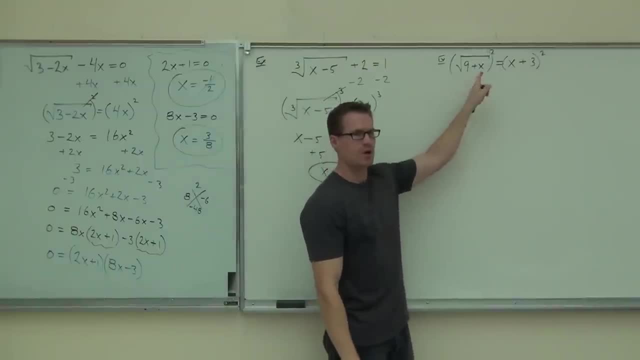 That's not a problem. What happens? let's go slowly through this one. What happens on the left hand side? What are you going to get out of that? That's the stuff we've been practicing, no problem. Now, on the right hand side, please, I'm begging you, don't just give me x squared plus nine. 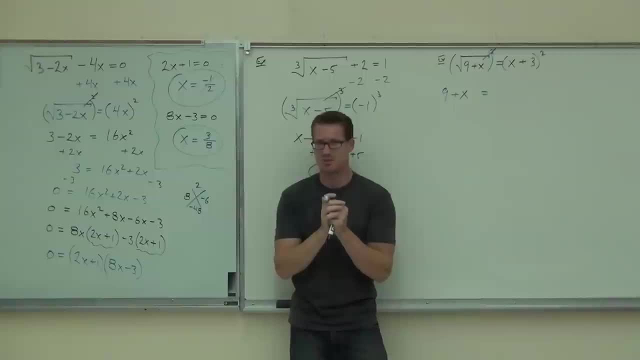 No problem, Please don't give me x squared plus nine, Do you promise? Yeah, Do you promise, Because I'm going to start crying if you give me that Let's weigh from homework, I mean. 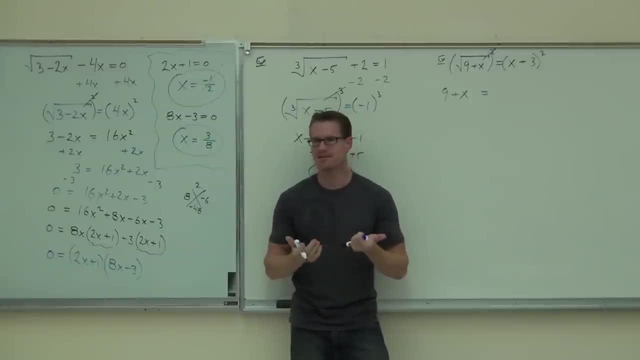 I mean, is going to make me sad, hurt my feelings? Is that going to lead you to dreams Too late? just kidding, That was last semester. Last semester led me to drink. Oh gosh, Wow. 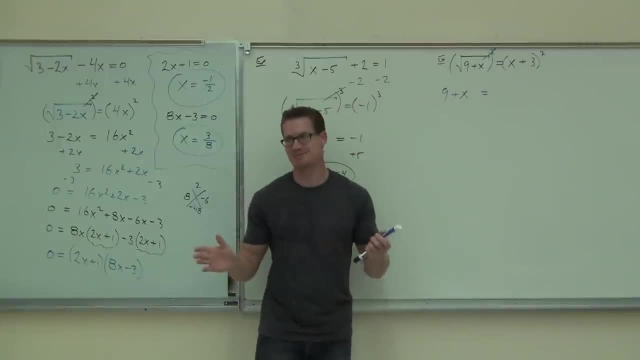 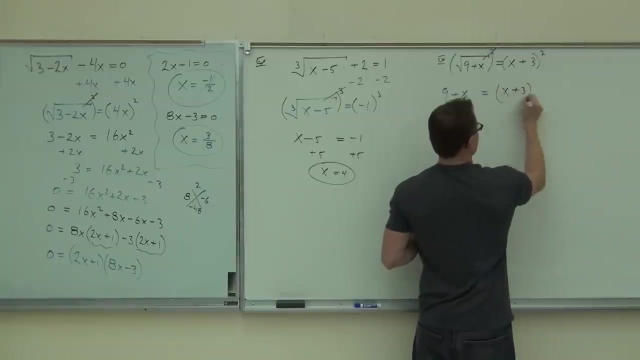 Just kidding, Okay. so here of course we have something, we have something squared That really means x plus 3 times x plus 3.. You have to write it like that because you're going to miss the middle term if you don't. 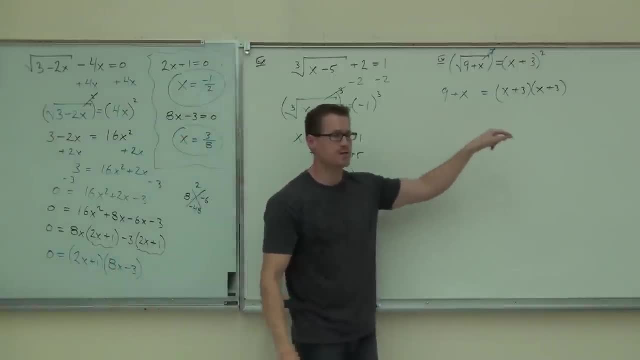 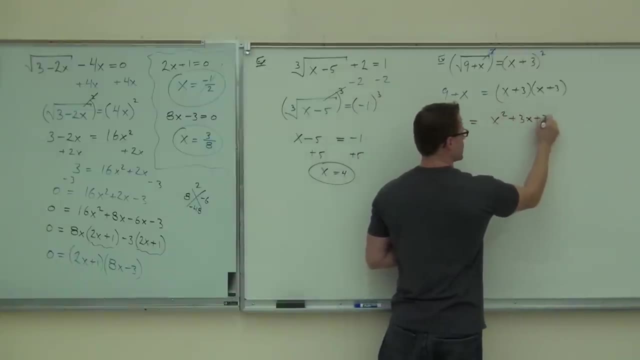 Yes, you are going to get x squared. Yes, you are going to get a 9.. You're also going to get 6x And we're going to see that when we do 9 plus x equals if you distribute x squared plus 3x, plus 3x plus 9.. 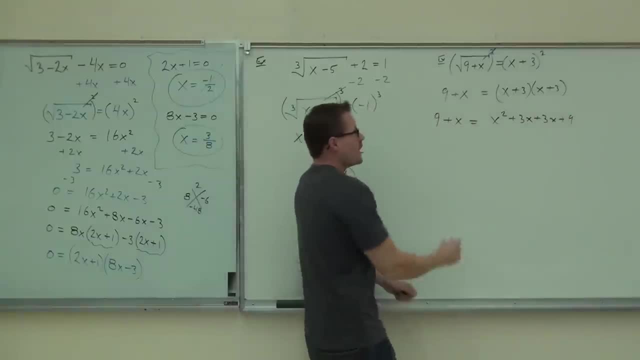 That middle term is what you would be forgetting if you did x squared plus 9.. Of course, we'll combine like terms. I'm not doing anything that you haven't seen before. In fact, after this step, this is old news. 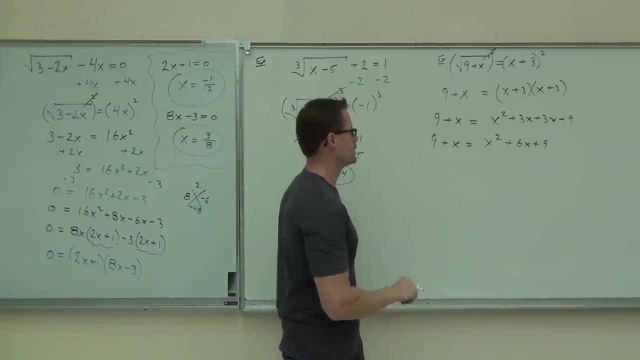 You've seen that before. You've had problems like that in your review. Oh my Well, what now You're going to move it all to one side? OK, Why someone else? do I move it all to one side? 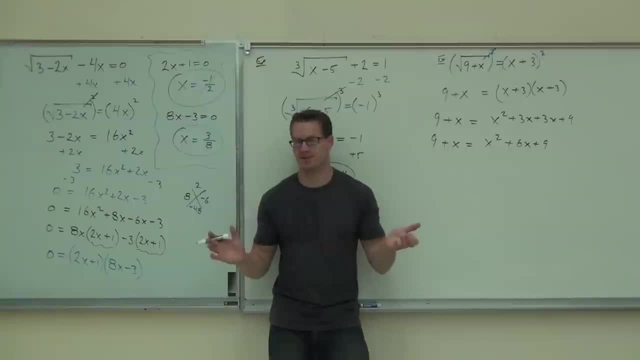 Because you can't have x's all over the place. OK, I can't have x's all over the place, For sure They're all over the place. Also, there's one thing that clues you in, that I have to move everything to one side and zero to the other side. 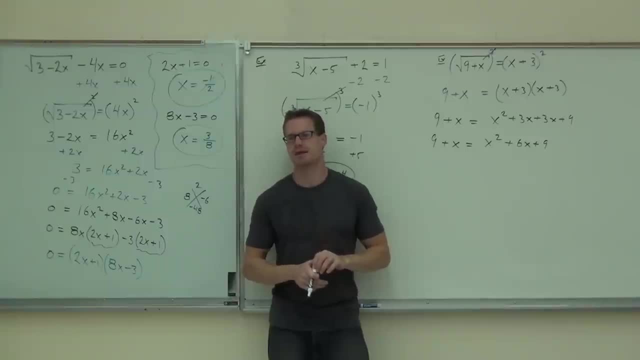 And Jacob, you said: what was it? You had the square. Yeah, It's got the x squared. That says everything on one side, zero on the other side. Now I don't want to move all this stuff because the x squared is positive. 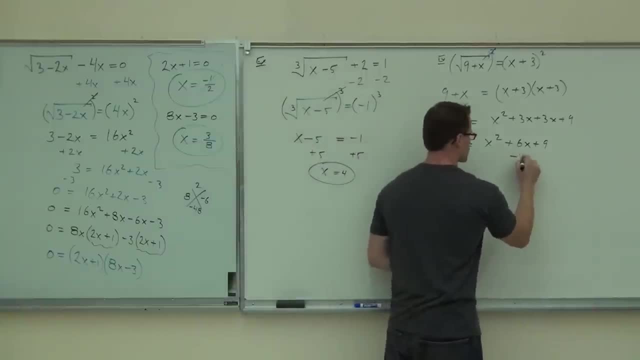 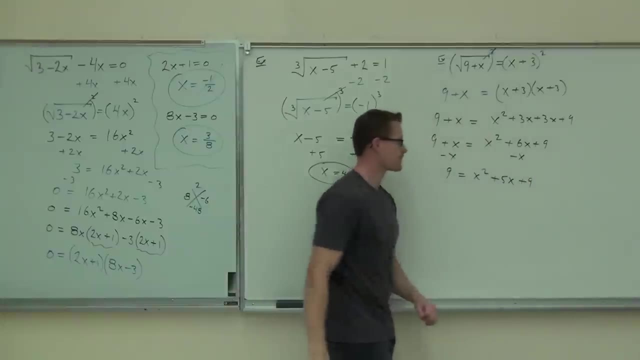 I want to move this stuff, So I'm going to subtract x from both sides. I'll get 9 equals x squared plus 5x plus 9.. Hey, is this good enough for you? Is that good enough? Should you be factoring this right here? 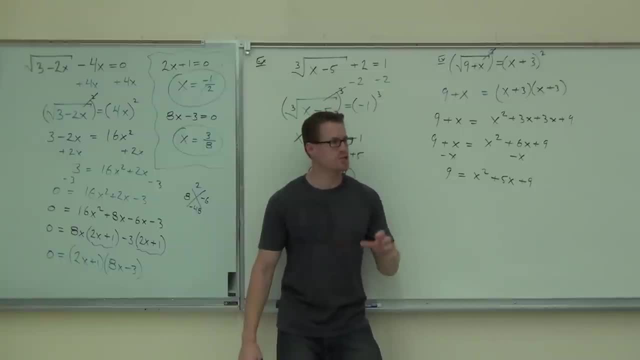 No, No, definitely not. I do need a zero. That's the only way the zero product property works by a zero. So you've got to go one more step. What's that last step we're going to do? Subtract 9.. 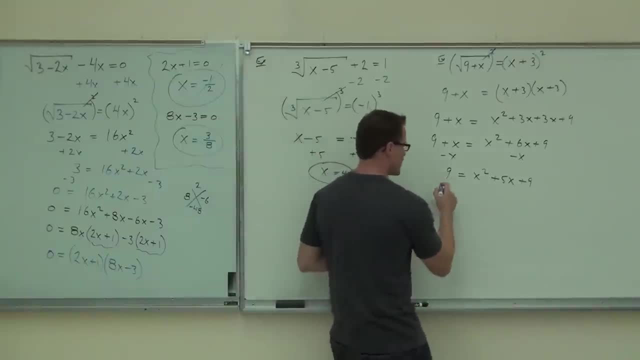 Now something kind of interesting happens here. I put this up here for a reason. That way you'd see this: If you subtract 9,, you're going to get 9.. You're going to get zero equals x squared plus 5x, but there's no 9 anymore. 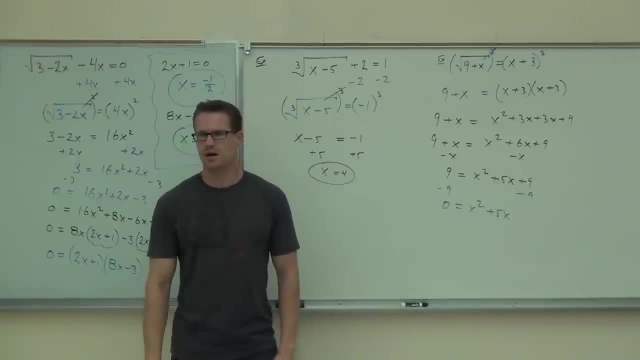 Those are gone. Can you still factor it? Yes, Yeah, Do you need a diamond problem? No, What you'd actually look for is the greatest common factor. That's the first thing you really should be looking for in any case. So when you look at this diamond problem- no, 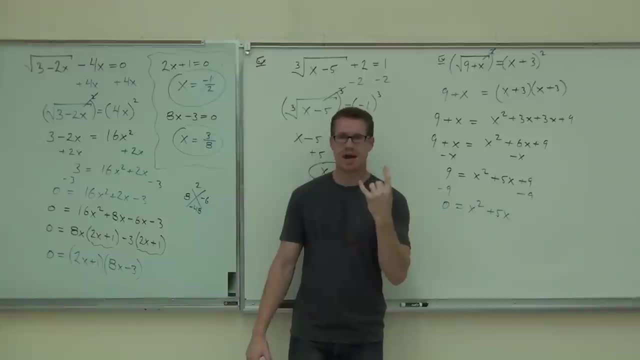 It's not even three terms, There's only two terms, Only options you have for two terms are a difference of squares, which this is definitely not, or a greatest common factor, And we have one. What factors out of both of those in terms? 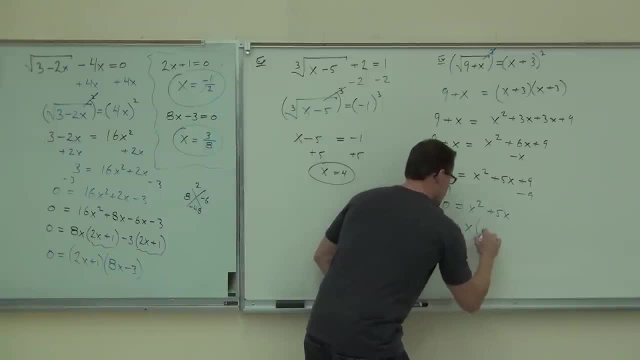 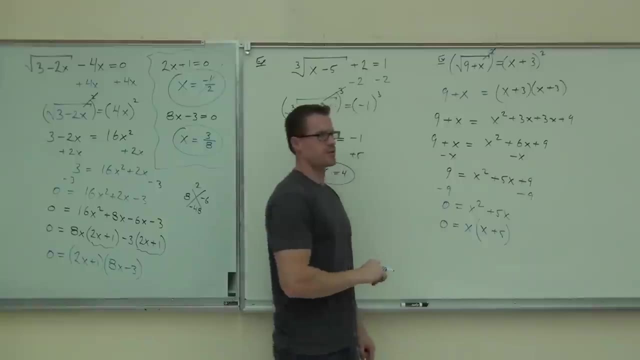 Factor next. Zero equals x times. if you factor the x, you get how much x plus 5 plus 5.. Yeah, not x squared plus 5. You get x plus 5.. You factored the x away. You divided out that x. 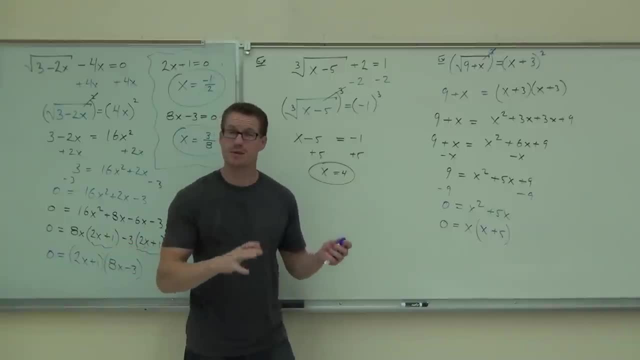 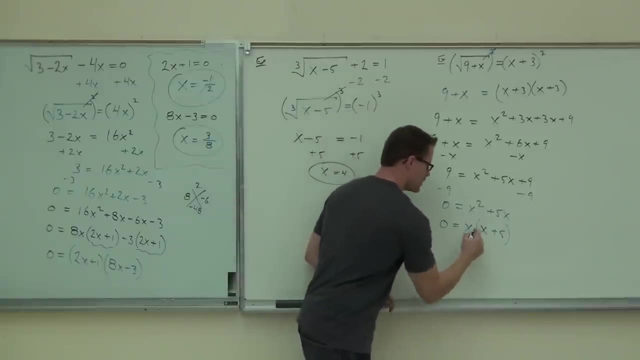 Now I've got to tell you the zero property still works. It works just fine. In fact it's a little bit easier. It says you have two things that are multiplied together that equal zero. What that says is that both of those things have 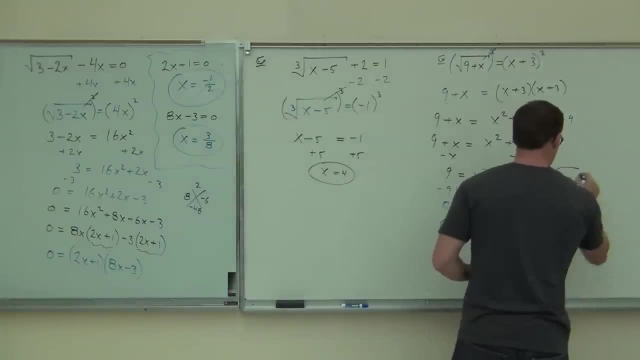 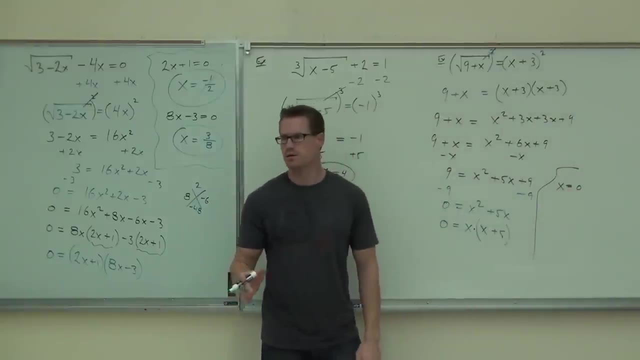 to be multiplied, They have to equal zero, So we would set the first one equal to zero. We get x equals zero. That's kind of nice, because there's actually no work there at all. You get x equals zero, you're done. 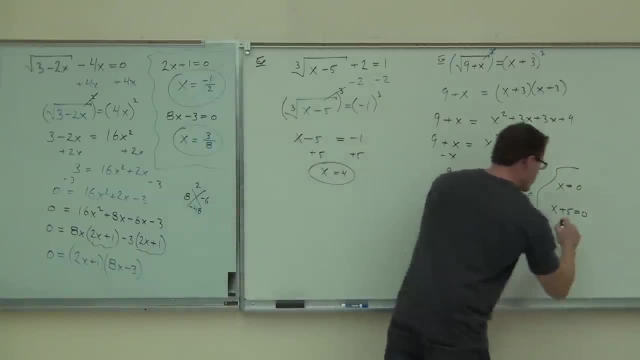 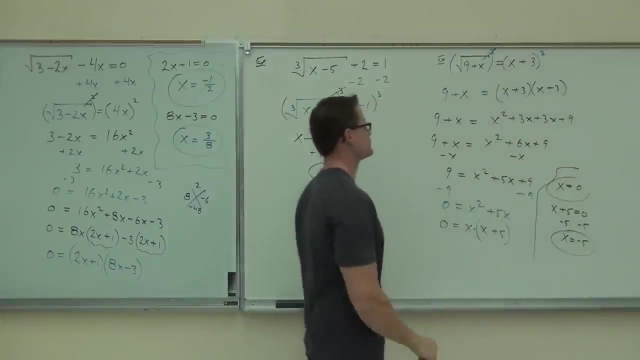 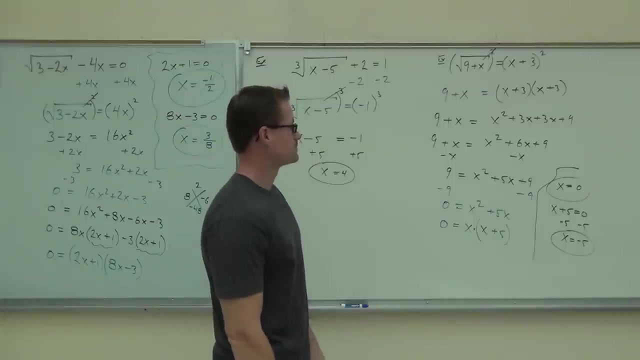 Last one. we have to do just a bit of work, for We have both of these things equal to zero. Subtract 5 from both sides, You get x equals negative 5.. And you've got to check your solutions here. You've got to check. 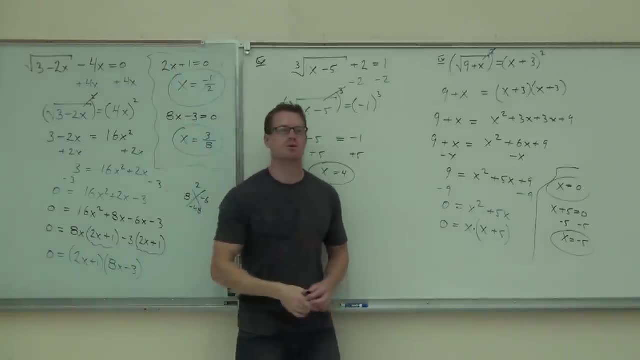 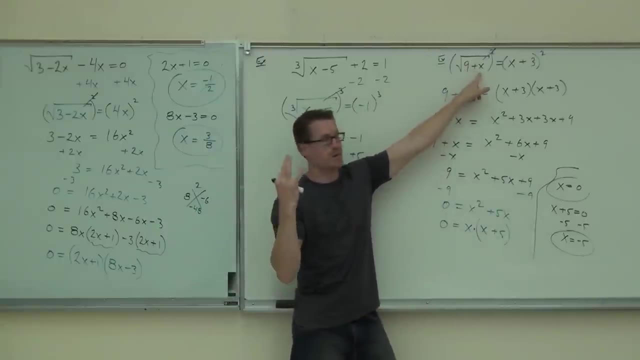 First thing, how many of you feel okay getting that far? Check the zero with me. If we check zero, we get 9 plus 0.. How much is that Negative? Square root of 9 is Negative. We've got a 3 on this side. 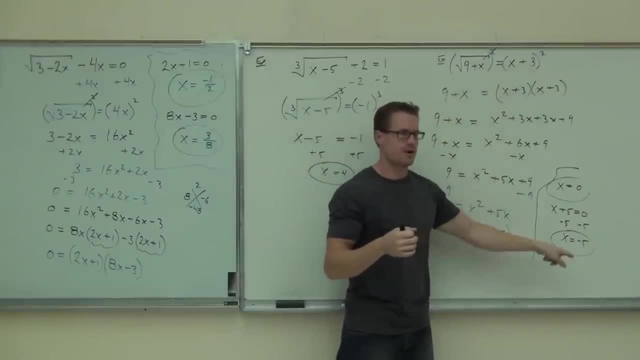 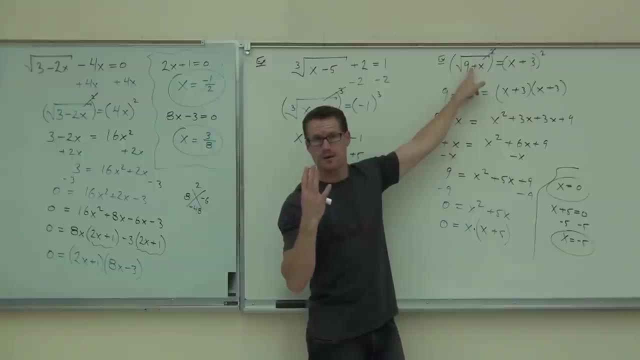 Zero plus 3 is 3. It works. Check the negative 5.. If you check the negative 5,, 9 plus negative 5, that's really 9 minus 5.. That gives you 4.. The square root of 4 is: 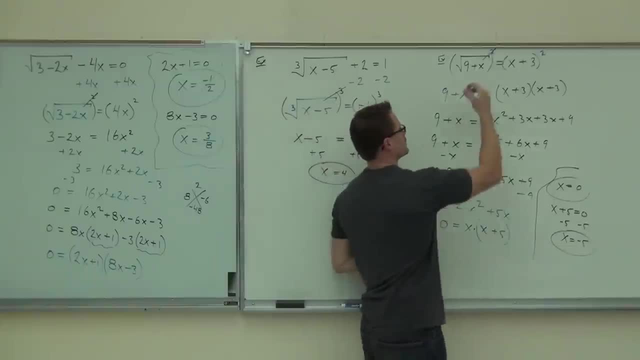 Zero. Now check the right-hand side. Notice we've got a 2. when you plug in that number, That would be negative 5, right? What's negative? 5 plus 3? Negative, Did that work? Yeah, Same situation that we have over here. 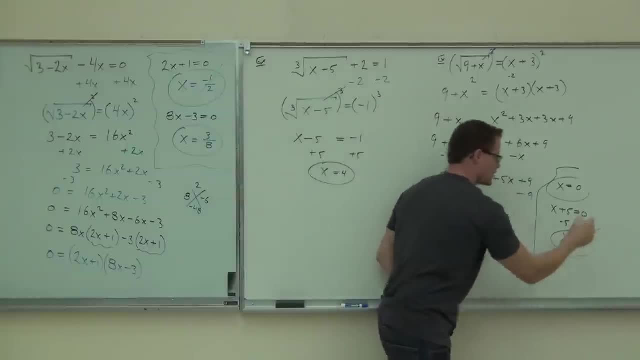 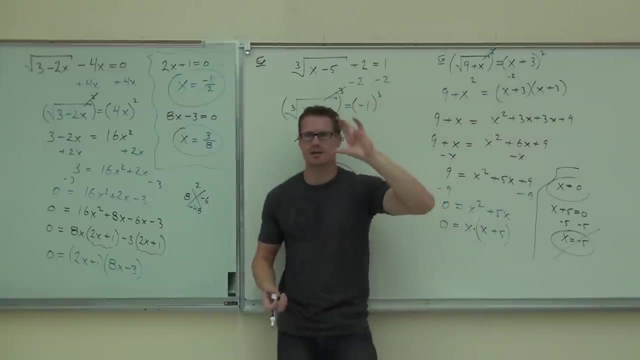 Basically the same situation we had over there. This expression or that solution is not going to work in our problem, So we cross it out, Because you get 2 equals negative, 2, again, that square is making Positive. Some false solution is positive, so it looks like it works. 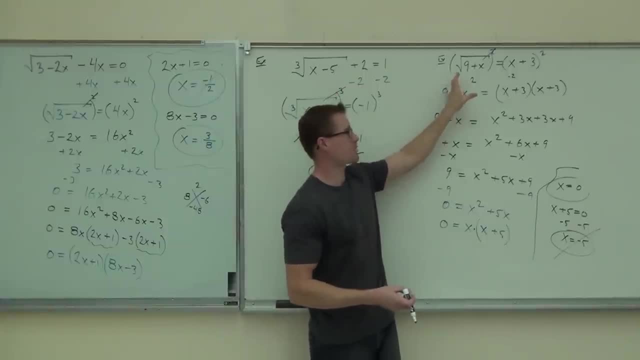 but it doesn't work Because that square, the square root, kind of gives a false sense of security. there It says you're squaring it and making negative as a positive. It's going to look like it works, but it doesn't. Did you guys kind of see the point there? 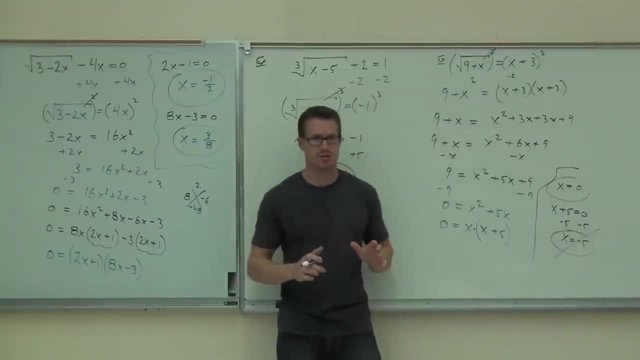 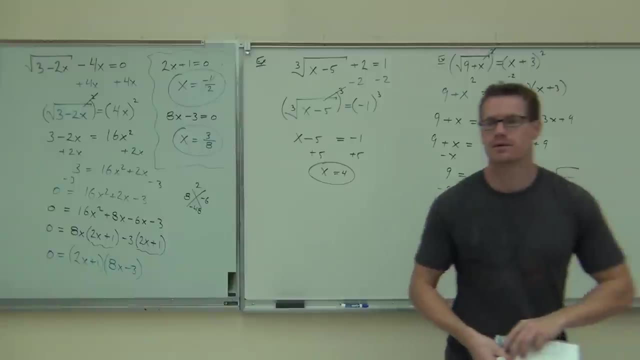 So you really do have to check. you've seen this twice now. You really do have to check your solutions because sometimes you're going to get those false solutions. that's not a good thing. So if we check that solution in the original problem before we put the parentheses- 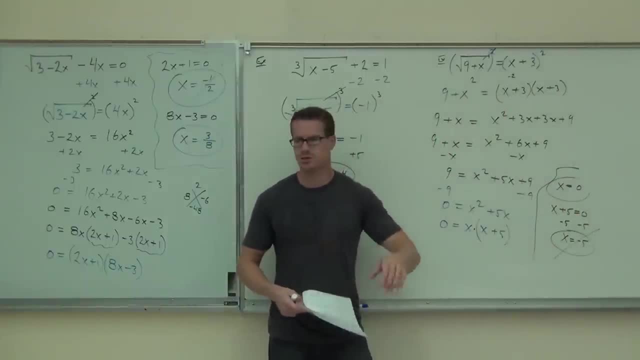 Absolutely. You have the very original one. That's how you check. all solutions is the original equation. You, okay, so far Got two more things to talk about. The first one: we're not going to go through this all the way down. 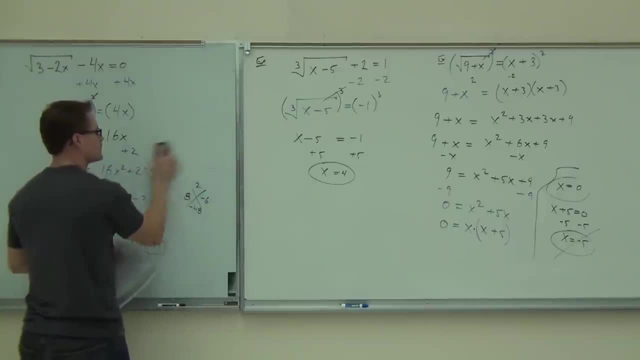 I want to show you the idea here. I'll give you the first step. That way you don't get completely lost on your homework. But it is the same idea- And then we're going to talk about something called the Pythagorean Theorem- that we can apply this to. 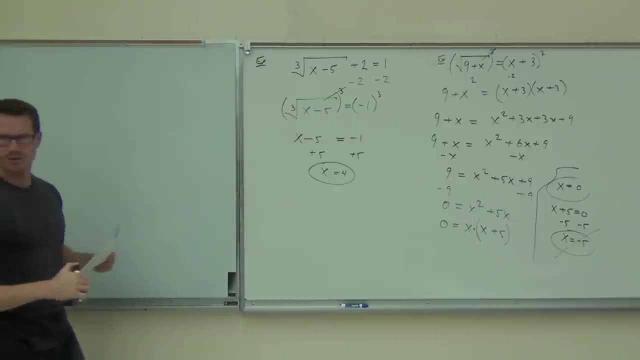 If you've never heard of that before. not really too much of a part of it. Actually, probably most of you have heard of it in some way, shape or form. But we'll talk about it in relation to this material. Oh my, 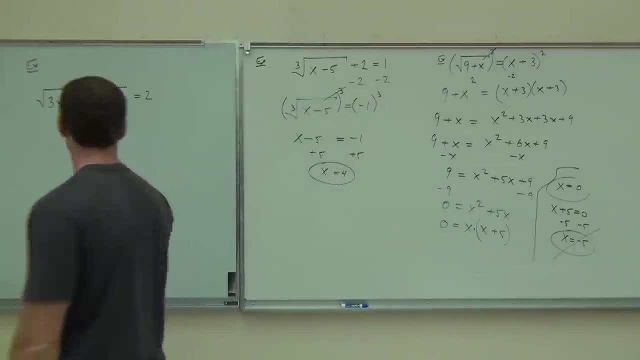 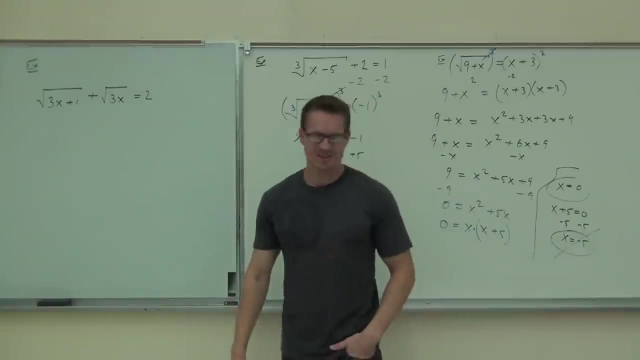 What, What Are you crazy? Oh, my goodness, What in the world are you trying to do to us? Leonard Must have been drinking before class, or something That's only on Fridays, Just kidding. Got a whole lot to look forward to tomorrow. I'll tell you that. 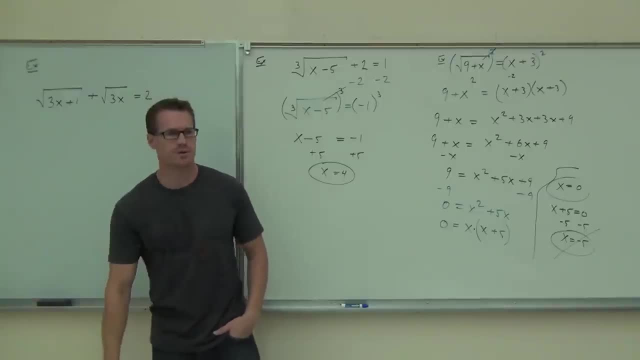 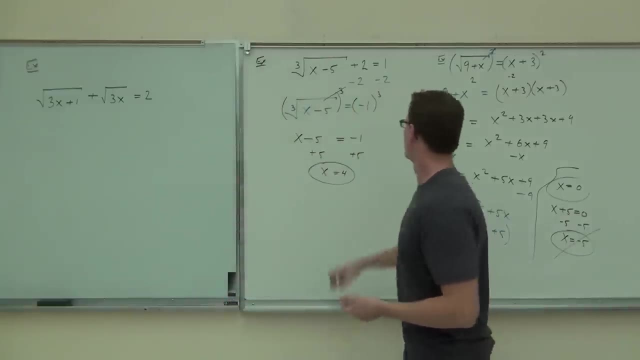 Just kidding. Okay, so we don't just have one square root, We don't just have one root, We have two roots now. Now, the idea was before: Isolate your root. That's why we subtracted the two. This was already isolated. 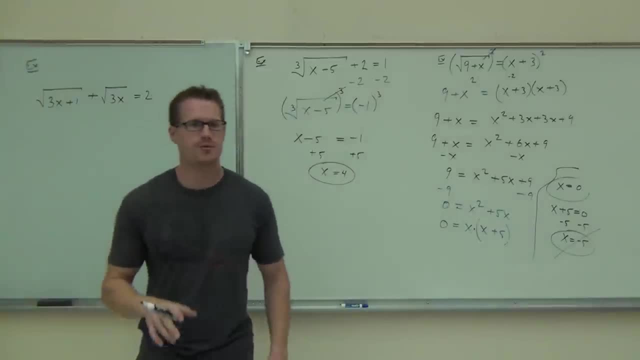 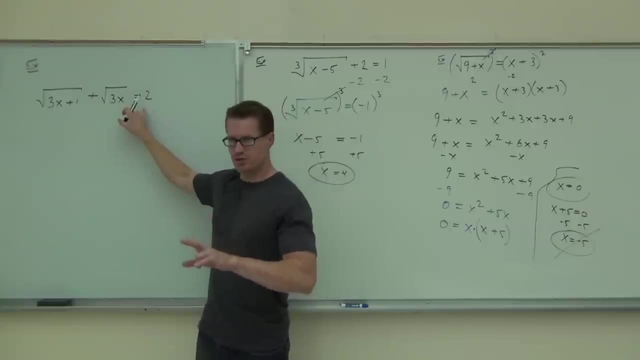 That was great for us. You're going to do the same thing here. Only, unfortunately, you can't isolate both roots because of that nasty two. Now, if that two wasn't there, this problem would work out just fine. You'd subtract one of these roots. 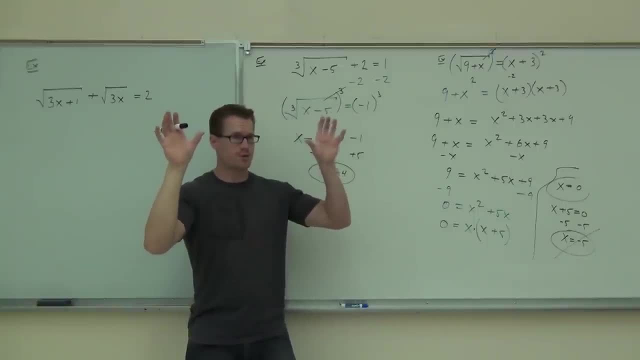 You'd get a root on both sides. You'd square both sides. Both the roots would go away. You with me. In fact, even the negative would go away when you subtract because you're squaring the negative. That would be an easy problem. 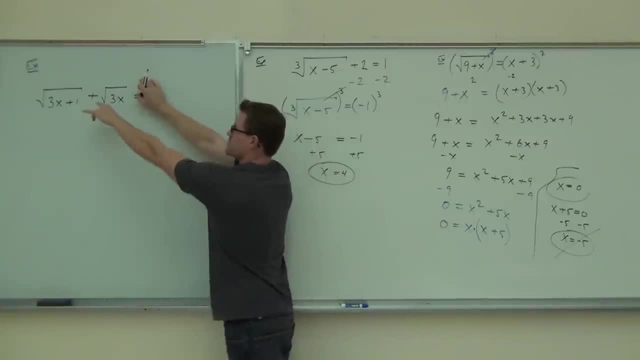 Are you with me on that? Yes, So if you're going to do this, you're going to have to do this. If the two wasn't there, you'd subtract this one, You'd square both sides. You would get 3x plus 1 equals 3x. 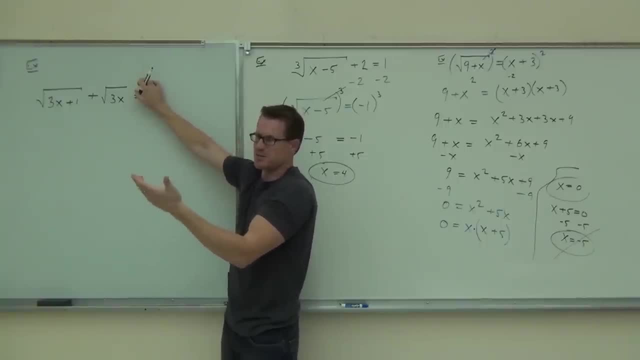 That would actually be a problem because when you subtract the 3x, you'd get 1 equals 0. There would be no solution to that problem, But that's the idea. That would be the idea there. Are you with me on the idea? 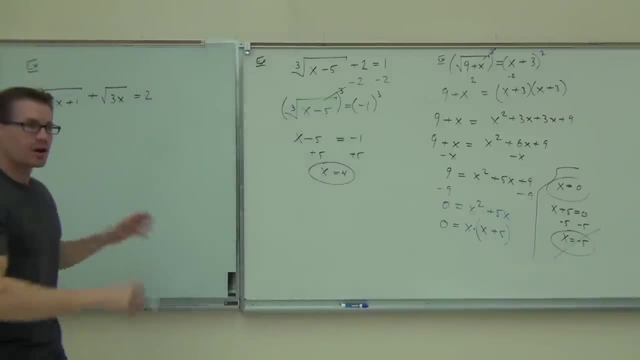 Now, with the two we have a different situation. We would isolate one of the roots. I'm going to choose to isolate this one, which means let's subtract the entire square root of 3x from both sides. You get the square root of 3x plus 1 equals 2 minus the square root of 3x. 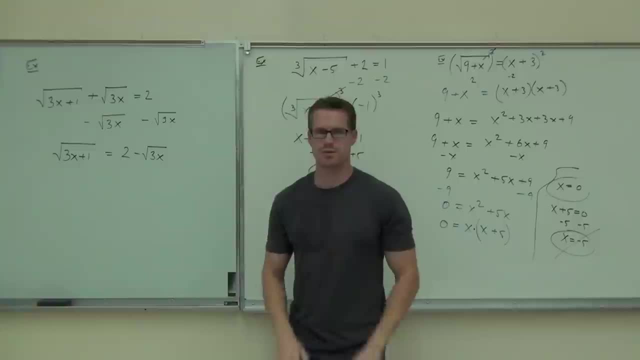 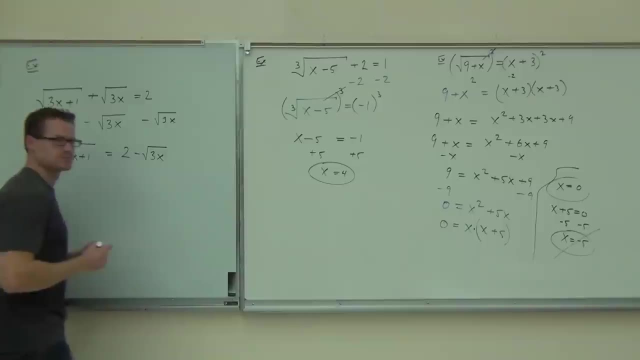 So far, so good. Right, We've isolated one of the roots. It's impossible to isolate both of them. Now, what power gets rid of our square root? Square root- You're going to square both sides, That doesn't just mean this one. 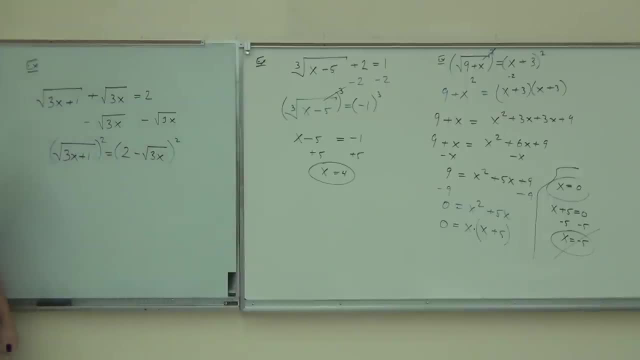 That means this entire side over here, that entire side. Now, while this simplifies out and you get 3x plus 1, I want you to notice that this should look very familiar to you. That's like your homework was a couple sections ago. 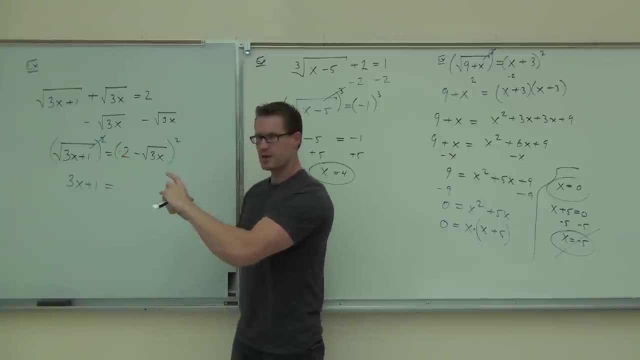 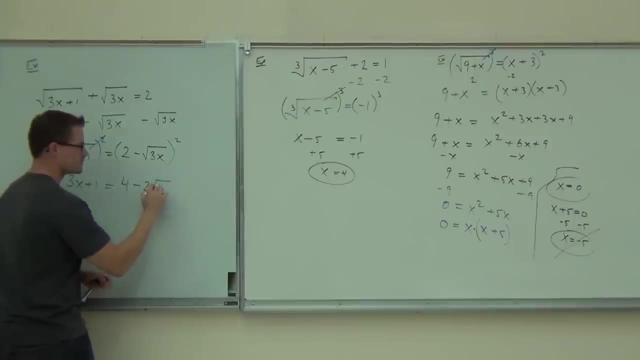 When you have this thing, you'd write it out, Follow me along here, But what you would get is 4 minus 2 root 3x. You're going to have to show. I'm doing this in my head. You would have to show some work on that thing. 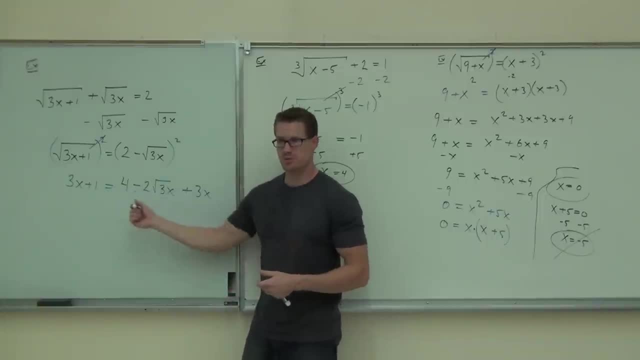 You would write it out, You would distribute it, You'd combine like terms and that's exactly what you would get. Do you notice how we still have a root? At this point, you'd isolate your root and do the whole thing over again. 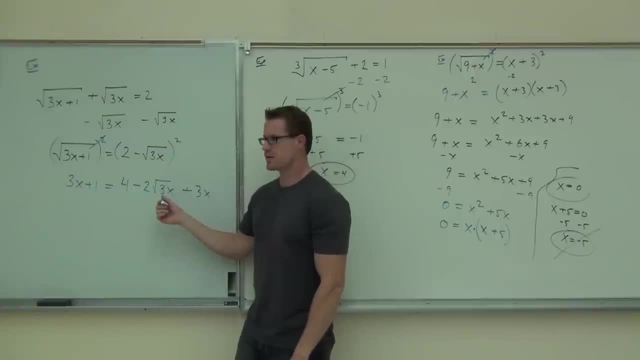 Okay, I'm not expecting you to do this on a test. Okay, This is a little bit advanced for us to do this, but this is the idea: Isolate one root, square both sides. You're going to get another root. 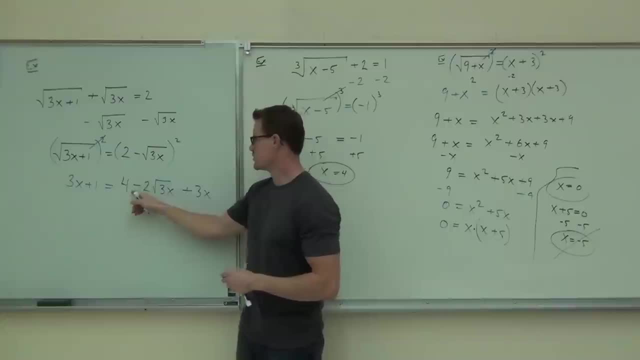 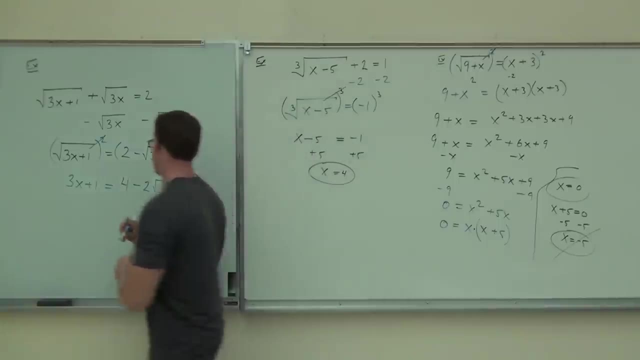 Isolate that root square both sides again. So in this case you would subtract 4.. You would subtract 3x. Oh, that one's going to be kind of nice actually. Let me make sure I did that right. It's 2 minus. 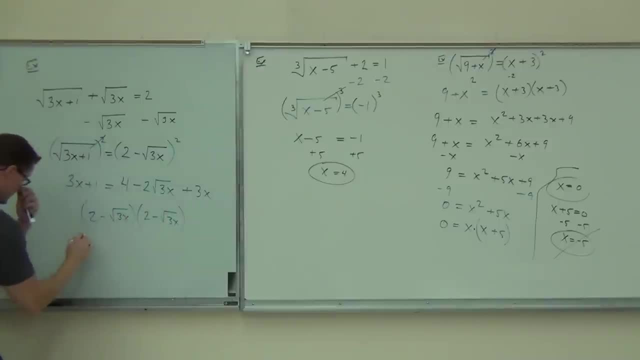 I might have made a mistake: See 4 minus 2 root 3x. No, I did it right. Yeah, those 3x's are going to be gone. That's isolated. That's actually not a bad problem at all. 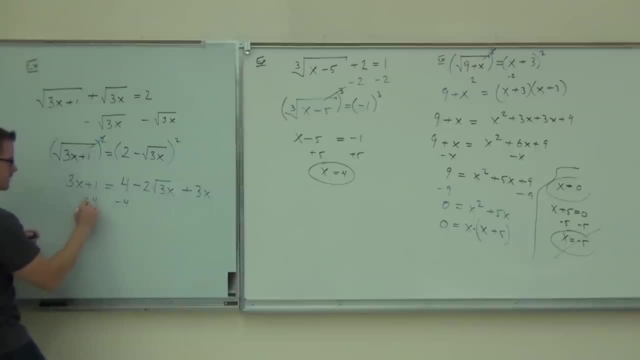 I'm going to keep going on that. So you get down to here. You'd subtract the 4. You get 3x minus 3 equals negative 2 root 3x plus 3x. If you subtract the 3x's, those things are gone. 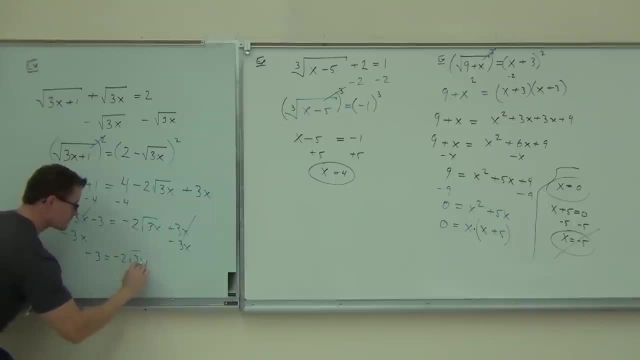 Negative 3 equals negative 2 root 3x. Before you square both sides, divide by negative 2.. And you would get positive 3 halves equals the square root of 3x. At this point, that's where you square both sides. 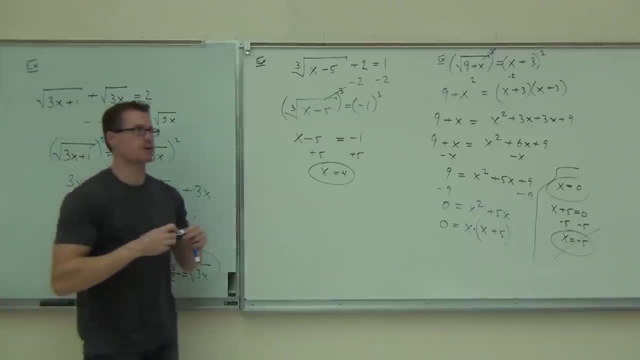 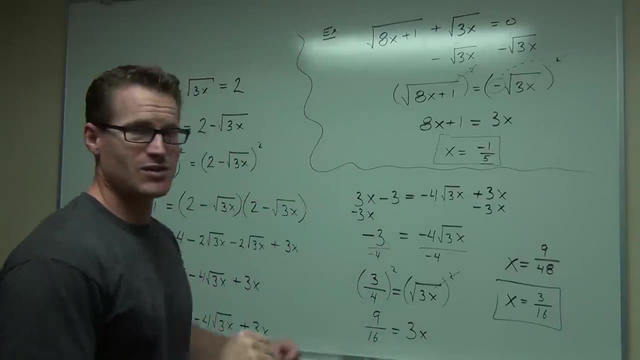 So from right here you should be able to go on that square both sides and solve for x. Okay, so actually there's a mistake on your previous problem Here. if you want to check this one out again, I made a mistake right down here. 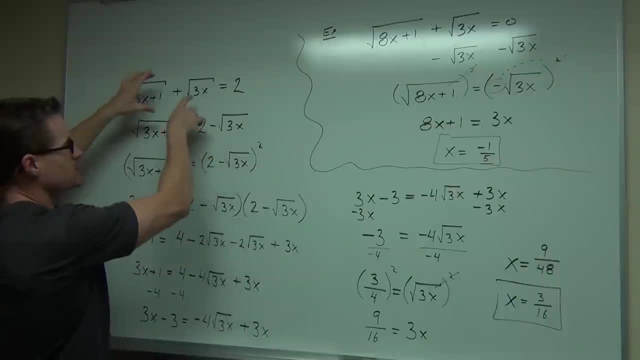 on this area. Of course, we're going to certainly subtract your square root of 3x And we're going to square both sides. That gets rid of our square root here. That distributes here. But watch what happens Here: 3x plus 1, that stays the same. 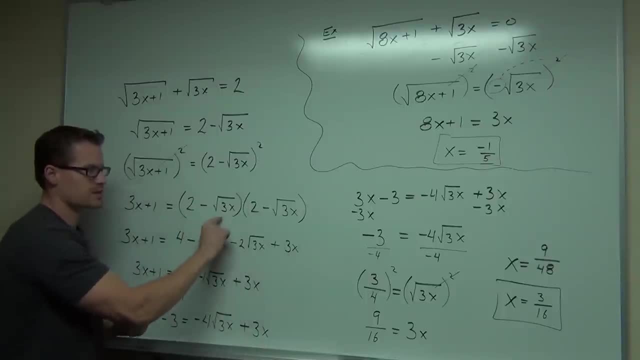 Here you're going to get the 4. You're going to get minus 2 root 3x, another minus 2 root 3x and then plus 3x. This is correct. I think I had this in class for you. 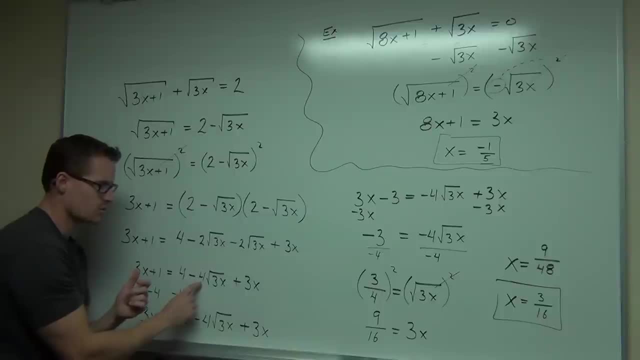 However, when you combine these, I believe I have a 2 root 3x. It should be a 4 root 3x. That's the correct version of this problem. After that, of course, we're going to subtract 4 from both sides. 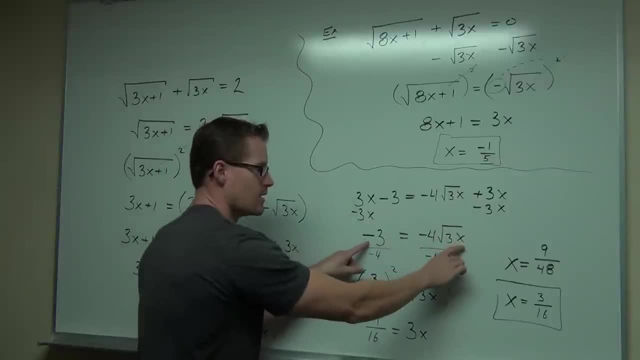 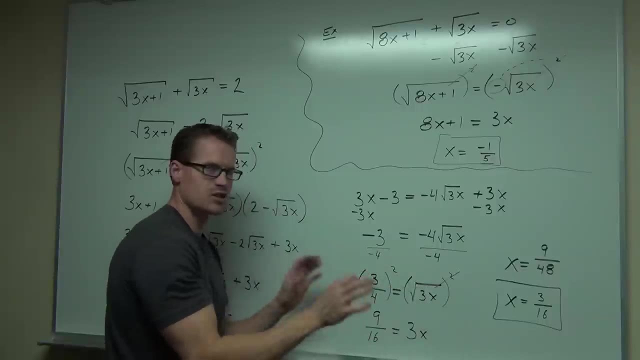 subtract 3x from both sides. We're going to get down to this step. Instead of the 2, you're going to have the negative 4.. Divide by negative 4. That becomes positive. We'd square both sides just like we did. 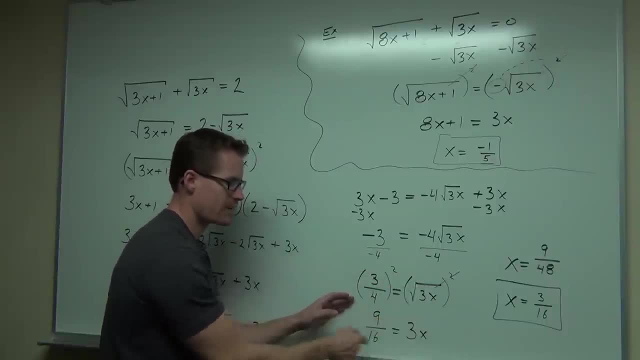 But we're going to get 9. 16ths equals 3x. If you divide both sides by 3, we get 9 over 48, reducing to 3 16ths. That's the correct answer. So check this out one more time. 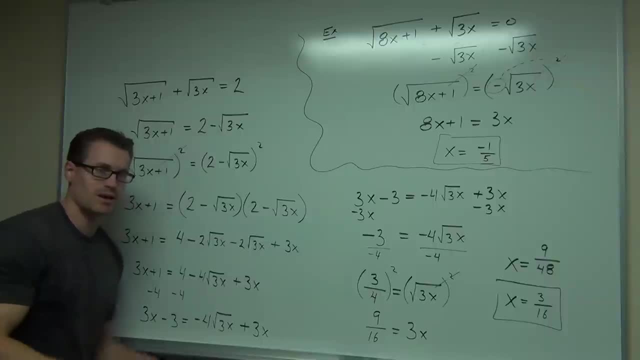 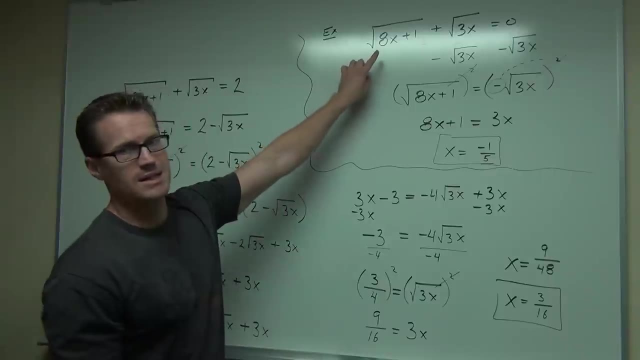 Make sure that right here you combine like terms properly, unlike I did My bad. Also one more example for you, if you want to check this one out. This is what I was talking about, but did not give you an example in class. 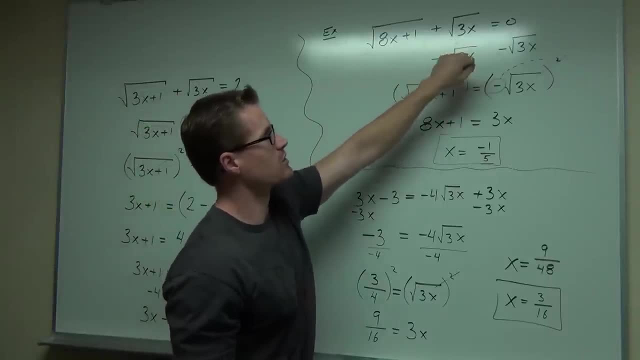 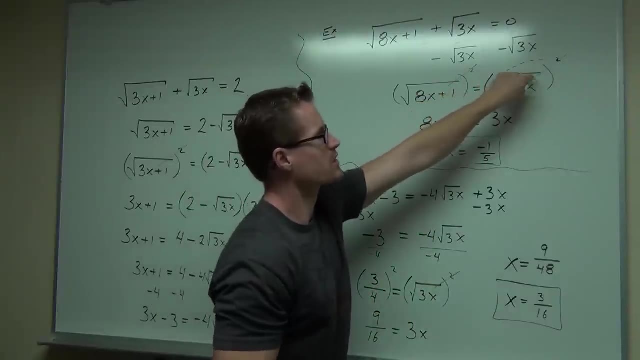 If you go ahead and look at this and we get a square root plus a square root equals 0. Isolate your square root. Square both sides. We do get this. when the square roots simplify, This negative also gets squared. That's why you don't have a negative right here. 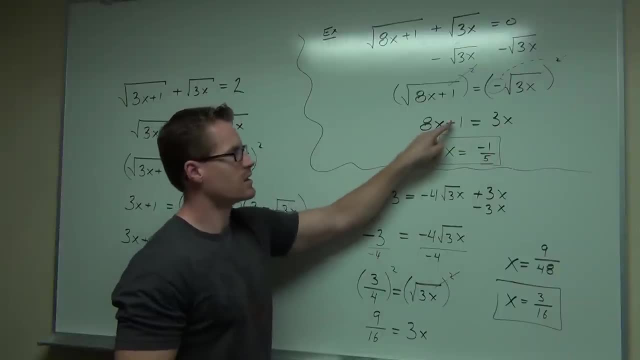 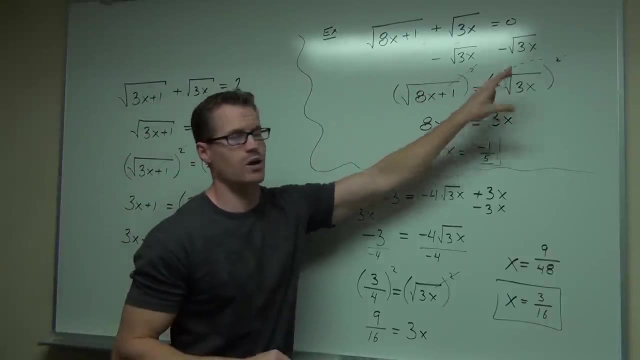 You get a positive. After that you subtract 3x, Subtract 3x, Subtract 1.. Divide by 5 and your answer will be negative: 1- 5th, I wanted you to see what happens when I have a square root equal to a square root. 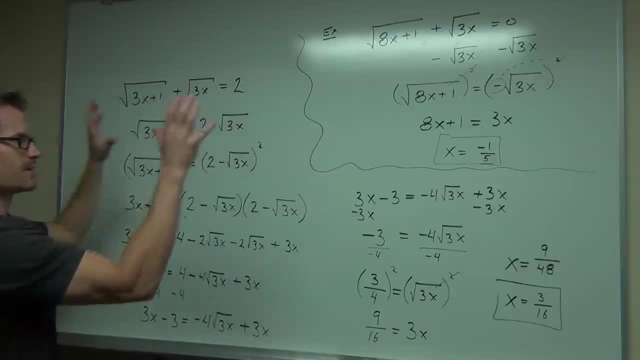 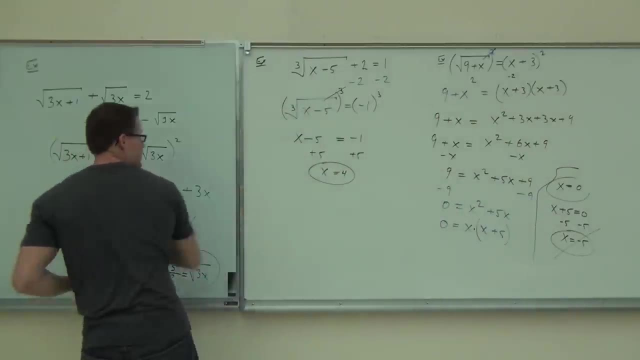 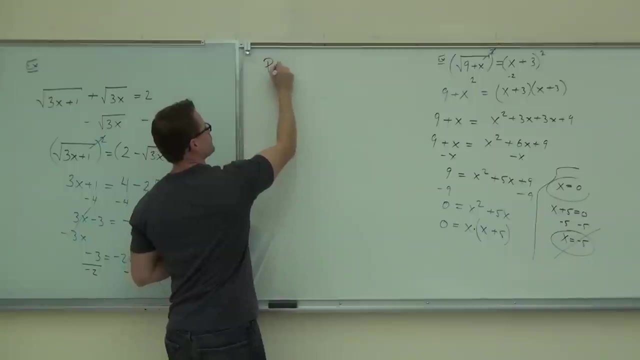 If we get a square, both sides, the square roots go away. So that's the correct answer here, and another example for you right there. Okay, the last thing we've got to talk about in our section here, Something called the Pythagorean theorem. 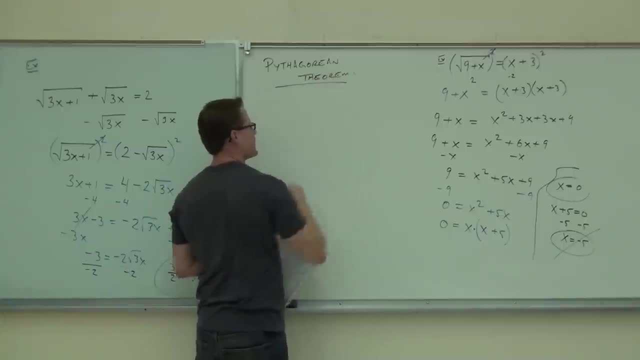 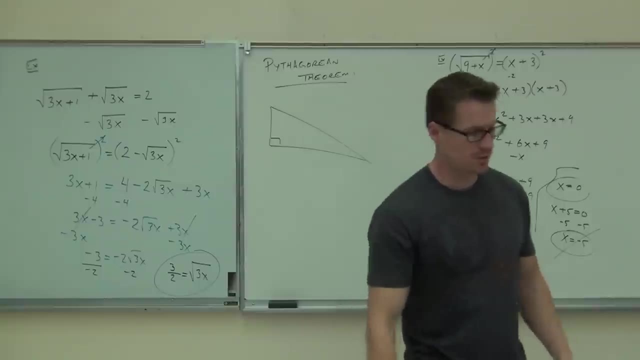 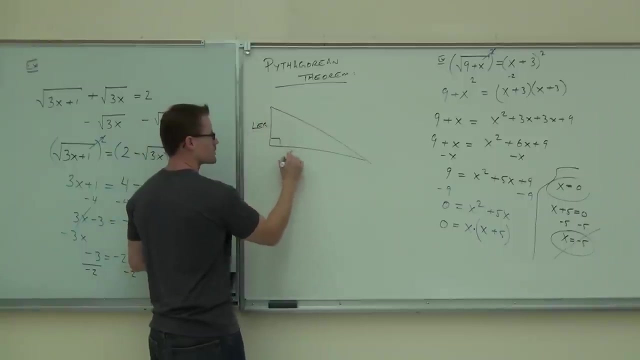 Pythagorean theorem works on something called a right triangle. A right triangle, basically, is a triangle with one 90 degree angle. We have special names for these sides, though. This one's called a leg, This one's also a leg, And this one- do you know the name of that one? 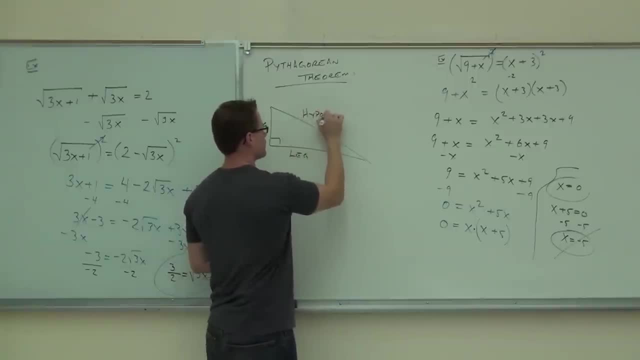 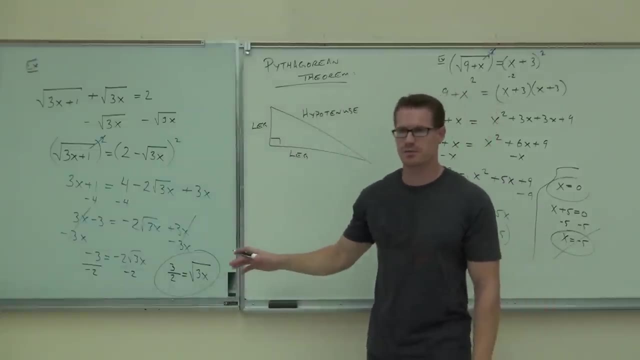 Hypotenuse, Hypotenuse, that's right. Bless you. Here's what the Pythagorean theorem says. Pythagoras is an old guy. They actually killed him. They murdered this guy a long time ago because he said that not all numbers are rational. 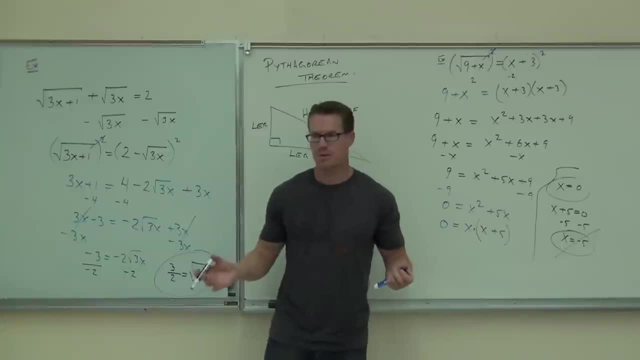 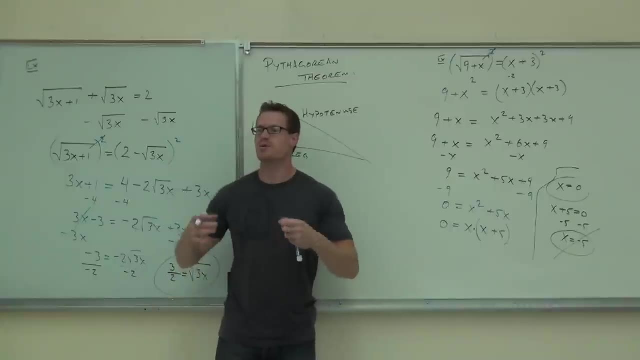 And these people? their religion was based on numbers, I'm not even kidding you. So they would like do all the crazy stuff with numbers. So they said, oh, every number can be represented as a fraction. This guy goes: no, it can't. 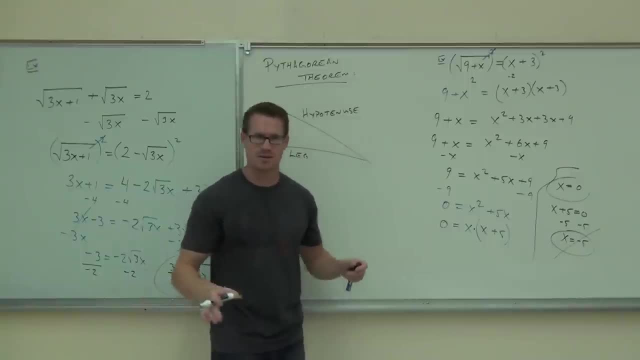 So they killed him because it ruined their whole religion. All right, That was the whole idea. So, anyway, Pythagoras, this guy- it's actually his followers who made this up. But, Pythagoras, The Pythagorean theorem says: if you take a leg and you square it, plus a leg and you 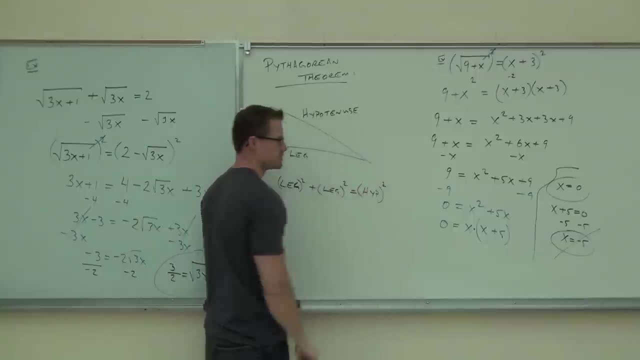 square it, it's equal to the hypotenuse squared. That's the whole thing. That's the whole thing. What this allows you to do is, if you have some missing sides for a triangle, you can actually solve them. For instance, if you knew this was 9 and this was 6 and this was x. 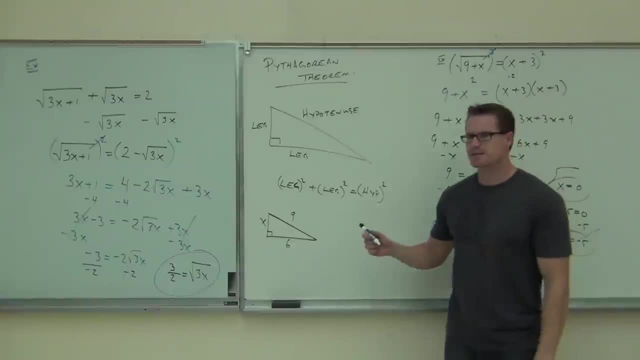 Can you tell me what one of the legs is here? 6 is a leg, Very good, Someone else? what's the other leg And what is the hypotenuse? Give me a little head nod if you're OK on those names. 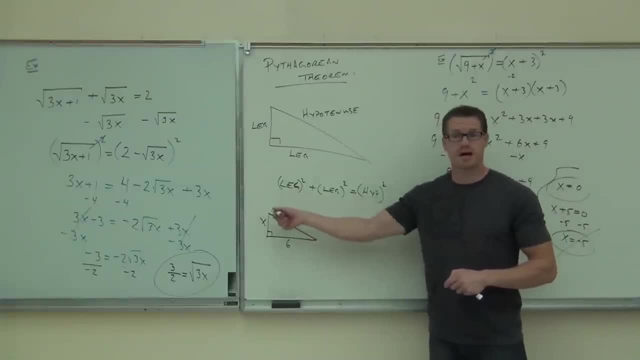 This is a leg and that's a leg and that's a hypotenuse. The longest side opposite the 90 degree angle is the hypotenuse. As long as you take this and set up in this equation, you can solve it. So if our leg is x, we would get x squared. 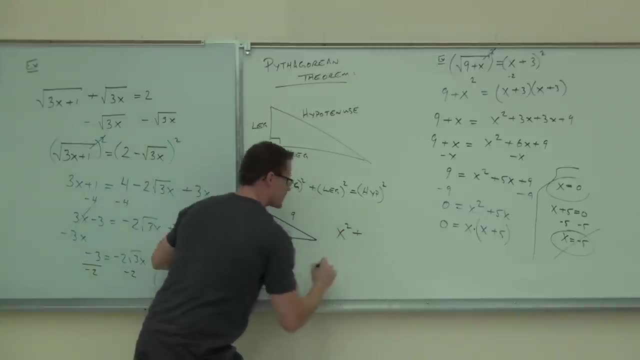 That's a leg squared Plus another leg squared. That would be 6 squared equals 9 squared. So far, so good. How much is 6 squared? How much is 9 squared? Can you isolate the square? How We would get x squared equals. how much is that? 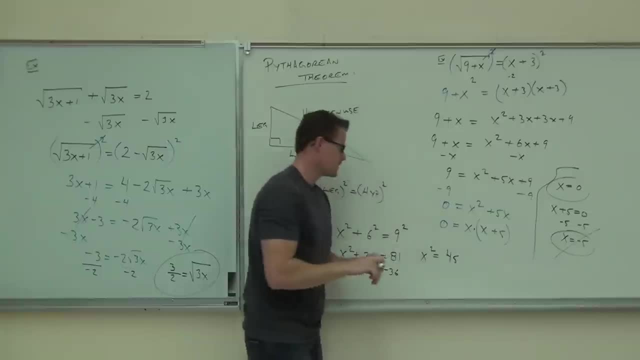 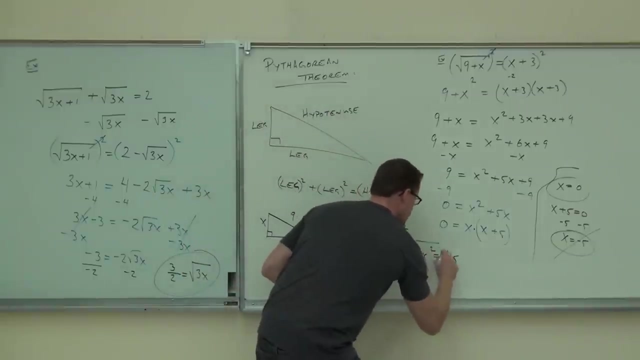 45.. Now here's the question: If you have x squared equals 45, what type of a root will undo a square? Remember, we can take a root of both sides, just like you can take an exponent of both sides. You square root both sides. 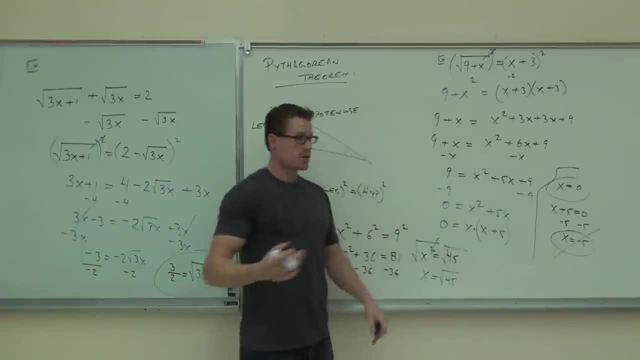 You get: x equals the square root of 45.. If you use a calculator, you're going to get something between 6 and 7.. Or you simplify this and get an exact root. Notice how 9 goes into this. This is 9 times 5.. 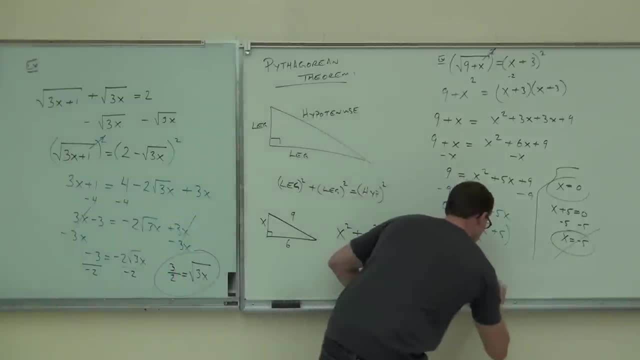 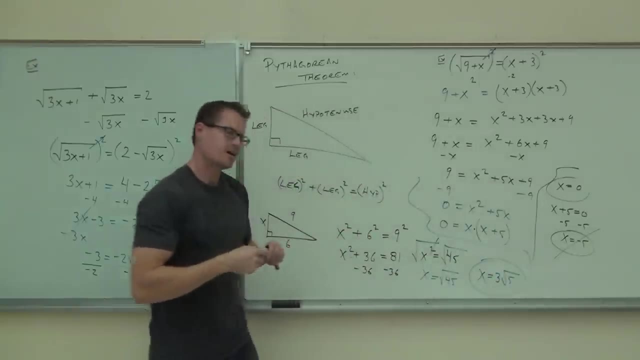 Or you get 3 root 5.. Does it matter which form it is, The book might have both an exact and an approximation, So a calculator would give you an approximation that's exact. One more thing: If you have something like x plus 1, notice how you would have to have this in parentheses. 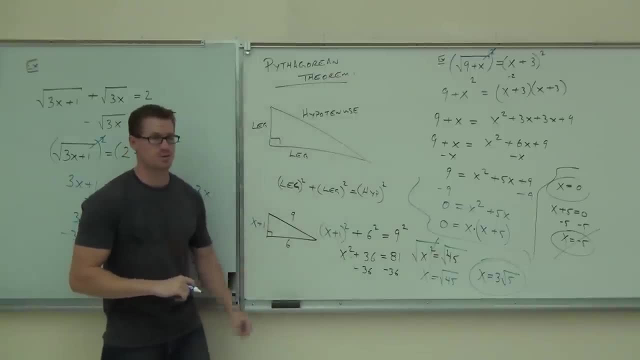 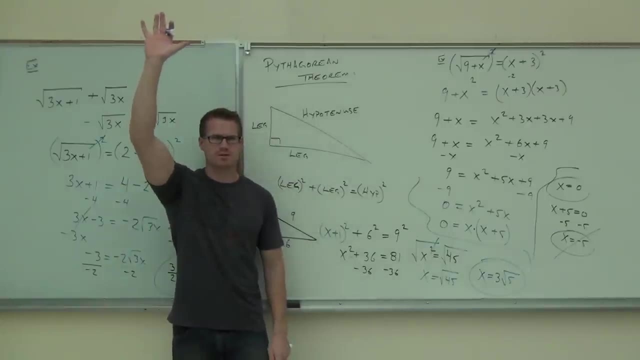 Like that. Do you guys see what I'm talking about? That's something you have to distribute: X squared plus 2x plus 1. Then combine like terms and then you might have to factor that How many of you feel okay with what we've talked about so far, including the Pythagorean theorem? 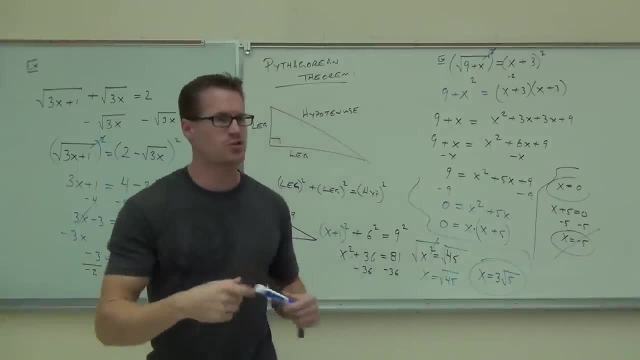 Okay now I went through that quickly. Your book does a very good job of explaining that, But that should wrap things up for you. It's not too hard. It's going to be hard, as long as you're able to set up that equation.